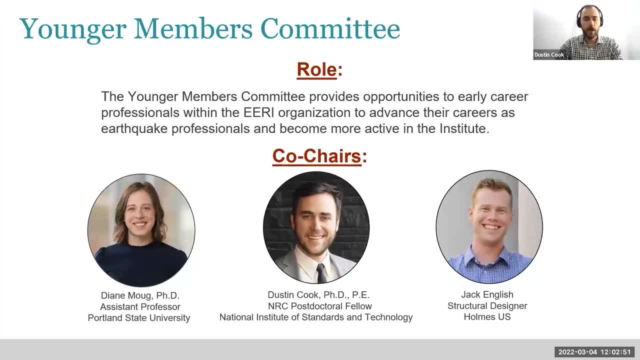 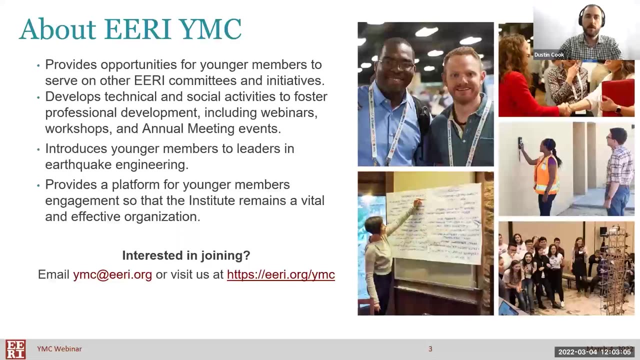 and to be able to kind of engage with the committee at large. The committee is hosted by volunteers. It's hosted by a set of co-chairs- myself, Dr Diane Mugg and Jack English, And so the ERI really so the idea of the YMC is to kind of provide that opportunity for 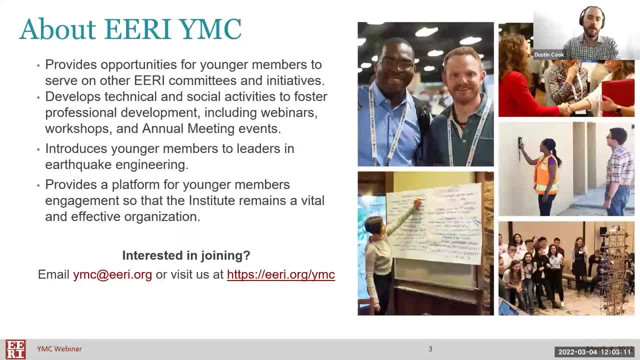 for, you know, basically younger members to become more connected and become a part of the community and serve a larger role with the rest of the ERI committees and initiatives. We also develop technical and social activities to help foster, you know, the professional. 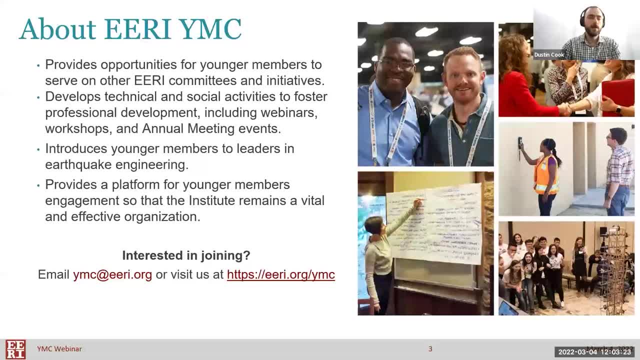 development of younger members. These include webinars and workshops we host throughout the year, as well as annual meeting events. We introduce younger members to leaders in the Earth Lake engineering field and get them connected for further opportunities, And we also provide a platform for younger members to engage with the committee and for the initiative. the organization 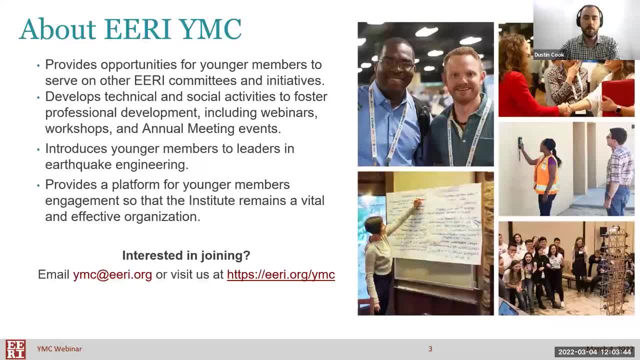 at large to come and participate in the community. So we're really excited to be here today. Thank you so much for joining us today. We're really excited to be here today. We're really excited to be here today to kind of learn from you know, the perspective of younger members. So if you are interested in 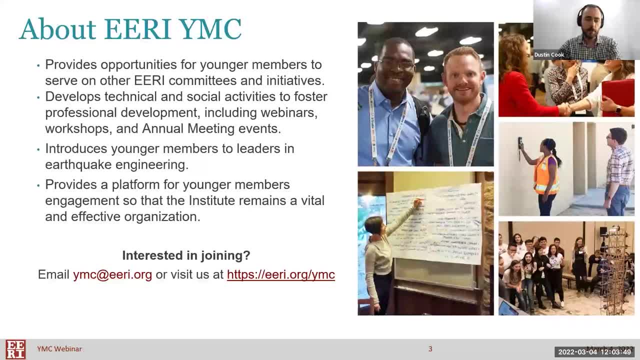 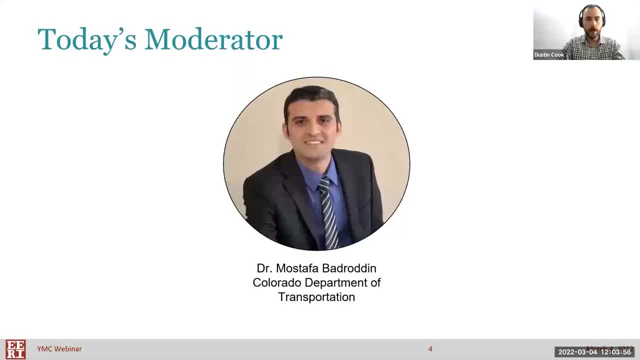 finding more about the YMC or joining. please follow some of these links below at the ERI's website or reach out to us directly. So the webinar today is going to be hosted or moderated by Dr Mustafa Badrutin, So if you, I'll hand it over to you now, Mustafa. 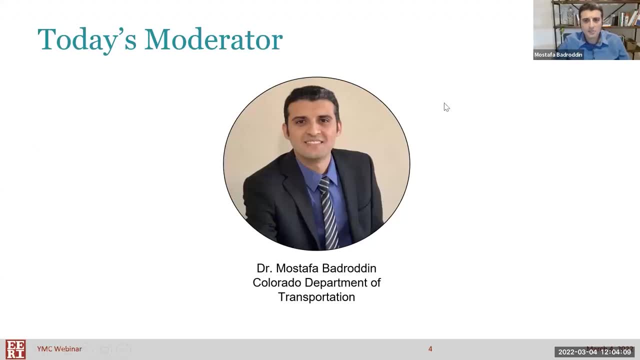 Thank you, Dustin. I'm Mustafa Badrutin, this year YMC webinar coordinator and today moderator. Thank you again for being here this afternoon. Today we will have two presentations on earthquake liquefaction hazard from site to regional scale evaluation. Next. 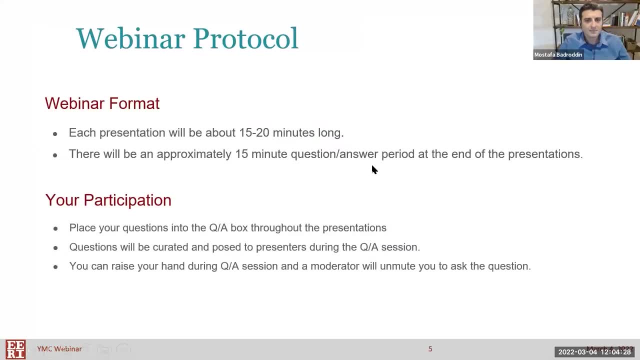 slide. please Dustin. A few quick notes. Each presentation will be about 15 to 20 minutes long. There will be an approximately 20 minutes of question and answer period at the end of the presentation And the webinar will be recorded, and the recording will be posted on the ERI YouTube. 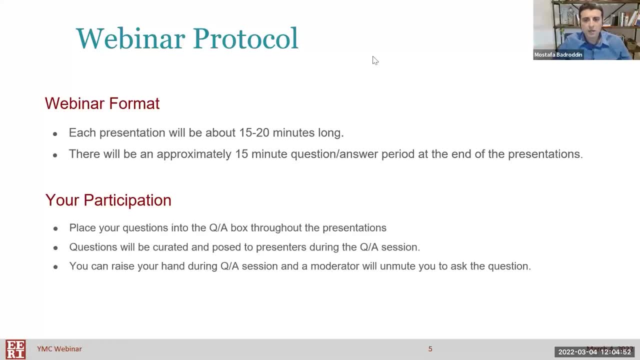 channel and YMC website in a few days. Please feel free to put your question into Q&A box down there throughout the presentations and during the Q&A period. You can also raise your hand during Q&A session and we will unmute you to ask your question. 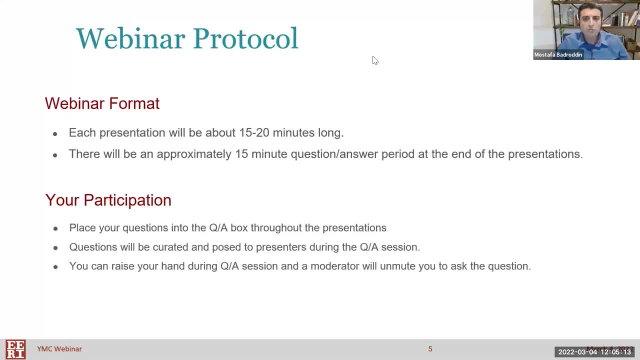 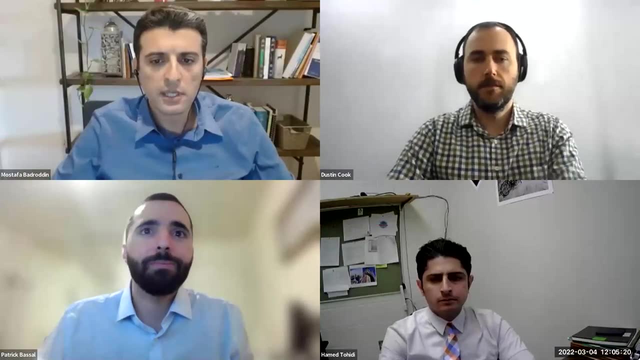 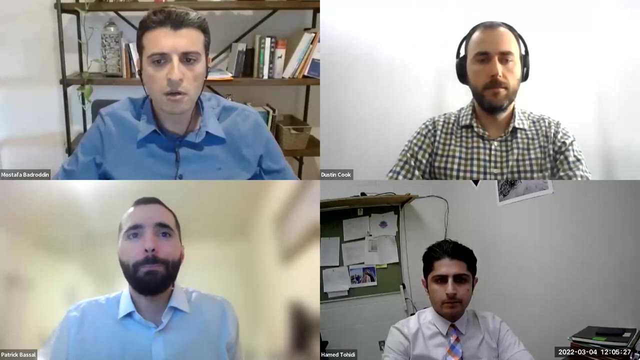 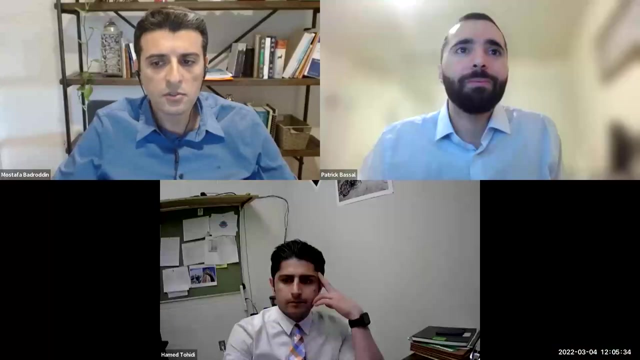 Without further ado, let's get started. Our first speaker is Patrick Basel. Patrick is a PhD candidate in geotechnical engineering at the University of California Davis. He's currently completing his research regarding the computational evaluation of earthquake-induced ground deformations for sites with interlayered soil deposits. Over to you, Patrick. 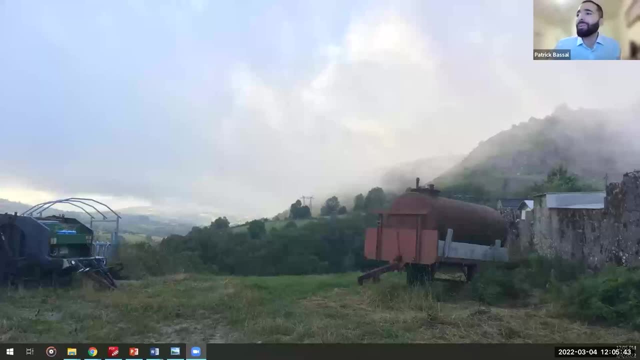 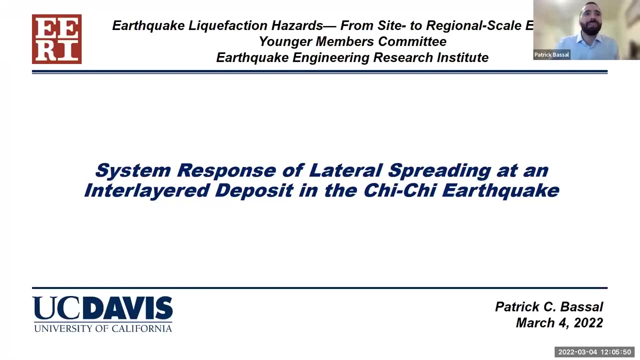 Thank you, Mustafa, for the introduction. I'll go ahead and share my screen, Okay. So since we're going to be discussing liquefaction from different perspectives today, my presentation is going to be more focused on starting things off looking at site-specific evaluations, And so I'm particularly looking at one site. 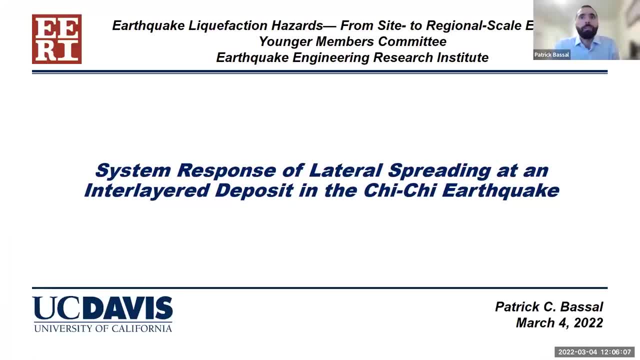 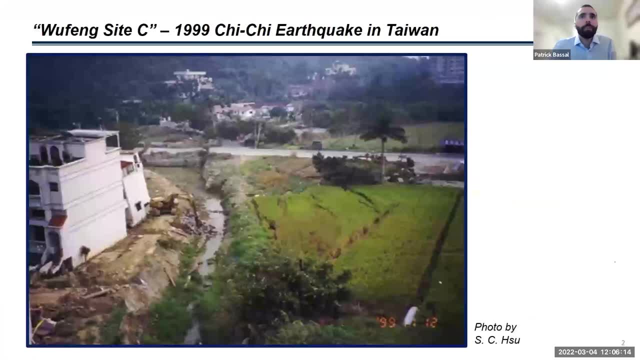 for this presentation, And so my talk is on the system response of lateral spreading at an interlayer deposit in the Chichi earthquake, And so I'm specifically going to be discussing Wufang Site C, And this is a site that was affected by the 1999 Chichi earthquake in Taiwan. 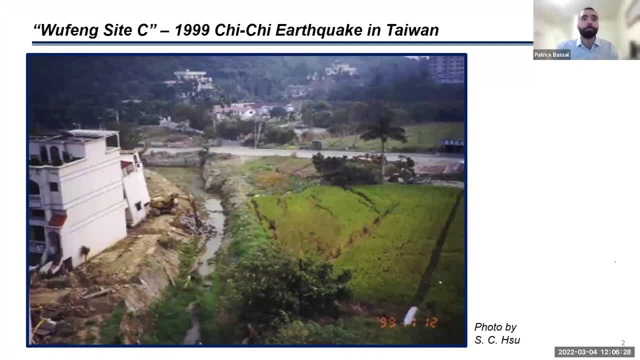 And so the site is a rice field adjacent to a meandering stream channel, And during the Chichi earthquake, the site experienced 50 to 200 centimeters of lateral spreading deformations, all concentrated within about 25 meters from the adjacent stream channel. 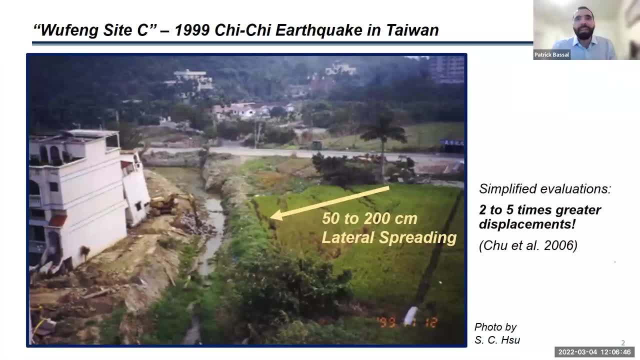 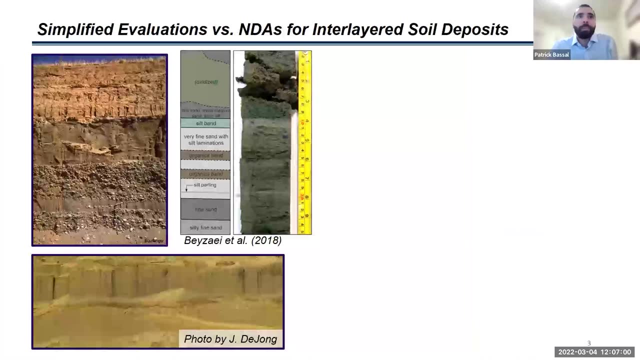 However, past studies were done following this event and they used common simplified methods and found that two to five times greater displacements should have occurred based on those existing simplified methods that are still used today. And so, if we take a look at the subsurface at Wufang Site C, beneath the surface we 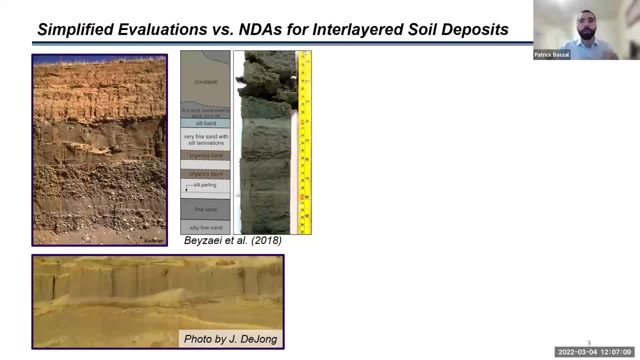 have interlaced. There's soil deposits with alternating and discontinuous layers of sand, silt and clays, And so the past studies that were performed at this site were performed using empirical and semi-empirical lateral spreading analysis, And these are simplified evaluations that are fast and common to perform still very 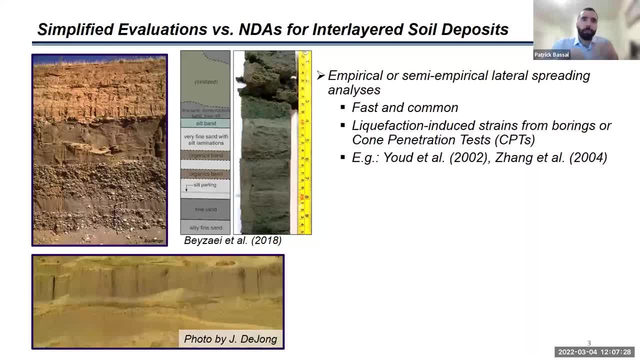 common in practice And they rely primarily on estimates of liquefaction-induced strains from correlations with our borings and cone penetration tests. This is a series of graphs showing a direct match between the Zang et al 2002 study and the Zang et al. 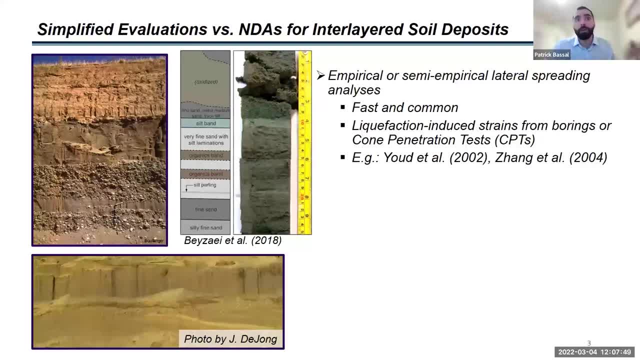 2004 method. However, as was the case at Wufang Site C, these methods do tend to overpredict deformations at interlayered soil deposits. This has been seen through countless past earthquakes, not just in the Chichi earthquake. 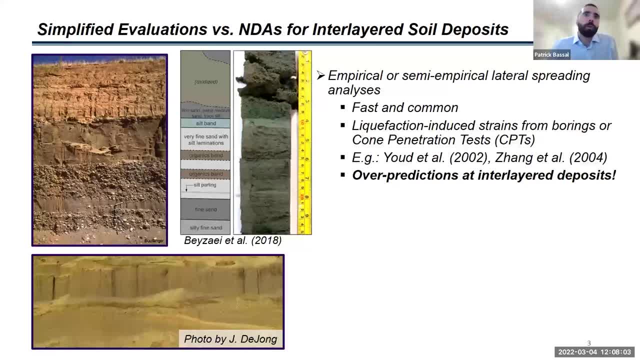 but others as well, And so when we're looking at more high-risk projects, we do see some Ensha19 and the other studies on this same topic. So, as the data shows, we see a lot of overprediction of deformation at interlayered soil deposits. 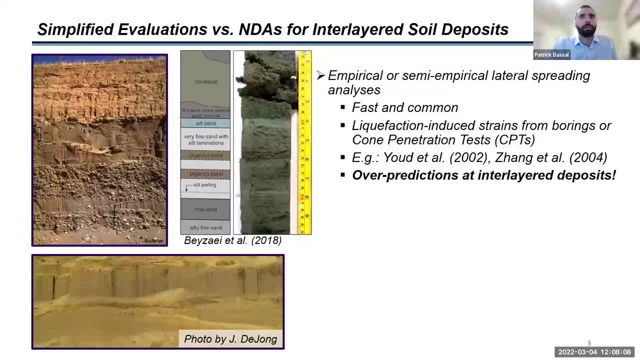 So let me just point out here the four different methods here. The first one is the Zang et al 2004 method, And that was the case at Wufang Site C projects. we can sometimes, as said, use a more detailed evaluation, which. 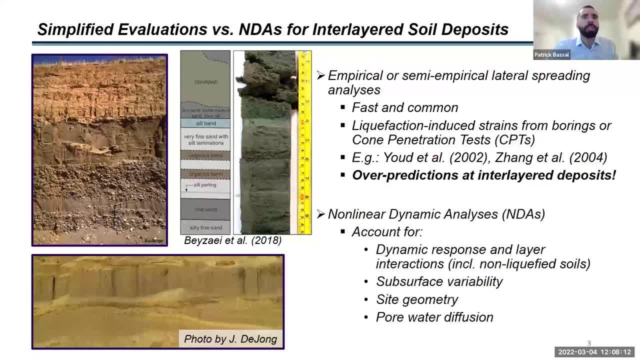 might be commonly done in practice for these bigger, high-risk projects, And these can often be termed as nonlinear dynamic analyses or NDAs, And so these methods can account for the dynamic response and layer interactions not only for liquefied soils, but also for non-liquefied soils that you might have. 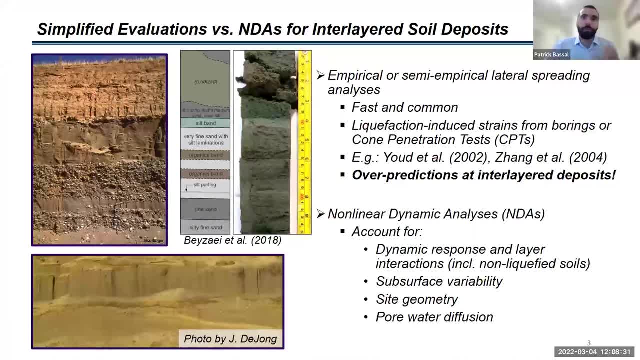 within an interlayer deposit. They can also account for subsurface variability, your site geometry, and pore. water diffusion, which might occur after liquefaction, occurs within a sand lance, for example. So one important question is: how much can these methods really improve our predictions? 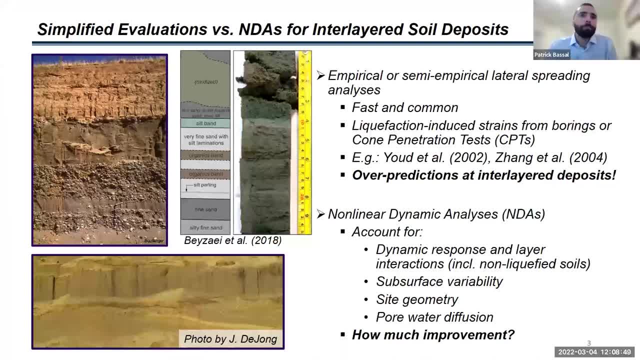 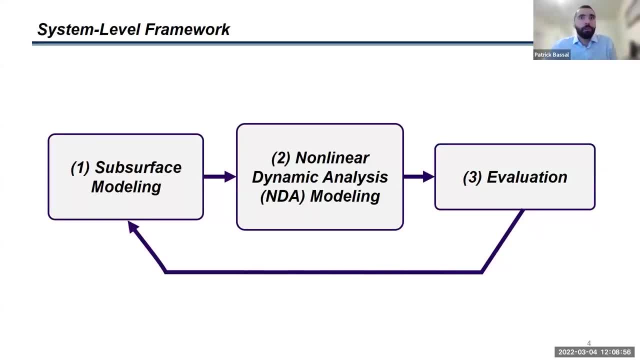 And so that's a big focus of my work, And so, in order to best evaluate the deformations that occurred at WuFang Site C, I followed a system-level framework that first considered subsurface modeling and then our nonlinear dynamic analysis modeling, or NDAs. 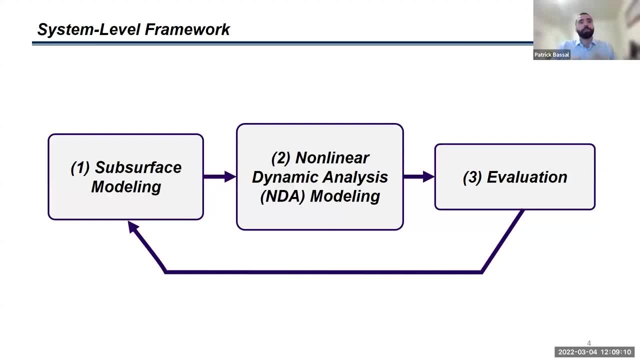 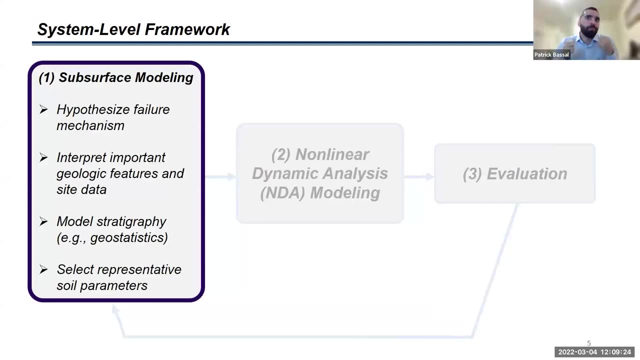 as well as an evaluation that's open to reinterpretation based on the uncertainties that we have at our site, And so the remainder of my talk is going to dig into details and lessons from using this overall system-level framework, And so the first step of this system-level framework- 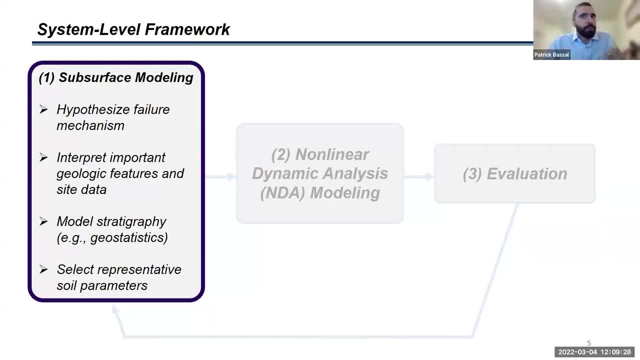 is subsurface modeling, And the approach that's taken here really depends on both the failure mechanism and the conditions at your site, And so it's important that you first hypothesize the expected failure mechanism that you would expect, And after you have at least an idea of what you're looking for. 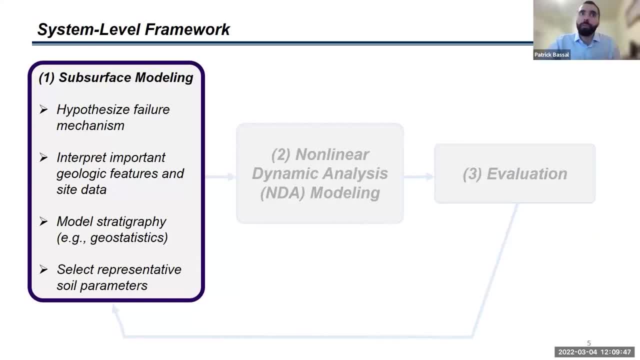 then you want to spend some time interpreting any important geologic features as well as your site data. You then want to model your stratigraphy, And this could entail using some geostatistics, which I'm going to dig into a little bit during my talk. 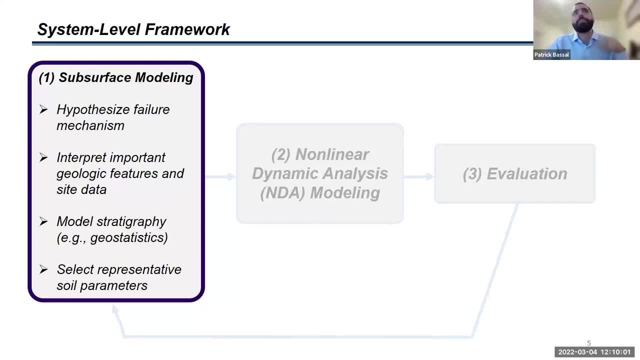 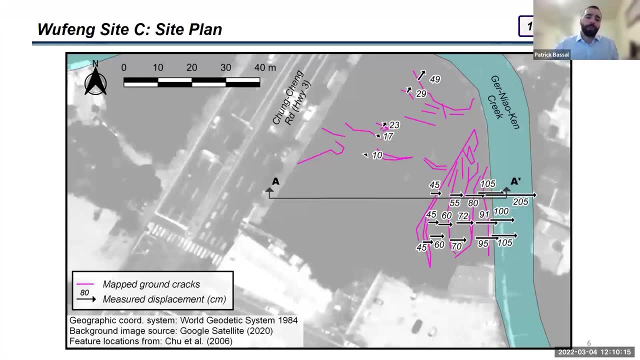 depending on how much detail you want to get into. And finally, you want to select representative soil, soil parameters to model your site. And so now, starting off with the subsurface modeling portion of our analysis, this map shows the locations of cracks. 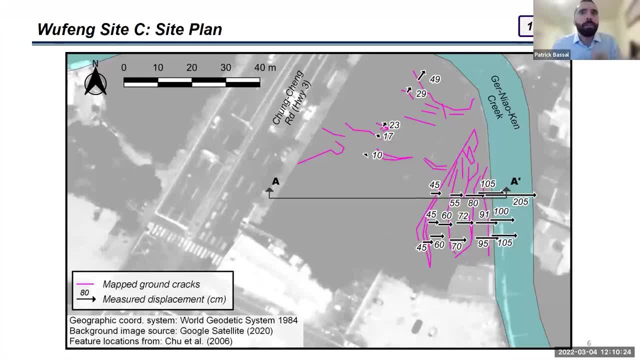 and purple aquifaying site C And you can also see the displacement vectors And if you pay attention to the east-turning displacements, they go from about 45 centimeters to 100 to 200 centimeters when you're near the channel. 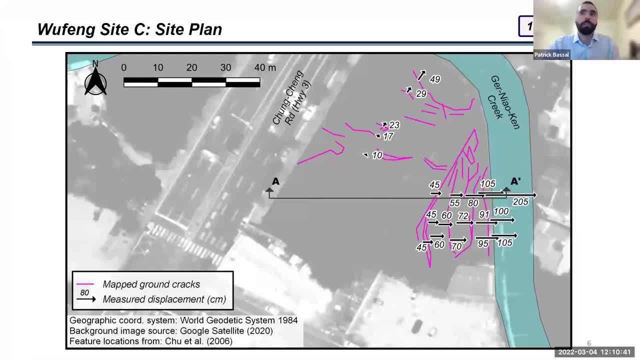 And they're concentrated within 25 meters of the channel, like you can see, And so we had site data. A site investigation was performed following the Chiché earthquake, And so these are the locations of our CBTs, our co-inventoration. 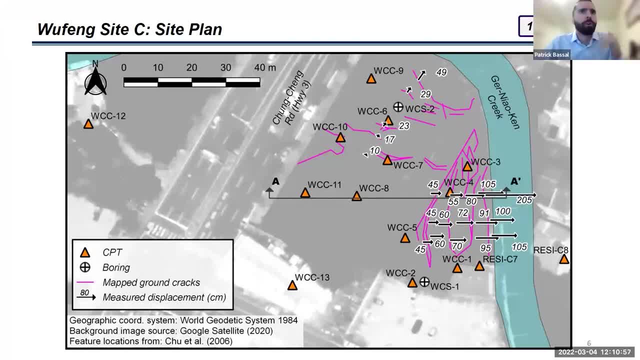 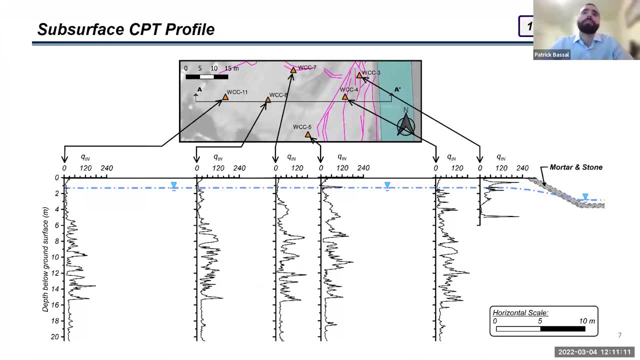 tests and our borings. We had about two borings, and the orange triangles are our CBT locations, And so now, having that map in mind, we can next look at a subsurface profile section taken along the eastward deformation, And so each of the plots shown here. 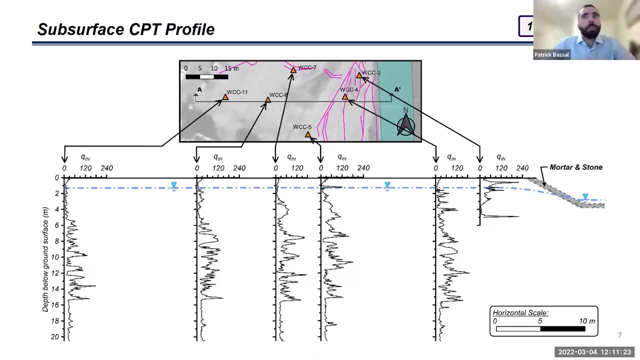 are for the CBT co-interprets, since, potted with depth, And in order to better interpret the subsurface, I categorized the data based on a soil behavior type index, And so this is just a little bit of a summary. This is just taken from the CBT readings. 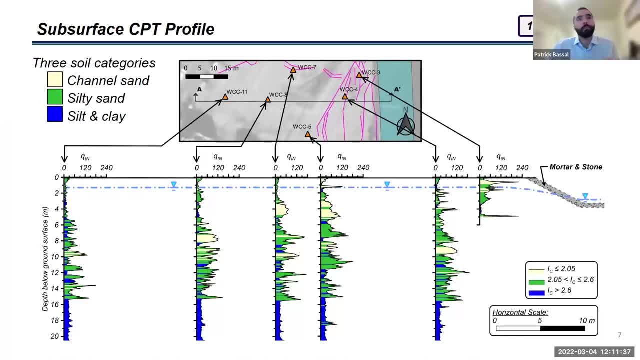 using a correlation that breaks up the data into some different potential soil units. So I broke it up into channel sands, silty sand and silt and clay materials, So this gives us a sense of what's happening as far as the different soil faces. 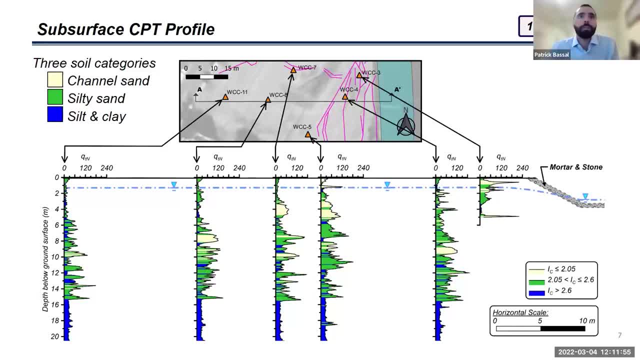 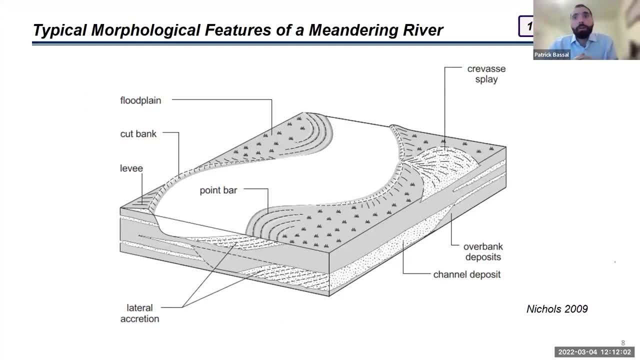 that we have And in order to better understand what's going on in the subsurface, we can further constrain and model the subsurface And by drawing on some general insights that we might have about the geologic environment. And so we think site C it's located at the inner point. 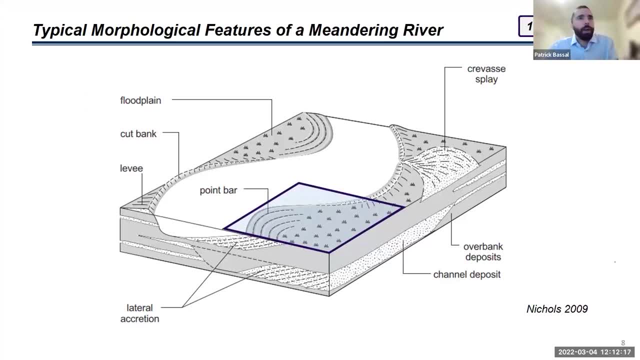 bar of the Mandarin Stream Channel, And so we can expect to have, within this area, based on the geologic environment, we can expect to have overbank deposits, as well as channel deposits and lateral accretion surfaces that occur due to the movement of the river channel over geologic 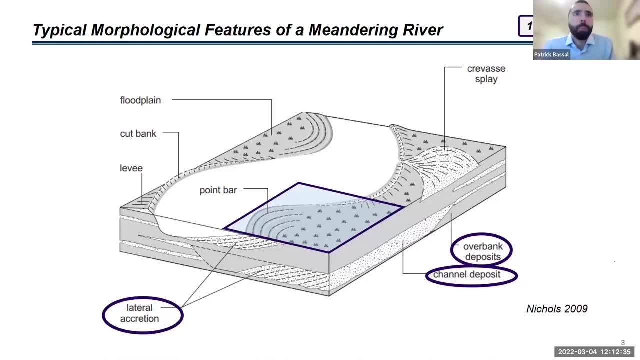 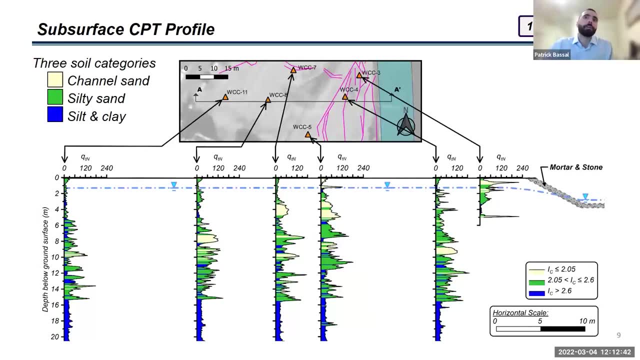 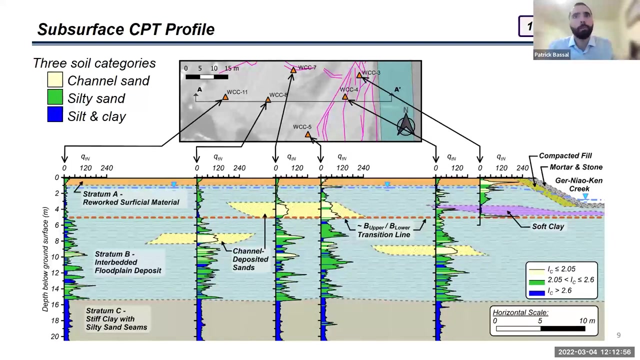 time, And so we can then use geologic inference and our CBT data to better refine our subsurface interpretation and really get an idea of, OK, what's going on. And so we drew up a profile based on what we know, And we did want to pay attention to certain features. 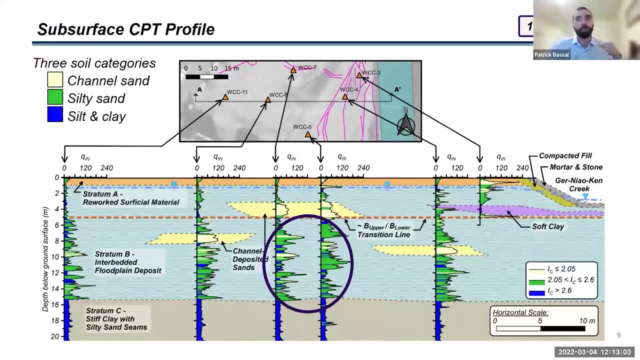 And we had discontinuous channel sands as well as interbedded overbank deposits. We also considered a soft clay seam near the channel And we had finer material further from the channel And that tends to make sense based on what we know about the geologic deposition. 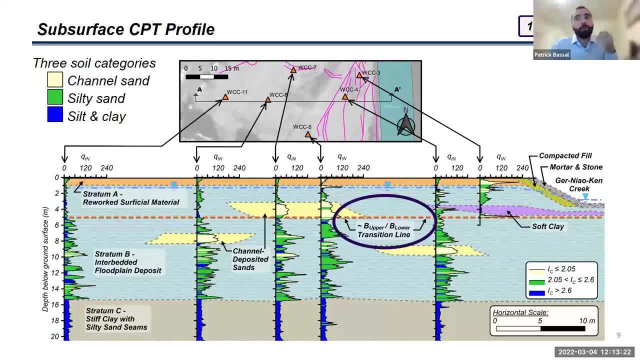 We might expect that. We also noticed lower soil strengths above a 5-meter depth, And this was present in all the CBTs. So we're not sure why that is, But of course it does make sense that. So we're not sure why that is, But of course it does make sense that. 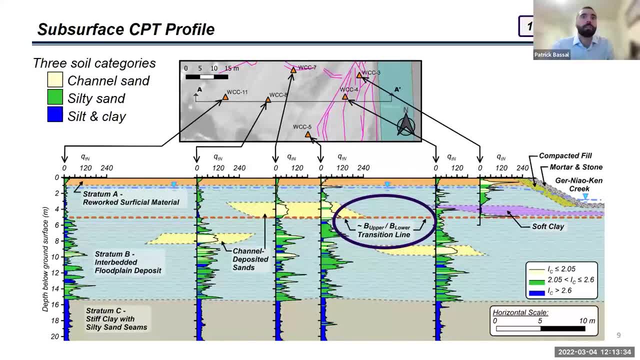 But of course it does make sense that. But of course it does make sense that You have less consolidated material near the surface, And so we do have weaker material above that depth. And so, since our goal is to evaluate the magnitude and extent of lateral spreading, 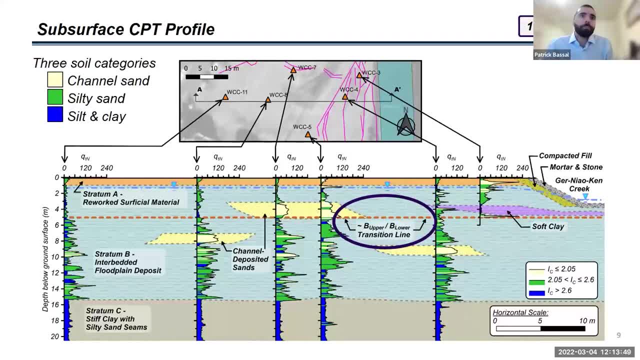 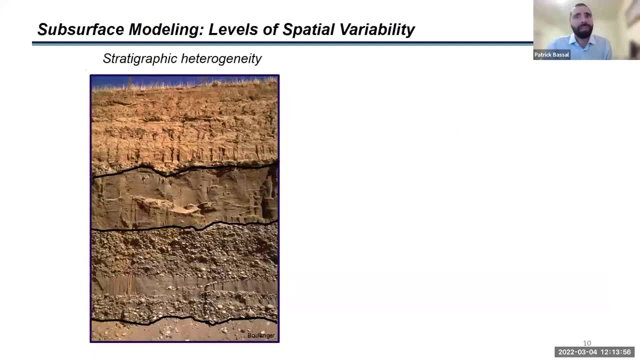 we did want to consider the influence of all of these details, And so now digging a little bit deeper into our subsurface modeling. depending on the mechanism you're trying to evaluate, the subsurface can be modeled to account for different levels of spatial variability. 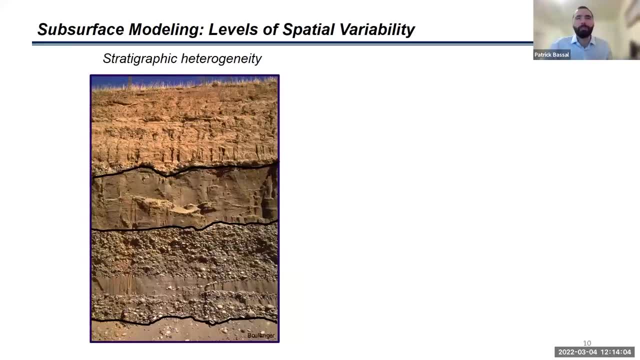 And so stratigraphically, we've done that And we've done that, And we've done that, And we've done that, heterogeneity is shown here, And this is really just looking at the major geologic depositional changes. So it's really just looking at layer thicknesses. 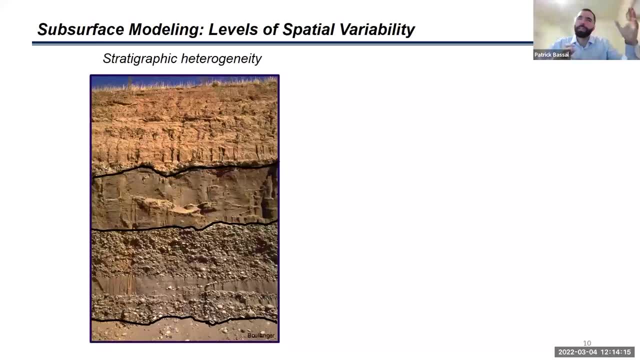 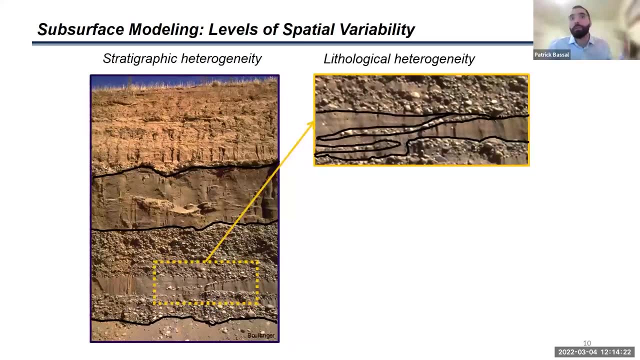 on the order of meters, And so we're not really getting into any details here. We're just really looking at the geologic deposition. If you dig deeper, look at the lithological variability within each stratigraphic unit, such as the interlayering. 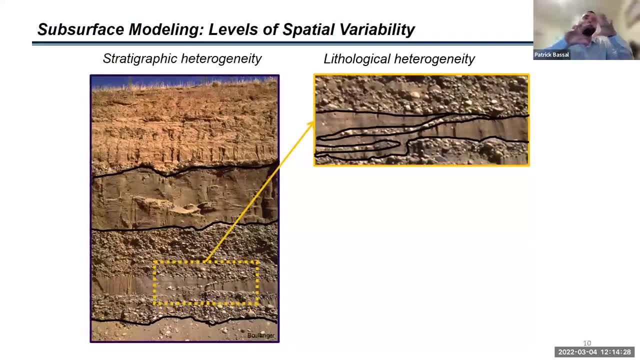 shown here, And in this way we can model different soil facies, different soil types within each unit. And we can also dig even deeper and look at the inherent soil variability that's due to parametric changes of a given soil type. whether we're looking at differences, 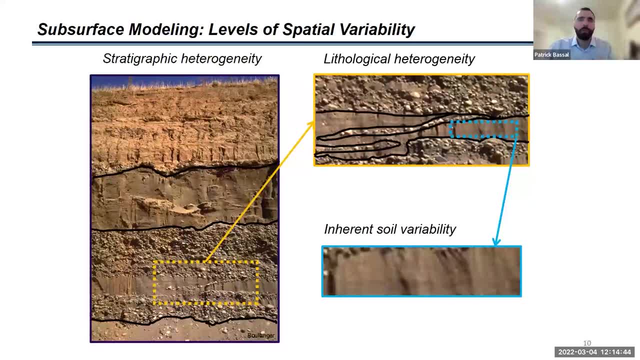 in the permeability or in your soil strength, your density, So we can also dig deeper and model that. And so, at Wu-Fang Site C, it was of greatest interest to capture the interlayering of the different soil facies within that floodplain deposit. 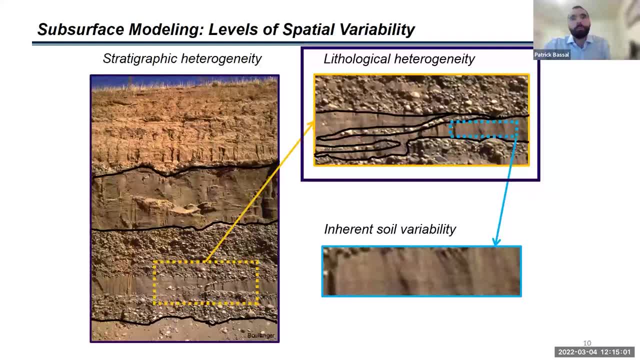 And so the scale at which that interlayering was expected to affect large lateral spread features was important. So really we're interested in this level of detail. We didn't think it was important to dig deeper into the inherent soil variability based on the properties we had at the site. 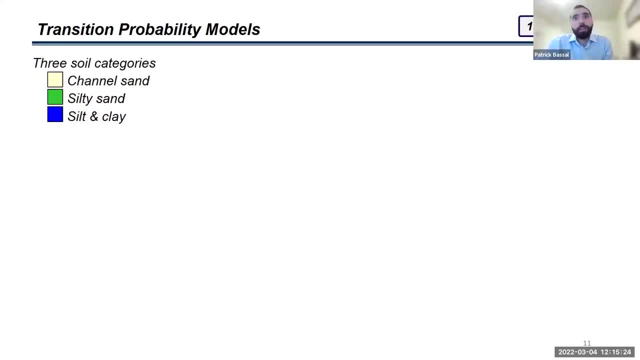 And so, in order to account for the interlayering, to account for this lithological heterogeneity between our different soil groups, We modeled the subsurface using transition probability statistics And so, just as an example, let's say we can interpret the interbedding from this one CPT. 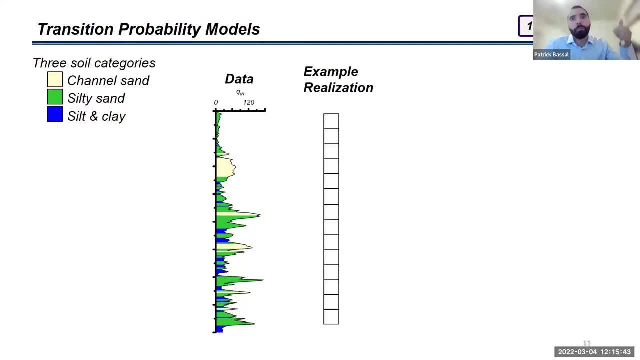 And we want to then build a realization along this column. Let's then say we're given a silty sand at this location And we want to predict the soil type adjacent to it, just a short distance away, right next to it, And so, based on the data we have from that one, CPT. 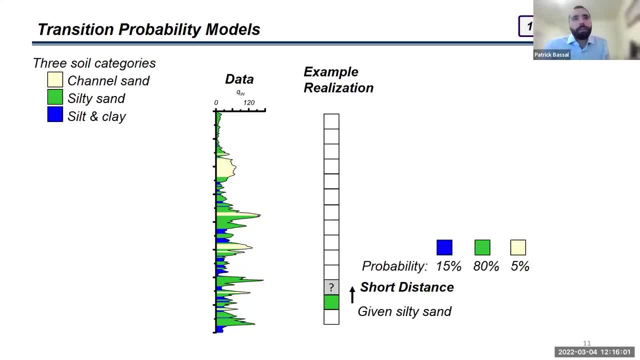 we might have these probabilities of having a different material or the same material, And so notice that there is an 80% chance of remaining within your silty sand material because you're moving just a short distance away. Essentially, we want to move a longer distance away. 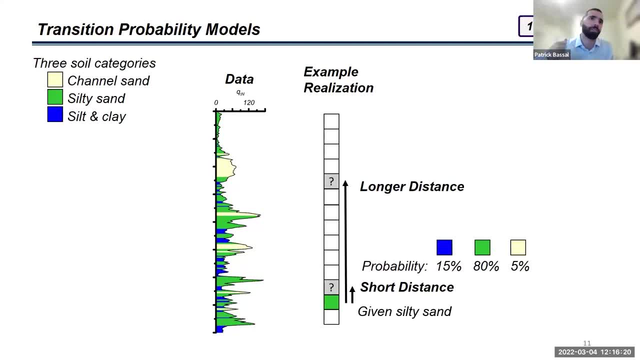 and try to predict what soil type we have based on only knowing that, given silty sand, Our probability of transitioning might now be very different. We might have only a 50% chance of getting the same material, And this is actually closer to the overall proportions. 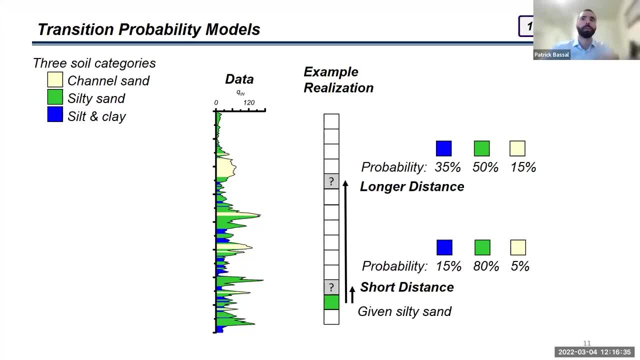 that we might have within the CPT now that we're moving further away, And so, by taking different random paths to simulate this column, we can then generate a realization that might look like this: We can build several of these based on just accounting for the probabilities with distance. 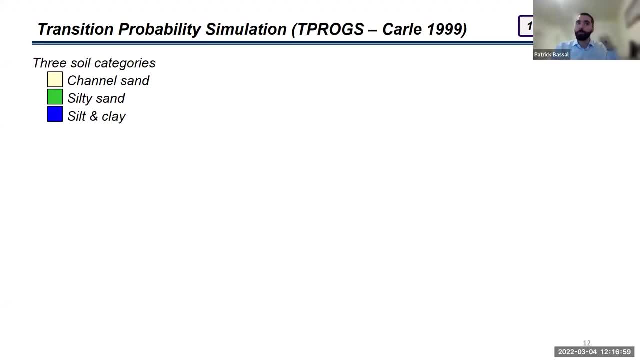 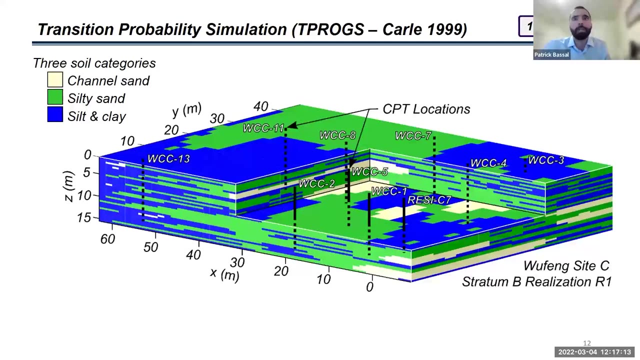 And so, using all the available data that I had at the site, I modeled the transition probability behavior in three different directions, And so it did require some assumptions as well as really considering the data we had, And so that ultimately led to producing this geosynthetical realization of our site. 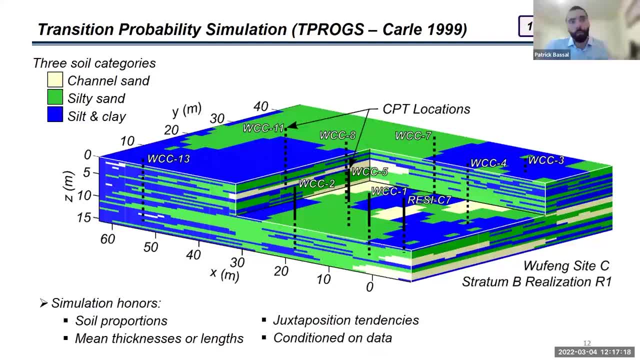 And so the simulation approach that I use honors our soil proportions, our mean thicknesses or lengths, our juxtaposition tendencies, which is just the relative ordering between going from a silty clay to a silty sand, For example, or from a silty clay to a channel sand. 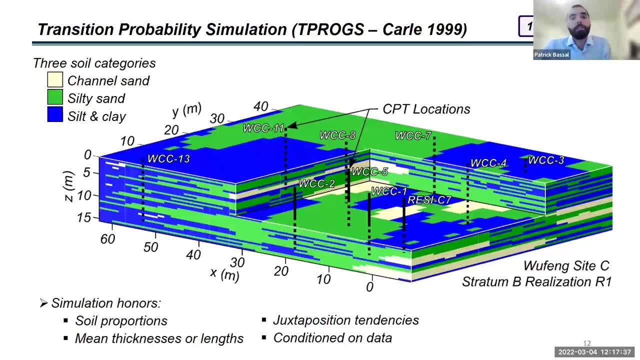 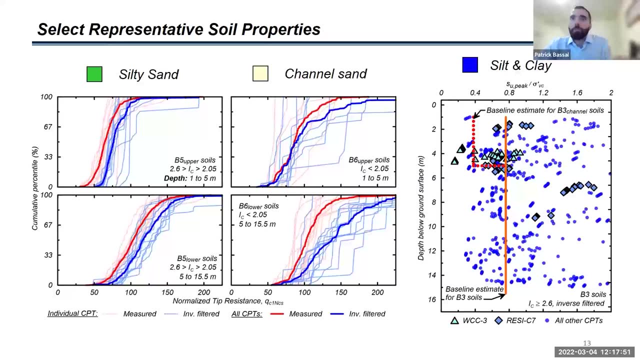 It's also conditioned on the CPT data, And so, using this model, representative soil units can then be assigned to each layer based on the data we had across the site. So I'm not going to go into too many details here, but I looked at the variability of properties. 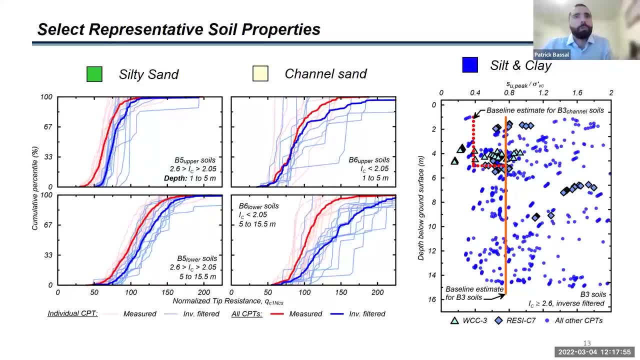 within each different soil category. And so for the silty sand and channel sands, the pots, the soil, And so we did look at that as well, And the plot on the right shows the underlying distribution of the CPT data, and we 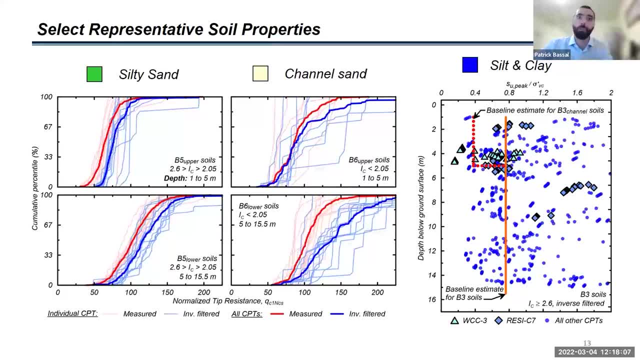 also looked at the cumulative distributions of the individual CPTs and the combined CPT data. We're looking at the normalized counter-resistance here, And so this gives us a chance to really consider any important lateral trends between our CPTs. The red and blue lines just represent different ways. 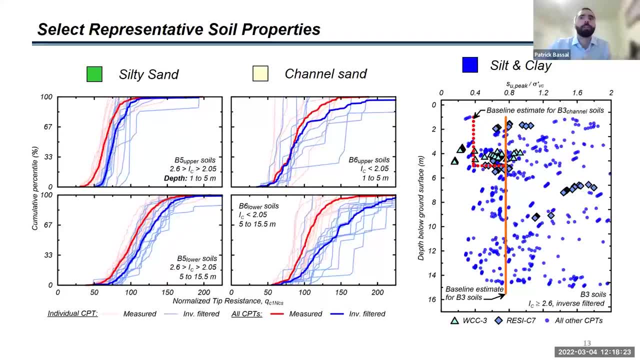 of looking at the data, either taking the measured data from the CPTs or applying a thin-layered correction, And so we did look at that as well. This is the underlying strength of the silting clay material and reporting it with depth. 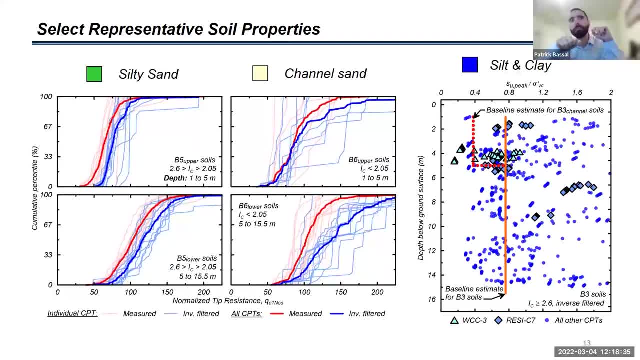 And so we tried to highlight in this plot some of the data from individual CPTs to see how they stood out from the remainder of the site. So now we will look for any differences that we wanted to model across our site. All right, so that was our subsurface modeling. 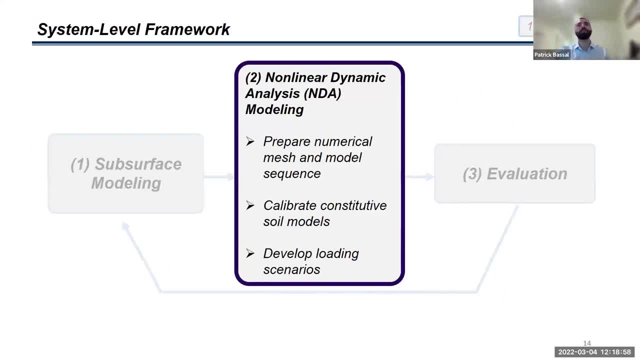 The next step in the system level framework that I'm going to briefly go through is the nonlinear dynamic analysis modeling, And so this step first involves preparing a numerical mesh and a modeling sequence and calibrating our constituent of solar models and developing loading scenarios. 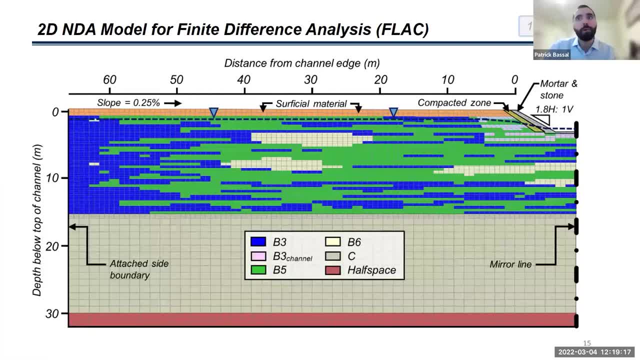 So sizes of the 3D subsurface models were used for our 3D analysis, And we used the flag-finding difference program for our modeling effort, And so this is an image of the mesh for one realization that was used in our modeling. 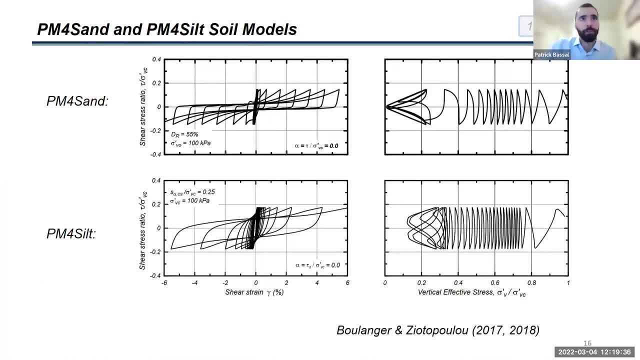 And so I used the PM4Sand and PM4Silt constituent models for the majority of the layers in my analysis, And so these are example single element simulations showing the cyclic sharing response of a PM4Sand and a PM4Silt element. 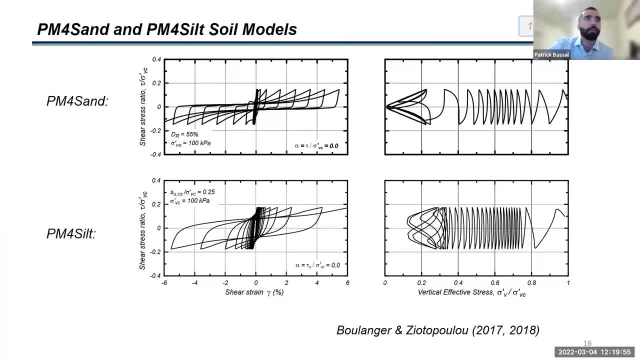 And you can see that this does closely model the key behavior of sand-like or silt-like soils. So you can see that the silt-like soils are showing the stress strain response And the plots on the left are showing our stress strain response and the plots on the right 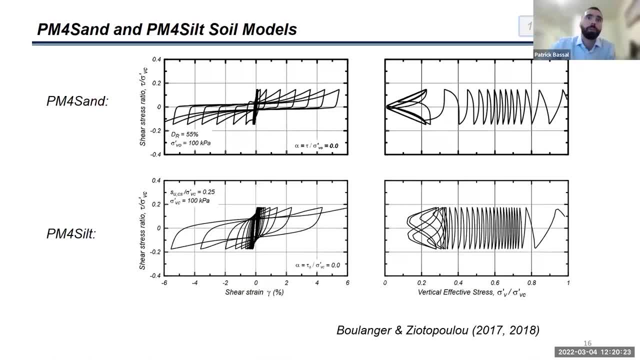 are showing our stress path And that does model what you might see from lab testing fairly closely. Of course you have to do some calibrations And that's commonly what's available in practice. You might not always have access to advanced laboratory testing. 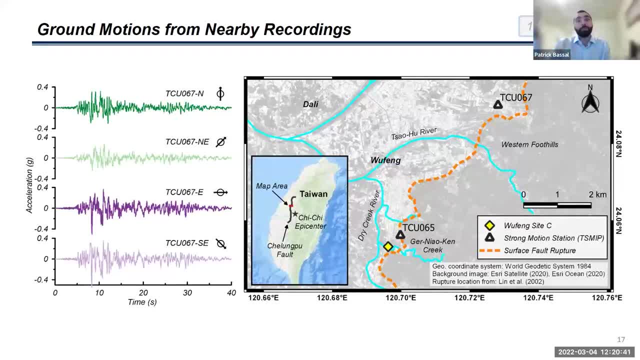 And so ground motions were then selected by considering and deconvolving nearby recording stations that were a similar distance from the fault rupture as the site was from the fault rupture, And so for this analysis, I was interested in really looking into what alternate orientations might give you. 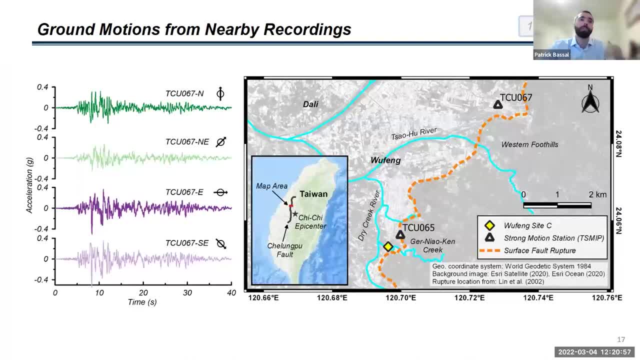 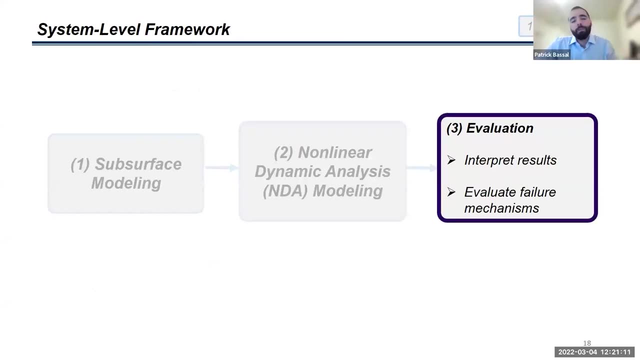 to get a sense of their influence on the lateral spreading of deformation, Because when you're looking at lateral spreading you really do want to consider the orientation in your motion. that could have a big, big effect on your response. And so that was me just looking at the MDA modelling. 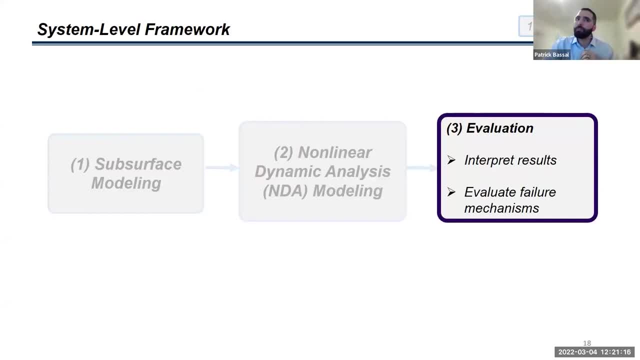 Just briefly looking at some of the assumptions we made. There are a lot more details on that. However, the final step in this system of framework is to interpret the results and then evaluate more failure mechanisms. So we're looking at different cables. So those are the kinds of contacts we use for these events. 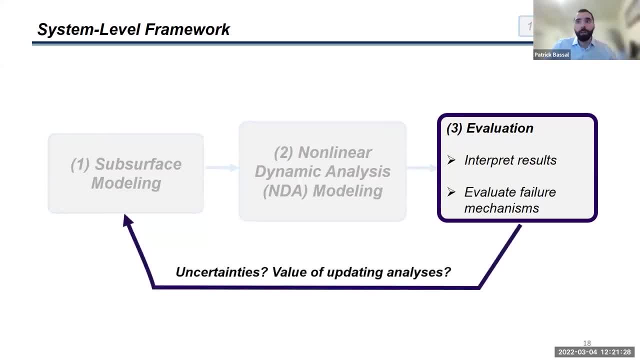 And this is ultimately a process for a type- бар Spring rules that follow come up next, But the bottomğırd élect attract AB mark. It depends on whether we agree with our original hypothesized mechanism and whether we should update our analysis considerations and maybe rerun some of our analyses to reconsider some. 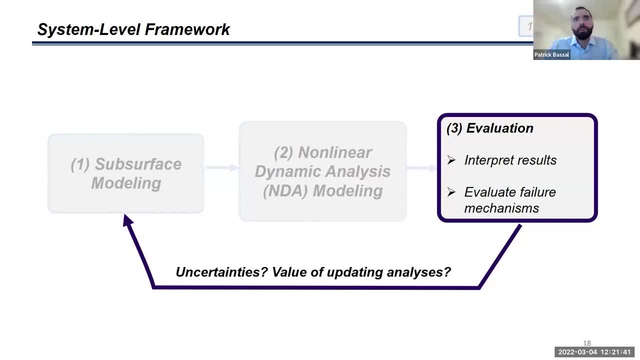 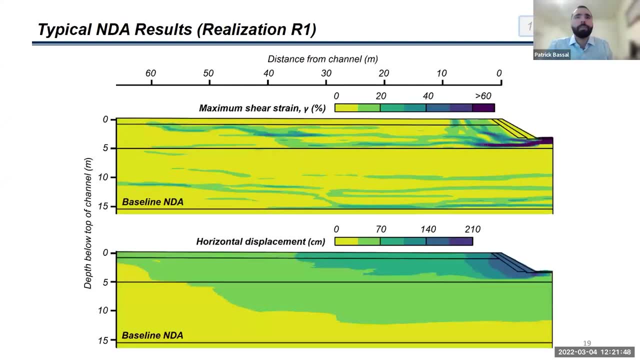 of the assumptions that we originally made based on the uncertainties that we have. These are example results for one analysis case using one of our subsurface realizations, And so the top plot is showing our maximum shear strains and the bottom plot is showing our horizontal displacements as contours. 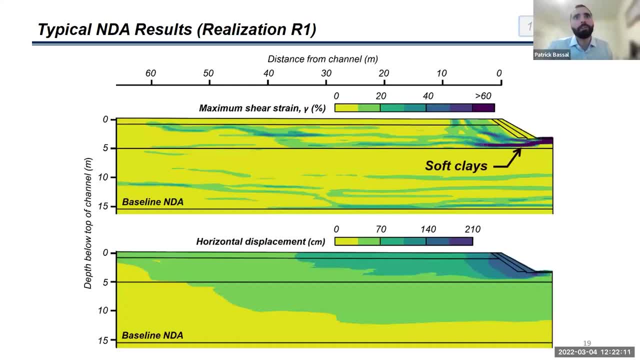 And so you can notice here that high strains of greater than 40% occurred in the near channel soft clay material, And this ultimately caused a rotational slump with large deformations near the channel. Also, high strains also developed in the silty sand due to liquefaction of those materials. 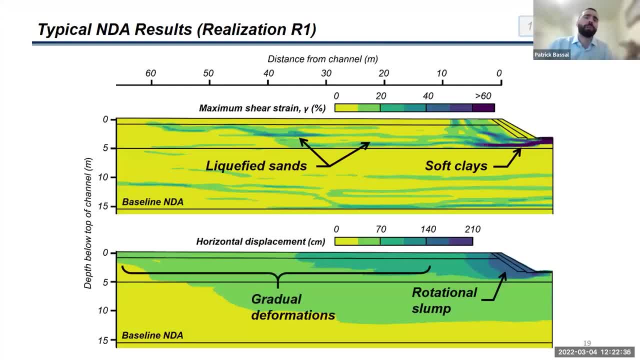 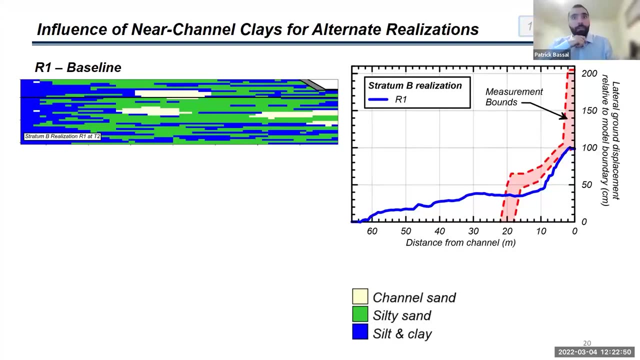 And this also ended up causing some more gradual deformations away from the channel, but they weren't nearly as extreme as the deformations from that rotational slump. So we then looked at the ground displacement with distance from the channel And we also looked at the channel for different realizations of our full-plane deposit. 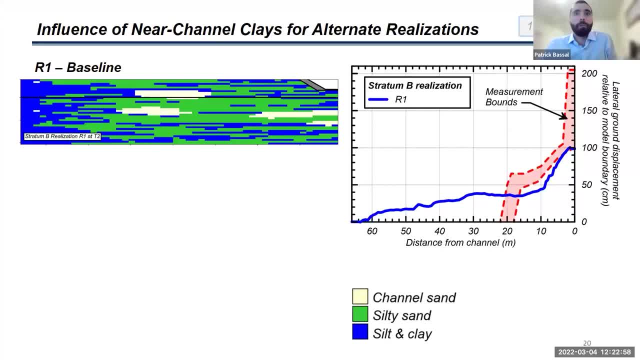 And so the red area on this graph here we're showing the measurement bounds for the ground cracks, the ones that were measured in the field, based on the crack widths, And the blue line here is showing results for one realization, the realization R1, that 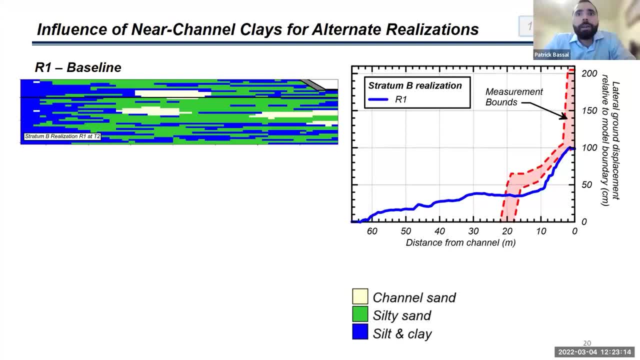 you can see here And you'll notice that the near channel displacement is approximately captured in our model. We are approximately capturing what happened in the field, but displacements away from the channel are slightly over-predicted And so, if you look at a different realization now, we have more clay near the channel. 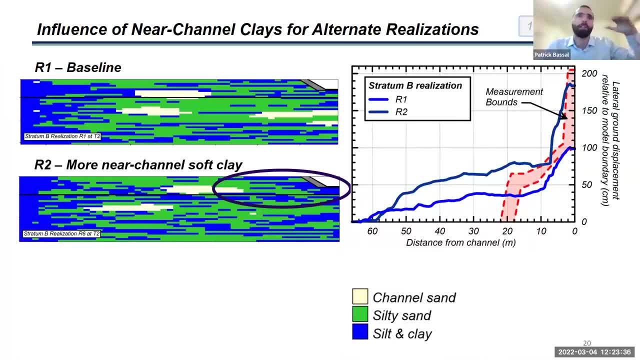 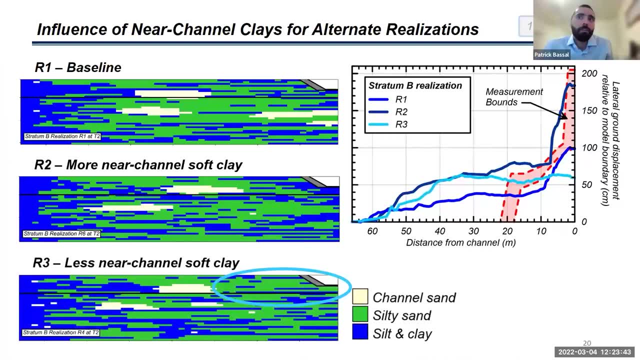 The near channel displacement is now also much higher and we're nearly bounding the observed response in this realization. And if we then look at a realization with a lot less of that clay material near the channel, we get much lower near channel displacements. 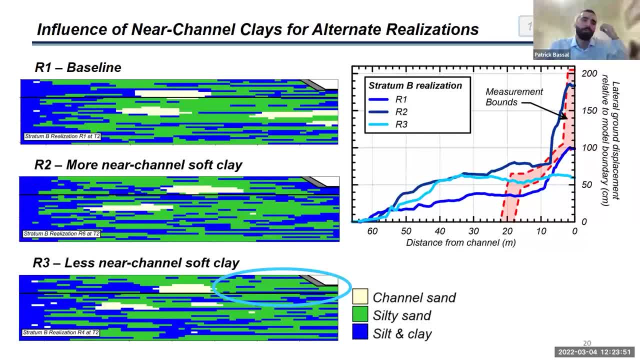 And this all makes sense. It's pretty clear that that's what caused the rotational slump. So now we're really just removing the influence of the clay on creating that near channel rotational slump, And so our data for this clay isn't well constrained. 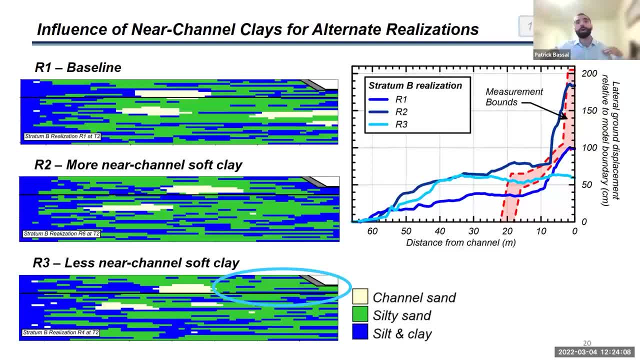 And so these realizations really give us a chance to understand the impact of that uncertainty of not having enough data to constrain how much material we have. And so we also looked at several other realizations, And they're shown in red, They're shown in gray here. 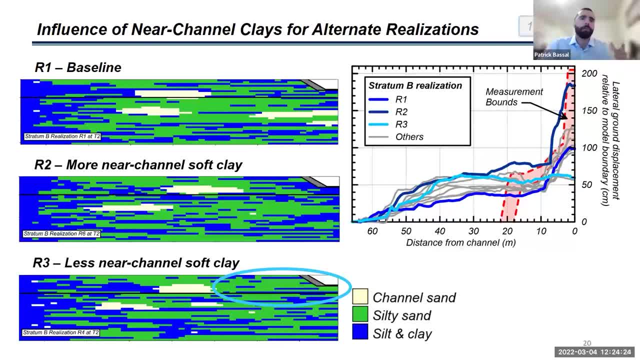 And you can see that they all tend to be fairly bounded within some of the other responses that we have. They all fall within a pretty close range. So the variability we get here it's not too great, except for what you're getting near the channel. 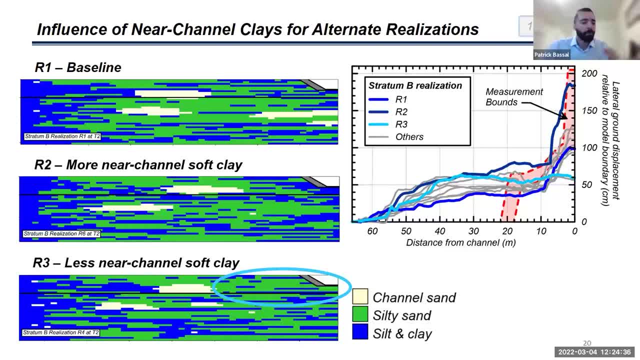 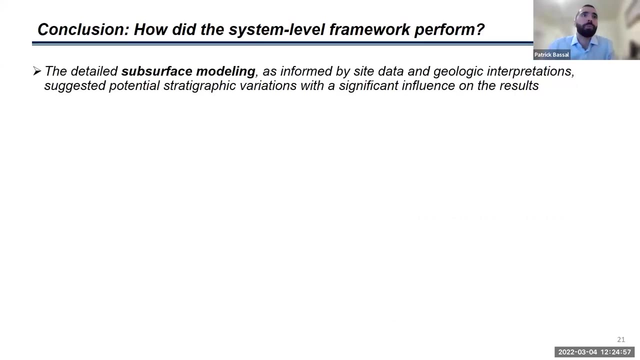 And for this study we did look at several other parameter assumptions and different ground motions, But one of the focuses here of this presentation is just to really get a sense of what's happening due to that stratigraphic variability. And so, in conclusion, how did the system-level framework ultimately perform? 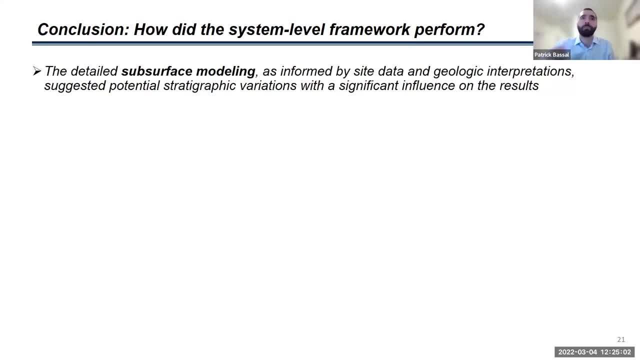 So the detailed subsurface modeling, as informed by our side data and our geologic interpretations, did suggest potential stratigraphic variations that did have a significant influence on the results, especially in the near channel area. The 2D NDAs captured aerodynamic layer interactions overlooked by simplified evaluation. So when we look at the data here, we're seeing some potential stratigraphic variations that did have a significant influence on the results, especially in the near channel area. The 2D NDAs captured aerodynamic layer interactions overlooked by simplified evaluation. 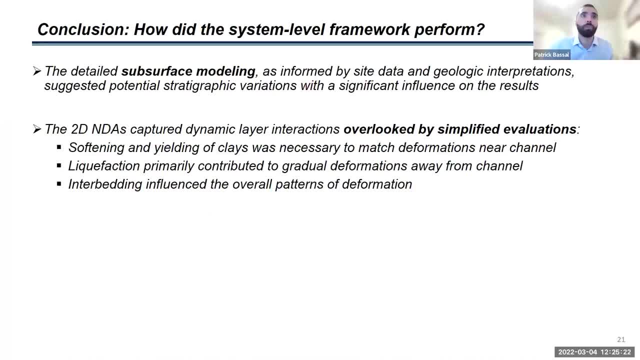 evaluations. So it did capture the softening and yielding of clays which was necessary to match the deformations near the channel, And so these weren't considered in those simplified evaluations because they really just considered on liquefaction. So it is important to consider. 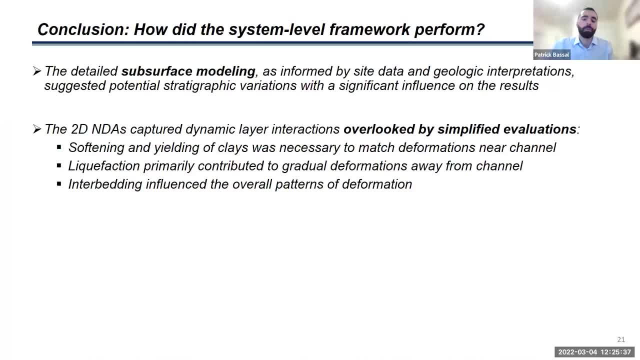 okay, like what other effects do we have? And in this case, the rotational slump did extend beyond what's typical, And so that did ultimately influence those overall deformations. The liquefaction did occur, but it primarily contributed to gradual deformations away from. 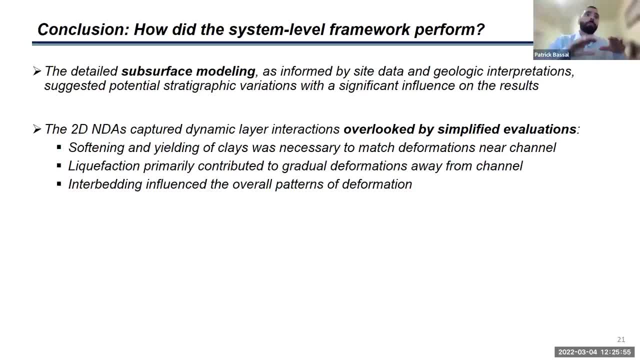 the channel And the interbedding did influence the overall patterns of deformations. Finally, both NDAs and simplified evaluations are well-suited to guide engineering decisions, as long as their limitations are recognized, And so I'd like to acknowledge some of my collaborators shown here. 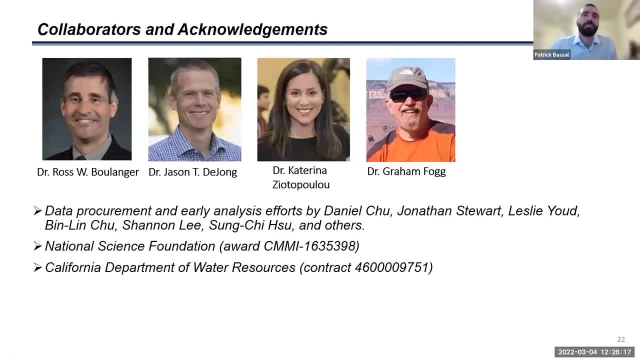 and as well as my colleagues here, And so I'd like to acknowledge some of my collaborators, as well as my collaborators here, And so I'd like to acknowledge some of my collaborators, as well as those involved in the regional site investigations and analysis for this site, and our funding agencies as well. 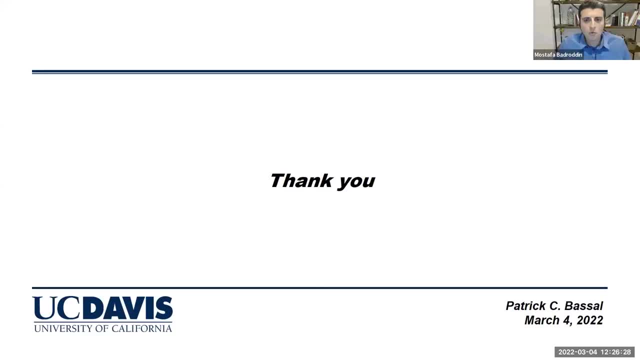 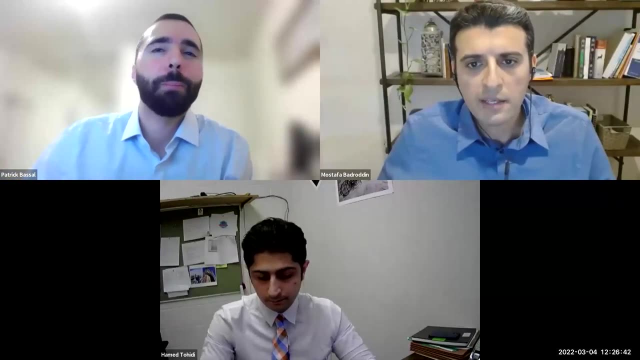 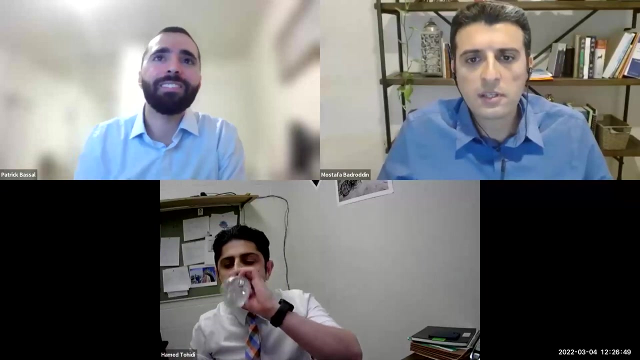 Thank you. Thank you, Patrick, for a wonderful presentation. So please feel free to put your question in the Q&A box and we will address those questions after the next presentation. So with that we go to next presentation. Our next speaker is Hamed Tohidi. Hamed is currently. 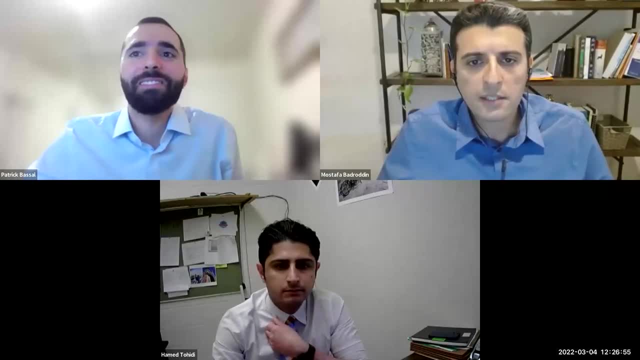 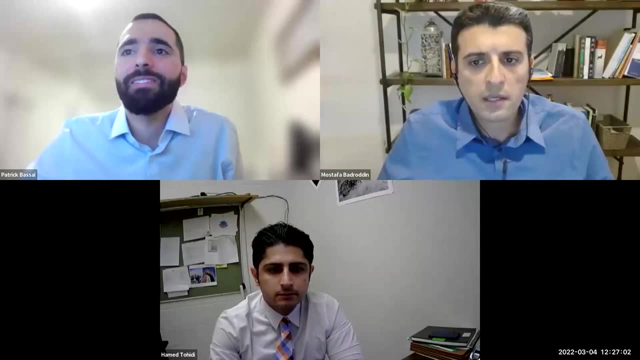 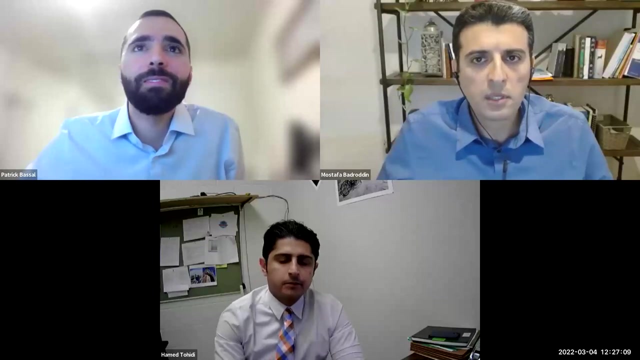 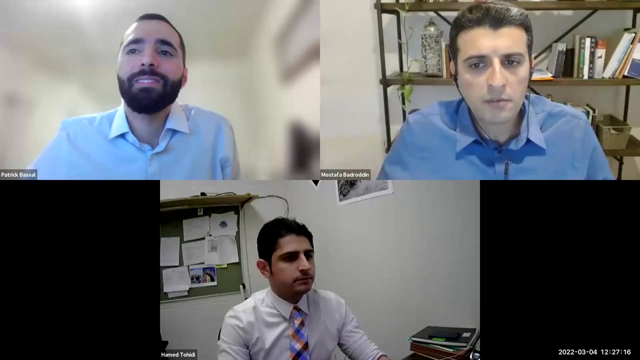 an adjunct faculty and a PhD candidate in civil engineering at the University of Memphis. His specific research area is geotechnical earthquake engineering. He's working on a five-year seismic and liquefaction hazard mapping project for western Tennessee. With that, I will hand it over to you, Hamed. The floor is yours. 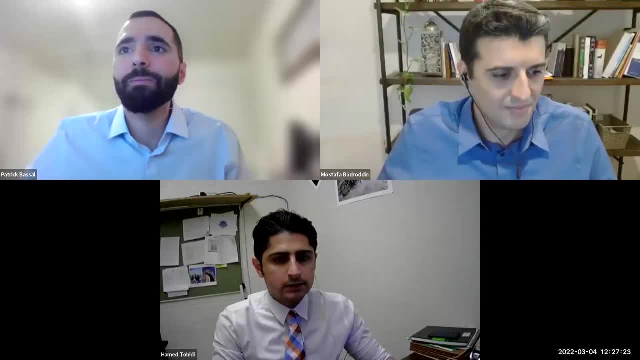 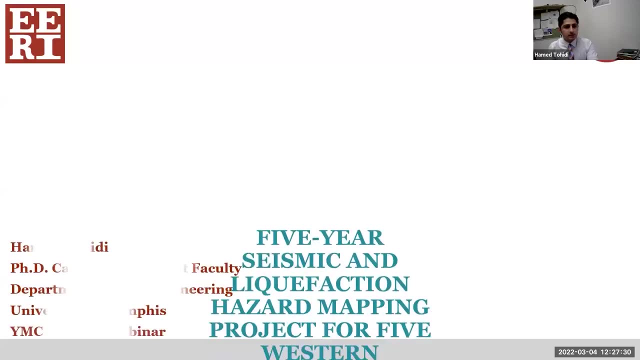 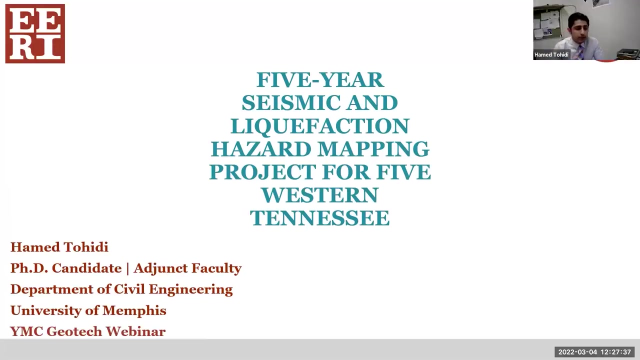 Thanks, Mustafa. I'm going to share my screen to start the presentation. So can you see my screen? Yes, we can. Okay, great, Hello everybody. I'm glad to hear, Actually, just before I start my presentation. 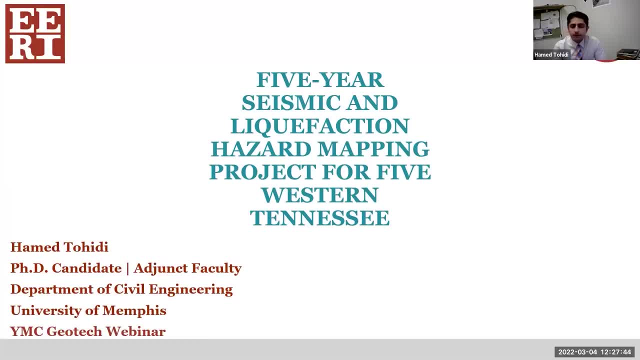 I was browsing the names in the participants and it's very interesting, very famous people in the field of seismology and liquefaction and it's a great opportunity for me to present some of my work in the liquefaction and seismic hazard analysis for the western Tennessee. So today, in this presentation, I'm going to talk. 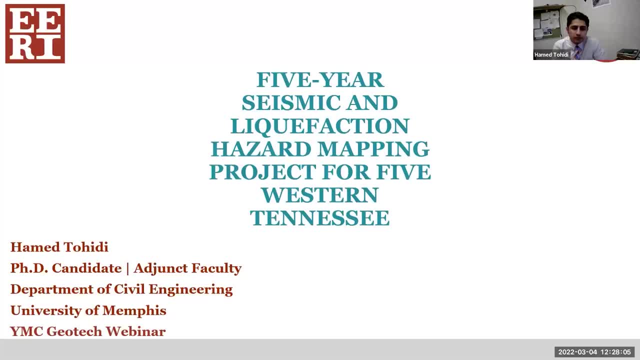 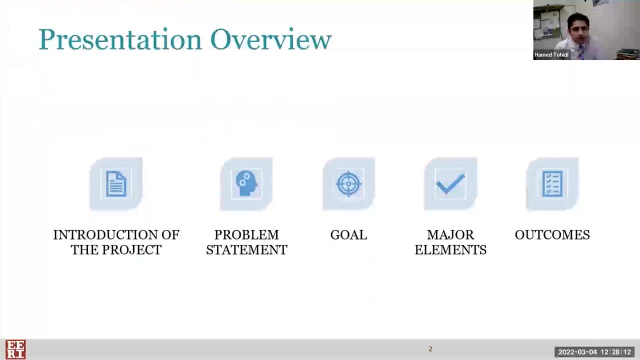 about the five-year seismic and liquefaction hazard mapping project for five western Tennessee counties that we have been working on since 2017.. So in this presentation, first I provide some background information about the project and then, by defining the problem segment of the project, I will talk about the goal of the project. 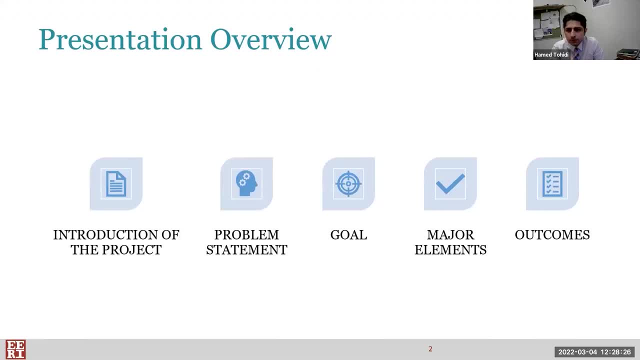 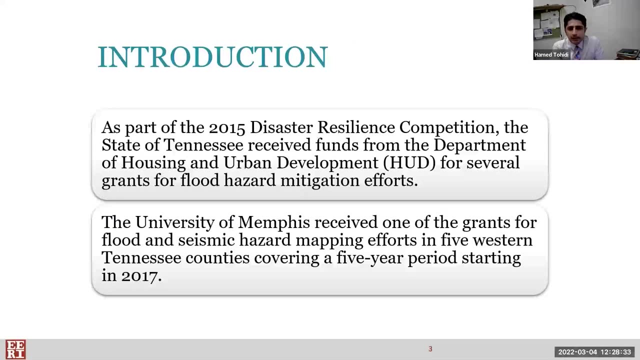 following by measure elements: and, finally, I will wrap up my presentation by talking about the expected outcome. outcomes of the project. This project has been funded by the Department of Housing and Urban Development, HUD, for several hazard mitigation project efforts at the University of Tennessee. 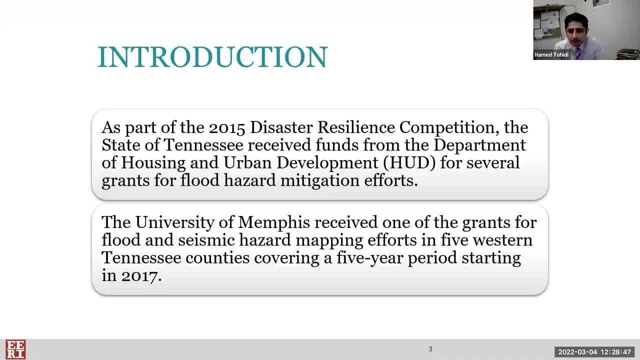 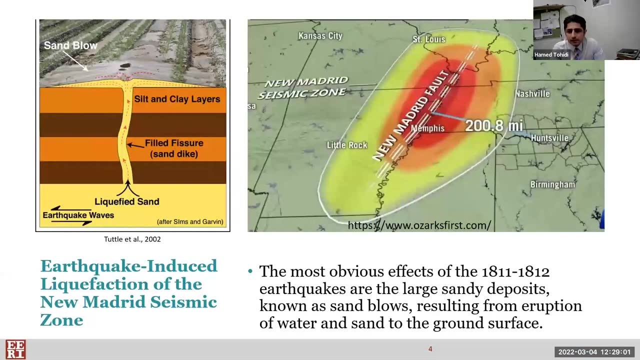 of Memphis received one of the grants for flood and seismic hazard mapping efforts in five western Tennessee counties covering a five-year period that started back in 2017.. So let's see why it's important to investigate the seismic hazard and seismic risk for the 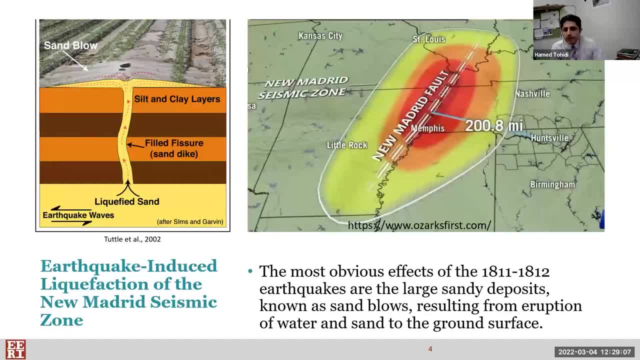 west Tennessee area. West Tennessee area is located within and adjacent to the New Madrid Seismic Zone, as you can see on your screen, which is one of the major seismic zones of the United States, and it is responsible for the huge and catastrophic earthquakes of 1811 and 1812 that occurred. 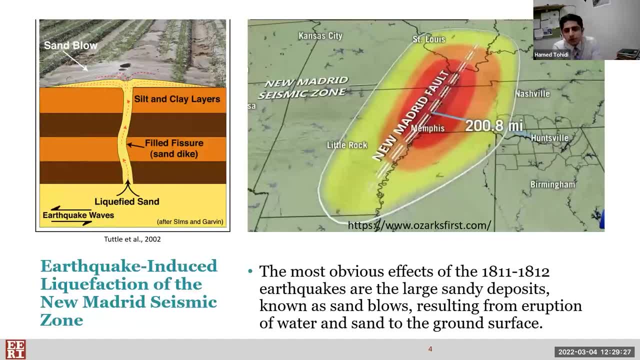 in St Louis, Missouri During the 1811 and 1812 earthquake. liquefaction and resulting lateral spraying was severe and widespread. Sand blows formed over, I think, an extremely large area about more than 10,000 square kilometers. 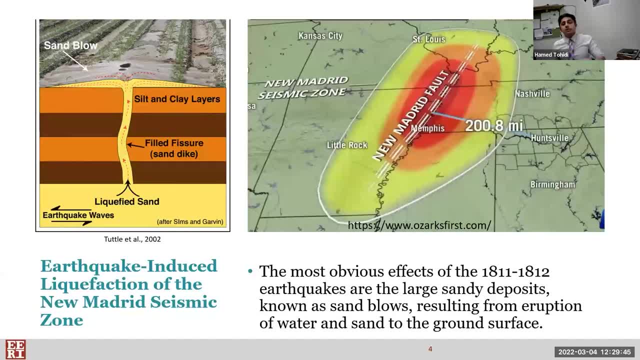 Also, the effect of the liquefaction extended about 200 kilometers northeast of the New Madrid Seismic Zone in White County, Illinois, 240 kilometers to the northwest of near St Louis Missouri and 250 kilometers to the south near the mouth of the Arkansas River. 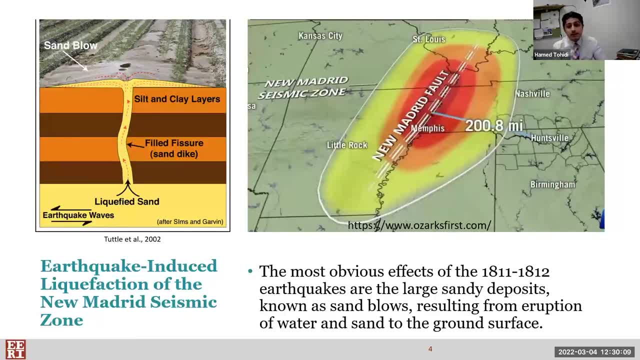 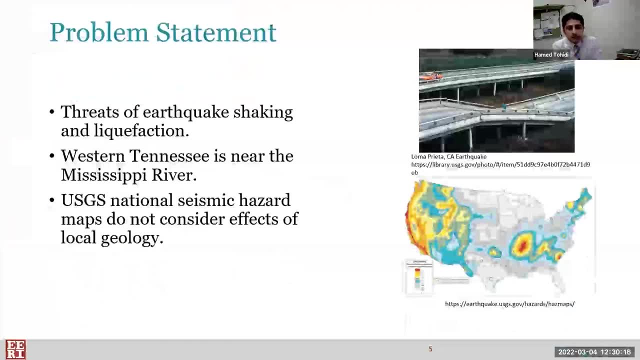 Still in these days in the New Madrid region, sand blows can still be seen on the surface today, After almost more than 100 years. So the main reason that this project is important are three faults. First, earthquake, shaking and liquefaction threatens vital structures and lifelines. 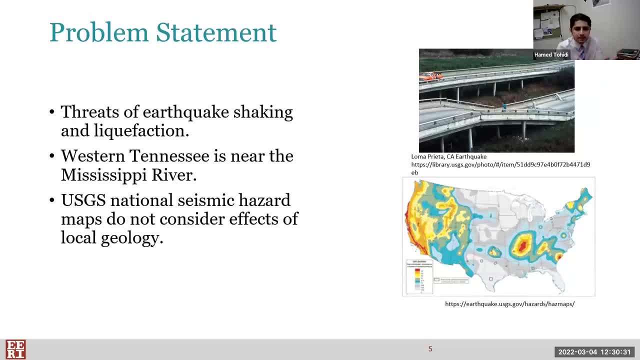 such as river levees, support facilities, port facilities, communities and transportation networks. In western Tennessee, near the Mississippi River, even magnitudes of the Mississippi River can be seen, So with magnitude 6, earthquake with magnitude 6 can potentially impair the key structures. 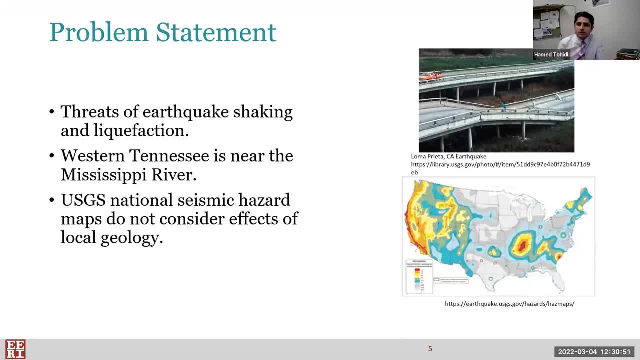 and network needed for flood control, emergency response to other hazards like wind, fire, etc. and also public safety. So one of the most important actually reasons that this project is very valuable is that the USGS National Seismic Hazard Maps. 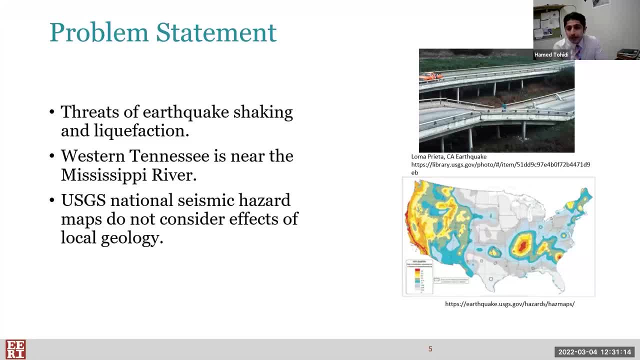 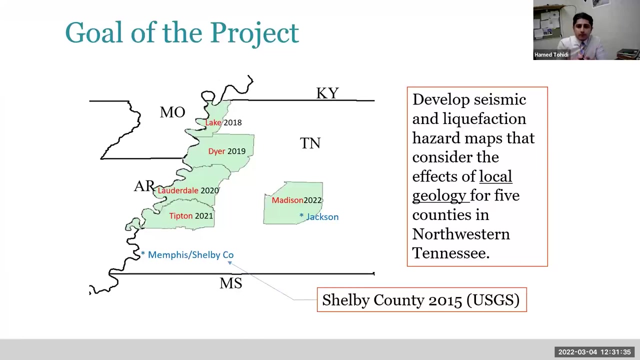 Do not consider the effects of local geology. In the other word, the local geology situation of the West Tennessee area must be considered in the attenuation relationship of the seismic hazard analysis for preventing the underestimation of seismic hazard in this area. According to the information that I just provided for you, the goal for the seismic hazard mapping 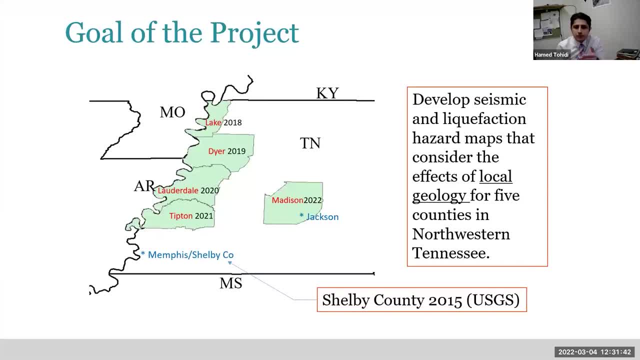 project. The goal is to develop the seismic and liquefaction hazard maps for using hazard mitigation efforts that, as you can see on your screen, there are five counties: Lake County- we started in 2018,. Dyer County- started and finished in 2019,. Lauderdale County. 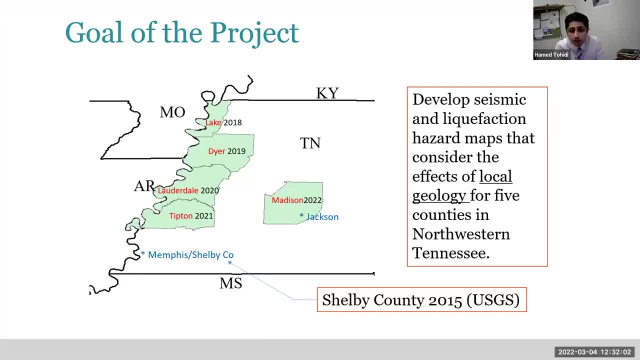 was done in 2020,. Tipton County was done in 2021, and we were supposed to finish Madison County by 2022.. However, we have done all five counties, So we have done all five counties In 2021 and currently we are working to combine data for all five counties and trying to develop. 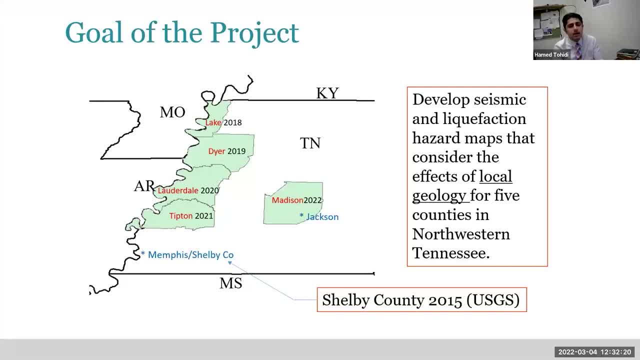 a liquefaction and seismic hazard, as well as the geology model for all five counties to get. Also, Memphis is located within Shelby County and the seismic hazard analysis of Shelby County was done in 2015 as part of another project which was funded by USGS. 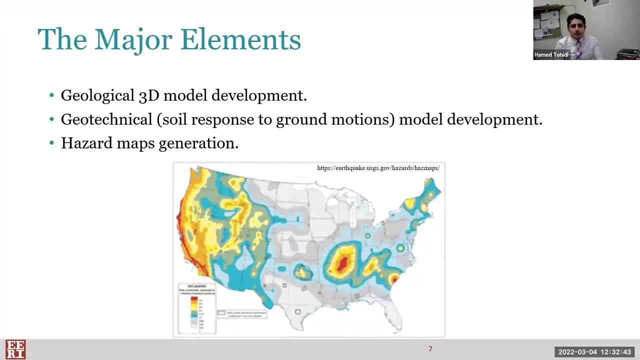 So this project consisted of three teams: geologists, geotechnical experts and seismologists. So information that gathered includes geological and geotechnical soft surface exploration logs, water table level data collection and measurements: measurements of shallow and deep shear rate velocity profiles using MASW test, which is a multi-channel analysis of 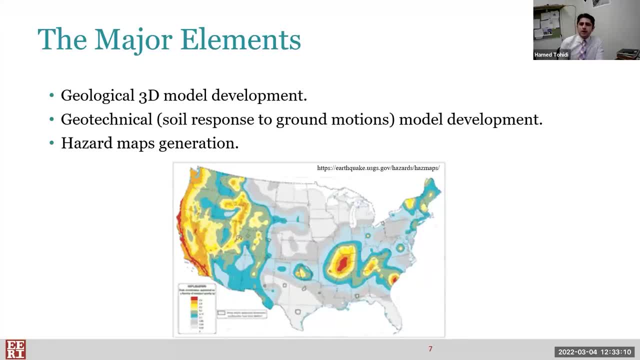 geological data. So this project consists of three teams: geologists, geotechnical experts and seismologists. This is a multi-channel analysis of surface wave and Raymar tests and the compilation of the existing shear rate velocity profiles in and around each county. 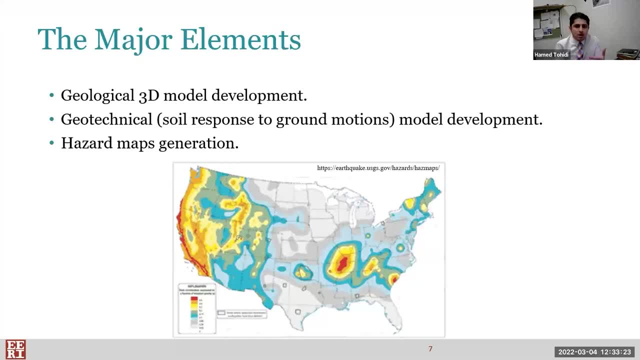 So what we are doing in this project. improvements are and were made in the 3D geological model that I'm going to show to you- a 3D geology model of each county, which is very interesting. Also, we have been developing that board. The very current groundwater level for the California Valley is 3D, That's a 3D geological model. The water level is 17,000 feet And the geological data is 1,816 feet. So each county has a 3D geological model. 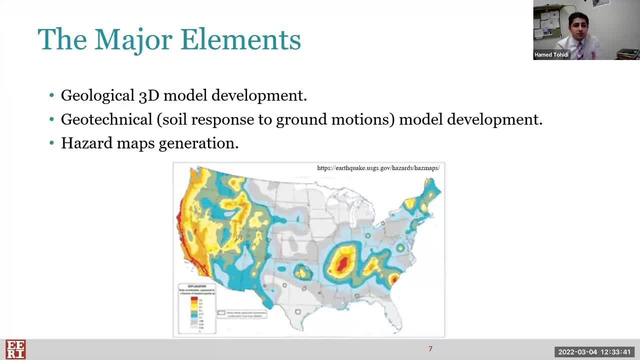 And since we have been developing this, some of these are all geological data. This is the water level of each county level model for each county, the geotechnical liquefaction probability curves and the shear rate velocity correlation with lipology model for each county. 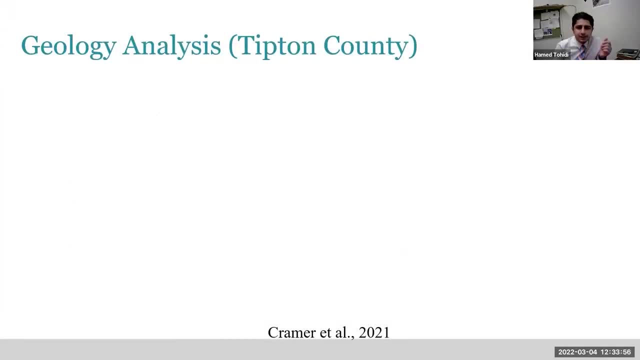 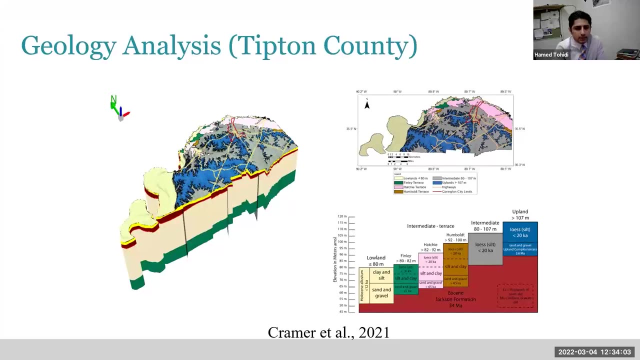 Okay, geology analysis. Here in this slide you can see an example of a geology work of the project, for example, for Tipton County, Tennessee. The topography of the West Tennessee area generally consists of lowland flood plains. 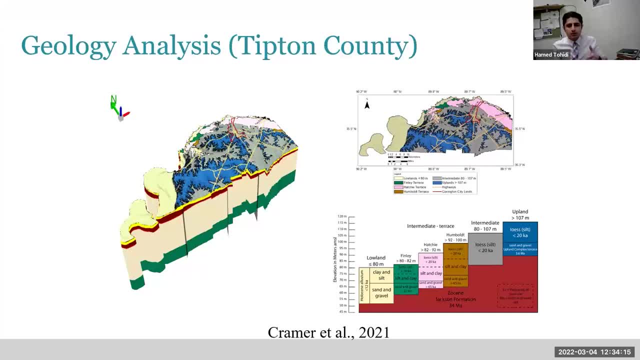 of the Mississippi River, which is the most susceptible geological unit to the liquefaction. Also, as you can see on the right corner of your screen- the lower picture, the lower figure- we have some terrace, intermediate terrace, as well as some uplands. 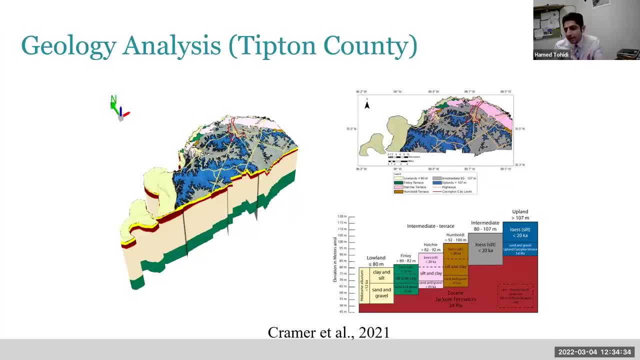 However, they are not as susceptible to the liquefaction as lowlands. Okay, As you can see here, by obtaining the subsurface data for each county, our geology team first developed this surface geology model, which is the very top right corner of your screen. 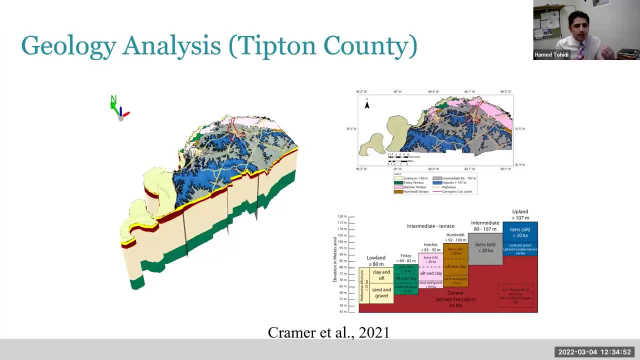 Then they develop a 3D geology model for each county. that's with the increment of five feet. Almost they go down to almost 100 feet for each county, which I think is a very valuable model. I have to thank Dr Roy Manners. 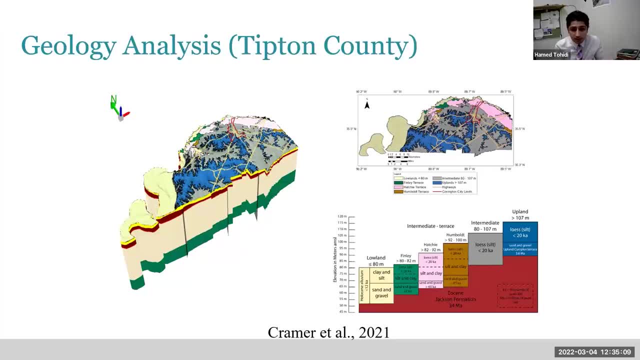 They, as well as is the students that helped us in this project to develop these very great models. as you can see on your screen, The soil profiles of this area, as you can see, are mostly loess. Loess is a very loose silt which is very common in the Tennessee area near the Mississippi. 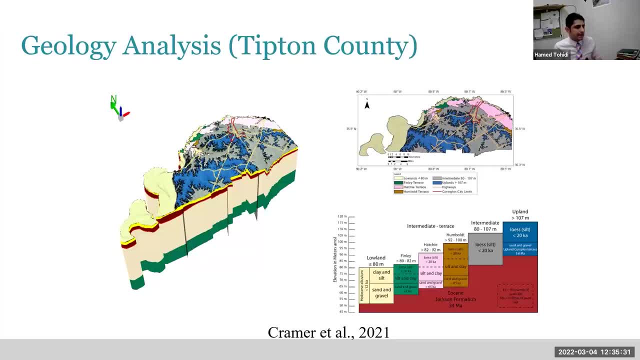 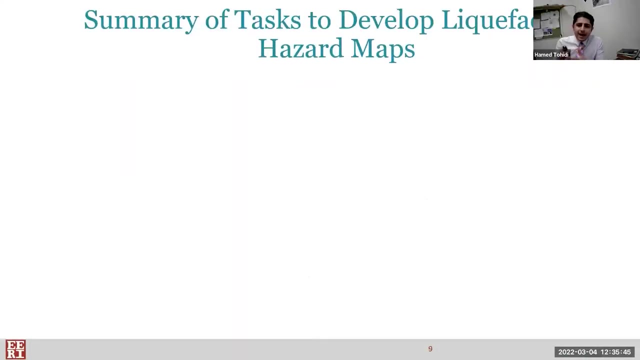 River. Also, we have sand and gravel, silt and clay, but the amount of sand and loess is way more than, for example, dense clay. So that's the reason we are doing the liquefaction analysis for this area. So, based on the background information, now let's talk more specifically about the development. 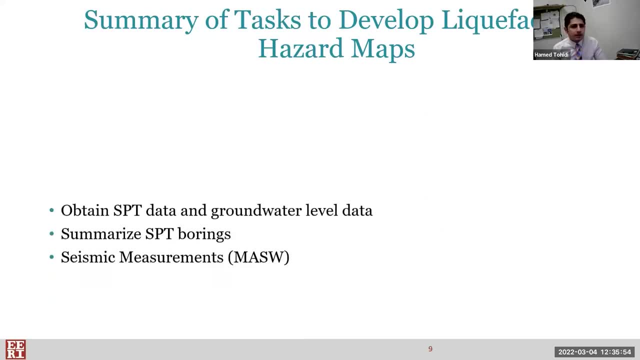 of liquefaction hazard maps in this project, A summary of geotechnical analysis conducted to develop liquefaction probability curves, following by liquefaction hazard maps, are provided in this slide. First, we obtain a standard penetration test as well as cone penetration tests from different 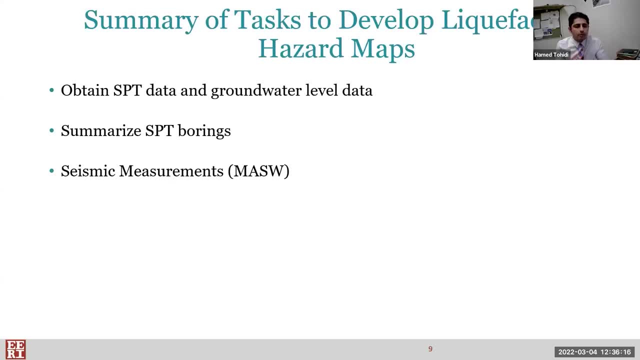 organizations like Department of Transportation or Army Corps of Engineers. Also, sometimes the private companies help us out here to add more data to our database. Then because most of the soil borings we receive are very old and they were drilled in 1990 or 1980. 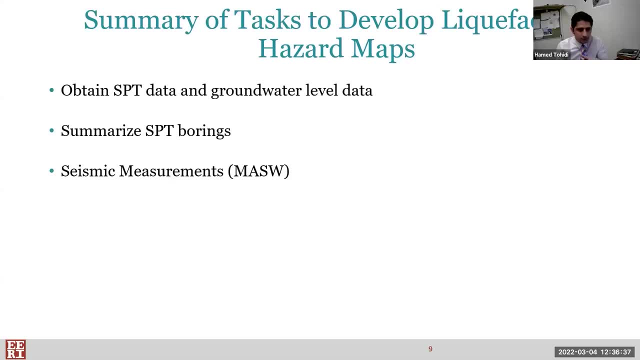 Dr Roy Manners, The groundwater level has been changed since then, so we cannot use the recorded groundwater level at the time of drilling the standard penetration test for it. Due to this reason we have to also obtain, and sometimes also measure, the most current. 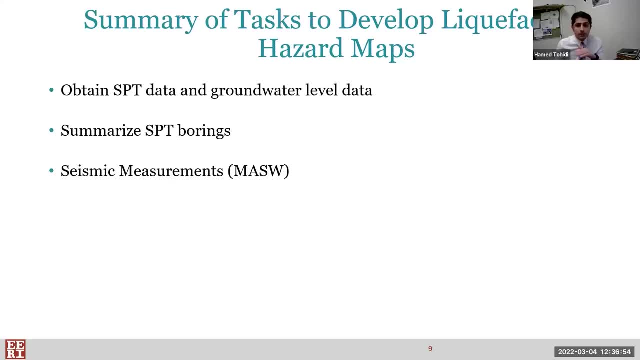 groundwater level for each county to make sure that we are doing the right analysis for liquefaction. After that the SVT soil borings has to be summarized for soil type for standard penetration tests, Also sometimes to cover some of the areas that we do not have that much SVT borings. 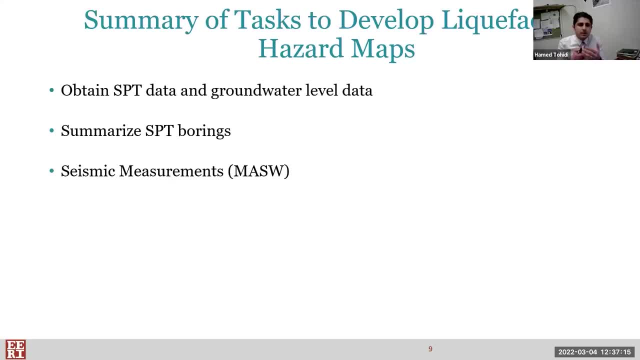 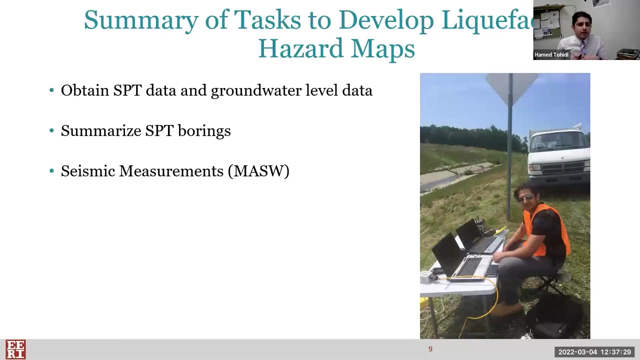 we go out and do the seismic measurement using MASW. we measure shear wave velocity And for some parts of each county our liquefaction analysis is based on the MASW test shear wave velocity. As you can see, I have been done that a lot out in the field, which was not fun. 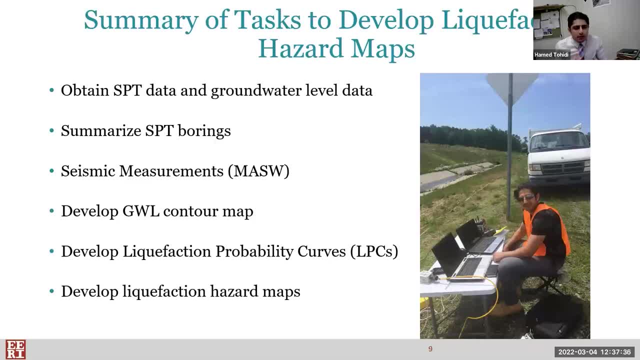 Dr Roy Manners. Dr Roy Manners. Dr Roy Manners. After developing the groundwater level contour map and summarizing the SVT borings or shear wave velocity profiles, we developed a liquefaction probability curves, And then the liquefaction probability curves for each specific geology units are going. 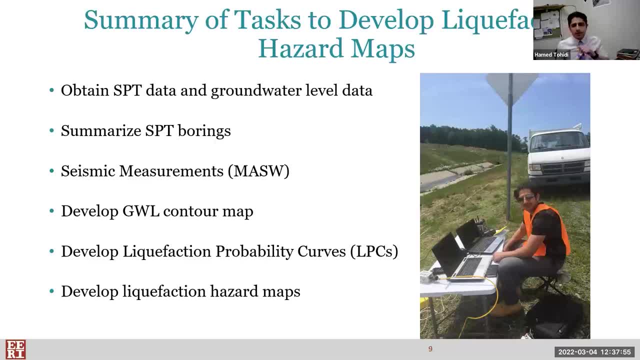 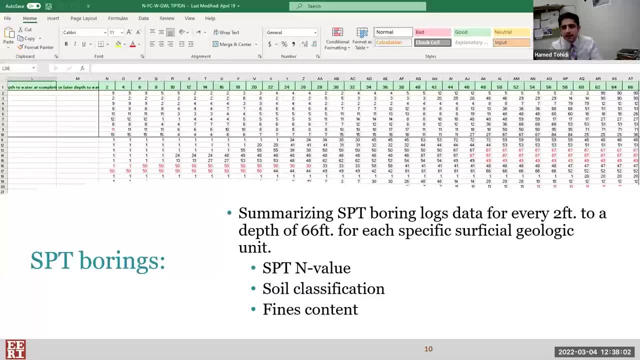 to contribute to development of the liquefaction hazard maps. Okay, In this project, after obtaining data from various organizations based on something, some specific criteria, we have to select borings. Borings- all are not applicable in liquefaction analysis because sometimes they are not deep enough, Sometimes they have too many missing. 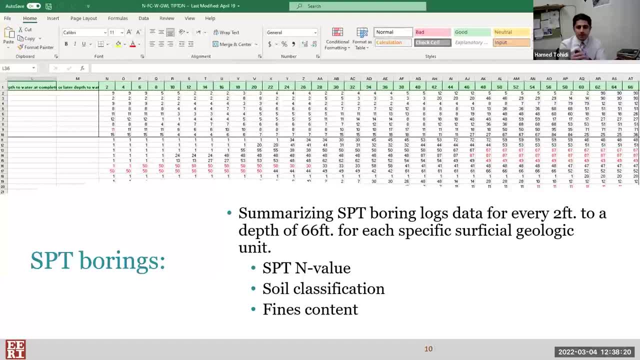 end values. Sometimes the soil type has not been recorded. Due to this reason, we have to make sure that we are selecting applicable borings to do the liquefaction analysis And after that, because the soil profiles of West Tennessee are very stratified, we have to summarize the borings. 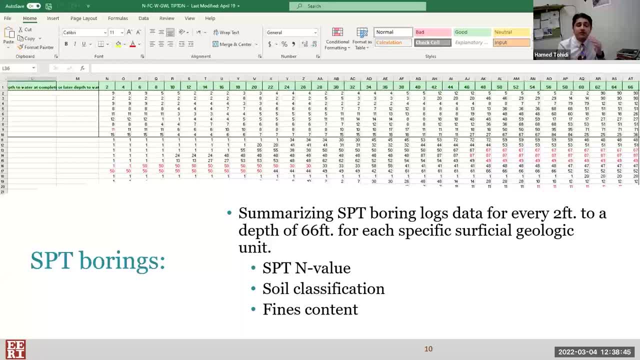 for each two feet depth increment to a depth of 66 feet or 20 meters, What we summarize for each SPT: boring End value, soil classification and fines content, which are the three most important parameters to do the liquefaction analysis. 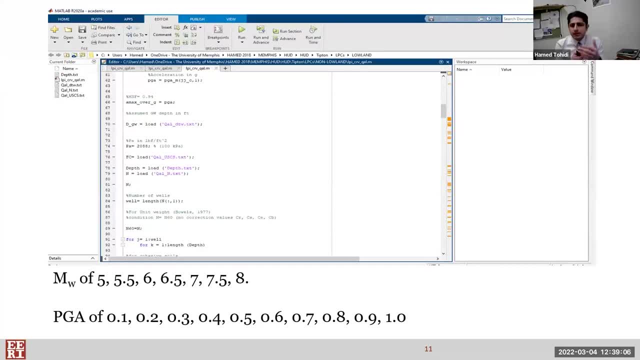 Okay, Based on the seismologist team research and recommendations for each county, we perform the liquefaction analysis for earthquake magnitude range 5 to 8, with increment of 0.5, and peak ground acceleration range of 0.1 to 1 with increment of 0.1.. So I can say that for 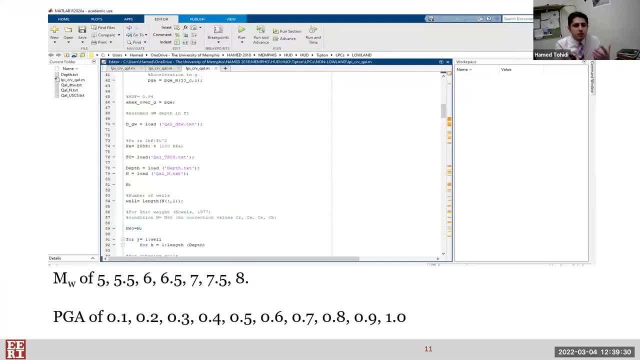 a total of 70 combination of earthquake scenario, we have to do the liquefaction analysis. Okay, Imagine that we have numerous boring logs for each county, that each boring is summarized for every two feet depth increment to a depth of 66 feet for liquefaction analysis And each analysis must be done for 70 earthquake scenarios. 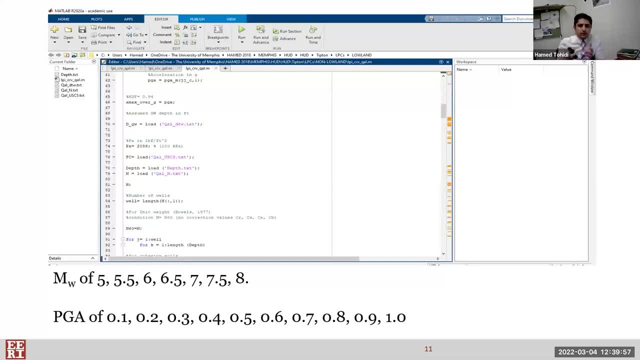 Of course, it's not doable with hand. I mean it's doable, but it takes forever. I have developed a coding MATLAB that goes through each boring read, all data for each county, go through each specific earthquake scenario and develop. 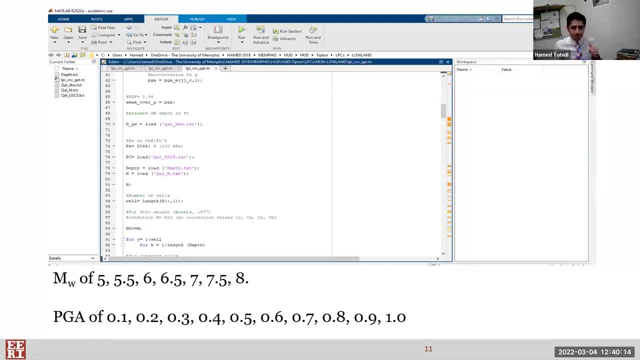 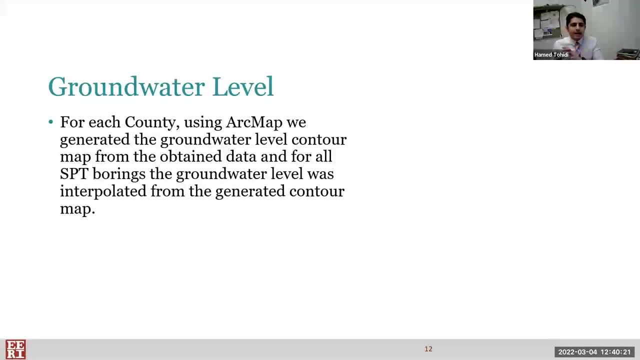 the liquefaction probability curves for each county and specifically for each surface geology unit. Also, as I mentioned to you, because most of the soil borings we have are very old and the groundwater has been fluctuated since then, We have to be the most current because currently, 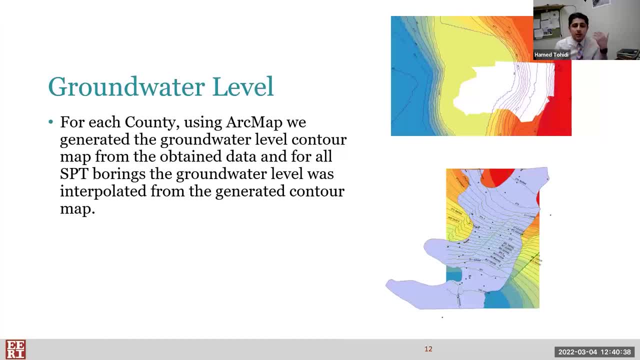 the groundwater could be shallower or sometimes deeper than whatever was recorded back in 1990 or 1980.. So by obtaining data from, for example, United States Geology Survey or other organization also, sometimes we do it, we measure the groundwater ourselves, our team out in the field. 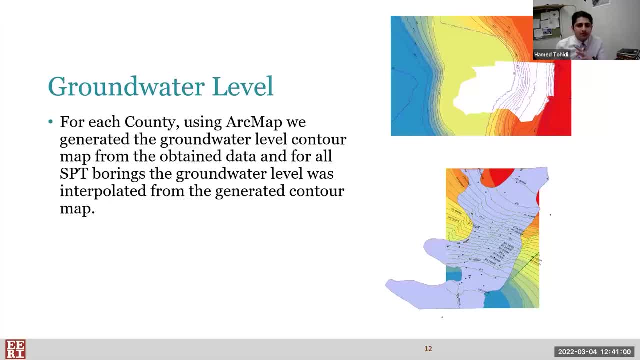 We try to develop contour map, ground level contour map for each specific count. For example, here you can see the upper figure is Dyer County, Tennessee. The lower figure is Lake County, Tennessee. Also, we have done this for each five counties Currently. for each county we have the most current groundwater. 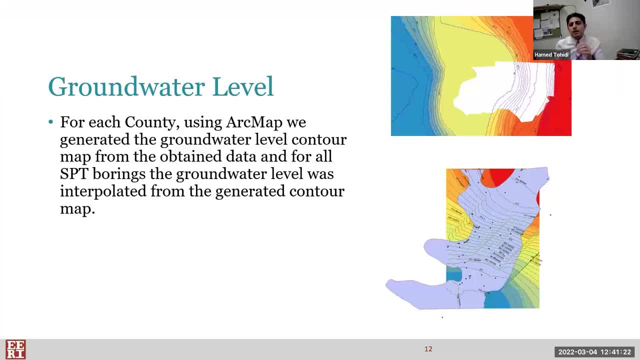 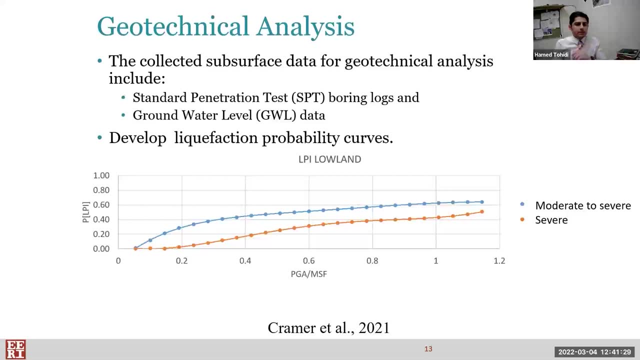 level, the most current 3D geology model, the most current seismic and liquefaction hazard maps. Here you can see some liquefaction probability curves for the moderate to severe, as well as severe probability of liquefaction. Also, keep in mind, whatever I'm talking about, liquefaction here. 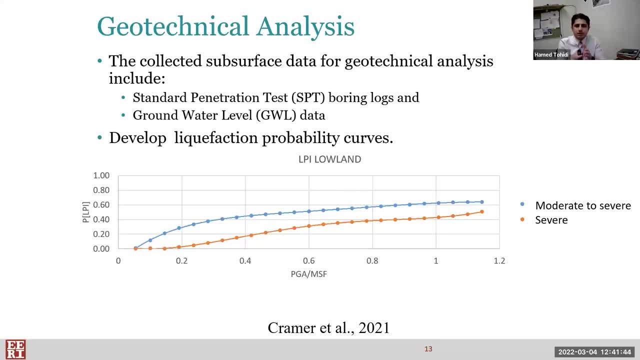 is liquefaction surface manifestation, because this project has been done in regional scale, not site specific. So what are liquefaction probability curves? LPCs are curves that predict the probability of surface manifestation of earthquake induced liquid action for various earthquake scenario. On your screen you can see each curve has different. 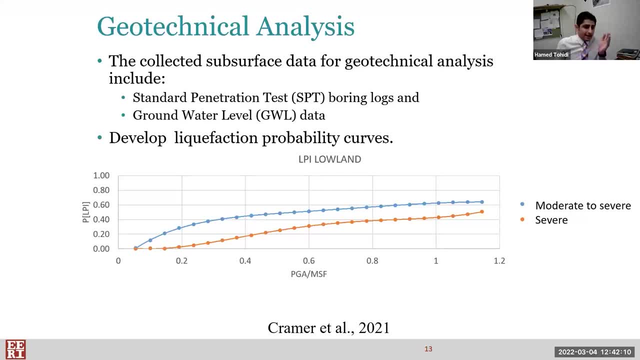 points. Each point represents one earthquake scenario, And here, however, I kind of reduce the amount of points on each curve. But for each county we have developed 70 points to come up with liquefaction probability curves. This liquefaction probability curves can be developed based on: 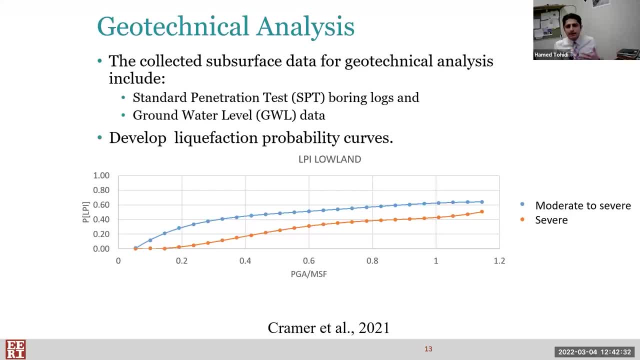 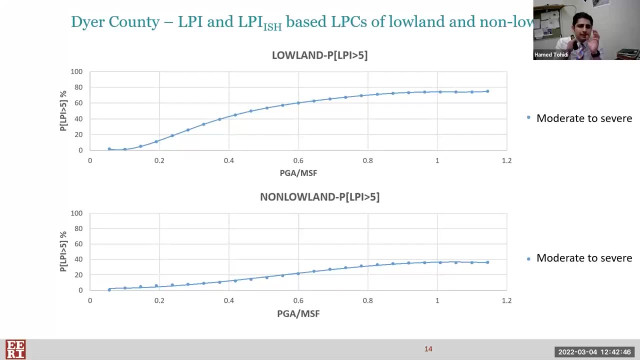 SPT, CPT, shear wave velocity profiles. That's mostly for the HOT project, the project I'm talking today. We have used a standard penetration test data. Okay, as I mentioned, this liquefaction probability curves has to be developed for specific geology. 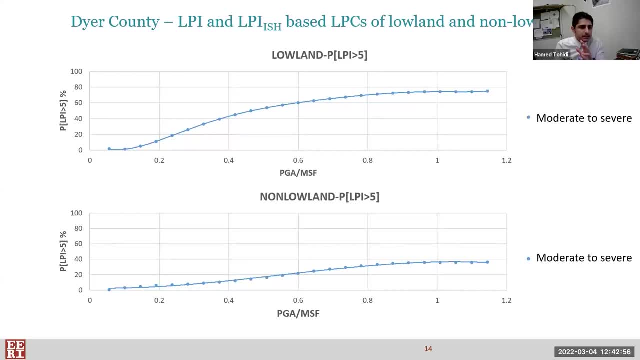 units For West Tennessee. excuse me, for West Tennessee area we have different geology units: Lowlands, intermediate terraces and uplands. But the most susceptible geology unit to the liquefaction is lowlands And usually for lowland area of each county we have had enough soil. 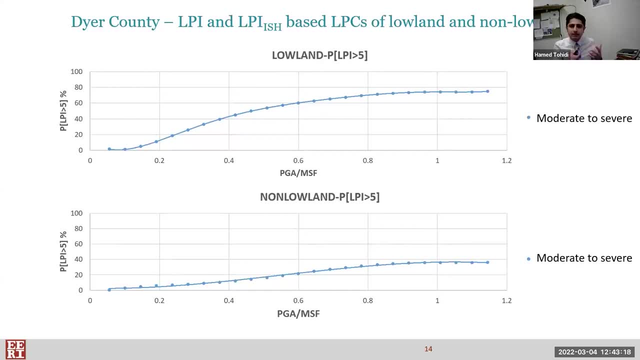 borings to perform, I mean statistically. we had a reliable enough number of soil borings to do the liquefaction analysis for lowlands, But for terraces intermediate and uplands, which they are less susceptible to the liquefaction, we didn't have enough borings. 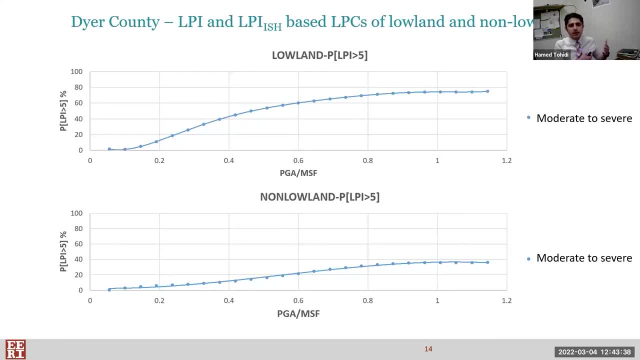 It means that, for example, for upland we had only five borings, or for intermediate we had only 20 soil borings. So instead of developing the liquefaction probability curves for each specific intermediate terrace and upland, we combined those data. 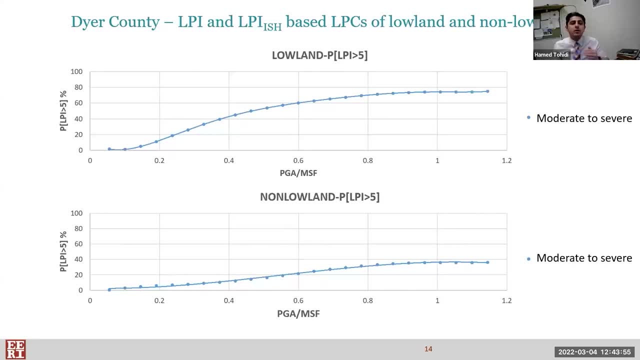 and add them together to develop the liquefaction probability curves for non-lowland areas And here, for example you can see the upper curve is for lowland area probability of moderate to severe liquefaction surface manifestation. As you can see, there is a huge difference between lowland. 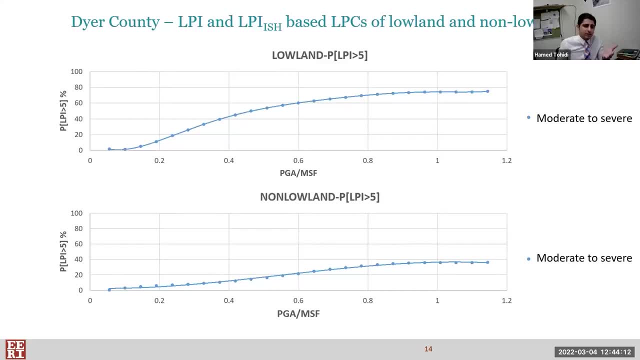 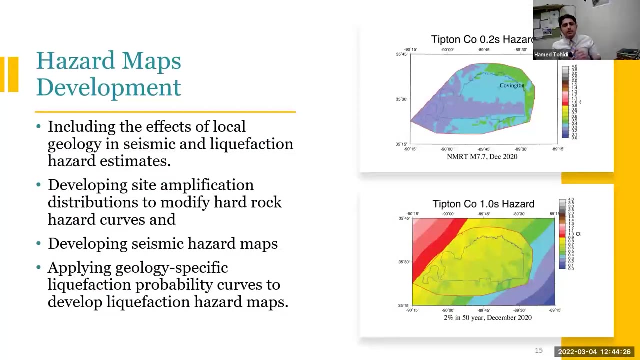 probability of liquefaction and non-lowland probability of liquefaction, specifically for more intense earthquake scenario, which is the increasing x-axis. Okay, To develop the liquefaction hazard map, our seismology Dr Chris Kramer- I have to thank him too- a standard methodology for 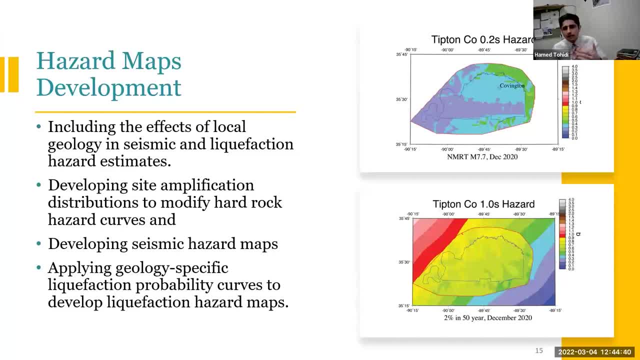 including the effect of local geology in seismic and liquefaction hazard estimates, has been used in this study Developing the site amplification distribution to modify hard rock hazard curve to geology-specific hazard curves. By geology-specific I mean lowland and non-lowland. 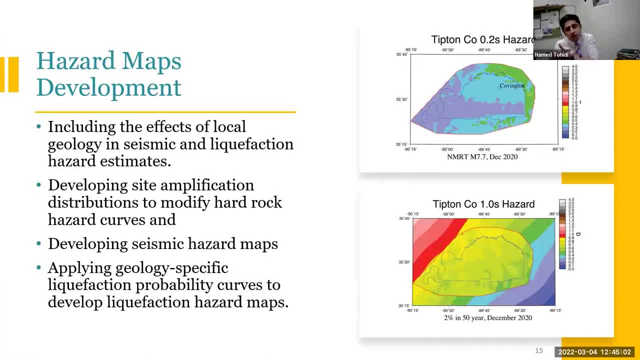 And then develop the seismic hazard maps and applying the geology-specific liquefaction probability curves to develop the liquefaction hazard maps for each specific geology unit And finally the combination of those gives us a complete map for each county. For example, here you can see the liquefaction hazard. in the right side You can see the. 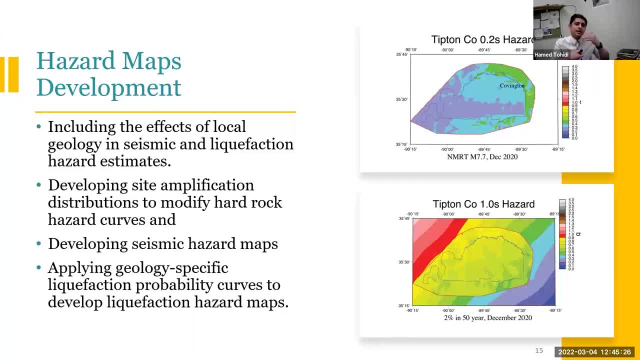 seismic hazard maps for Tipton County And then by including the effect of local geology as well as the liquefaction probability curves. these maps can be converted to the liquefaction hazard maps And also for each county we have developed two types. 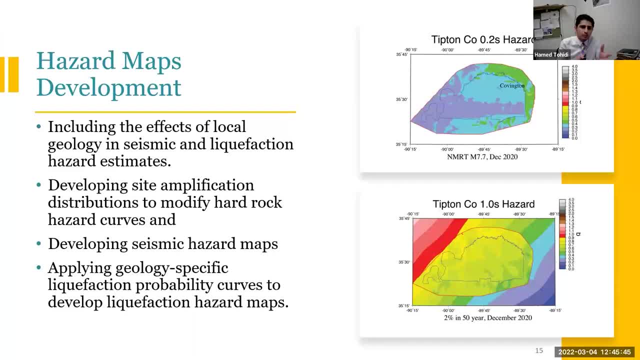 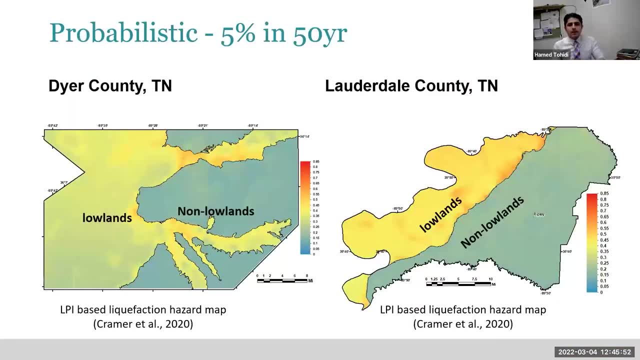 of maps- probabilistic and deterministic maps- that in a minute I'm going to talk about more about those maps. Okay, Let's take a look at the liquefaction hazard maps here: Dr Chris Kramer, Dr Calif. Dr Chris Kramer. 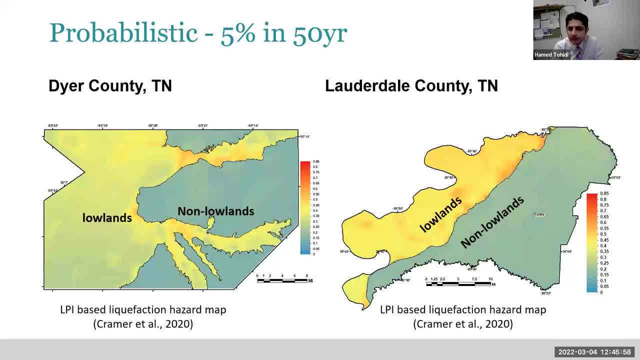 Dr Calif, Dr Calif, Dr Calif. Here we can see Dyer and Lauderdale County tents. These maps are designed to give general public, as well as land use planners, utilities lifeline owners, a better tool to assess their risk from earthquake damage. 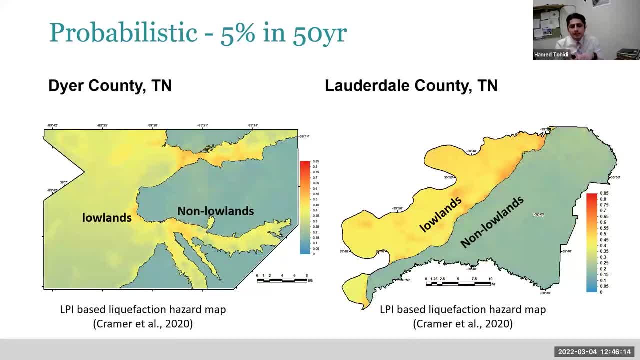 As I mentioned, we have two types of maps: probabilistic and deterministic. That in this slide you can see the probabilistic maps for probability of 5% exceedance in 50 year, As you can see, of course, the probability of liquefaction. 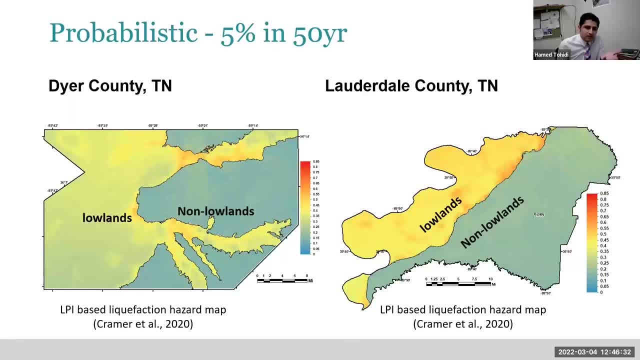 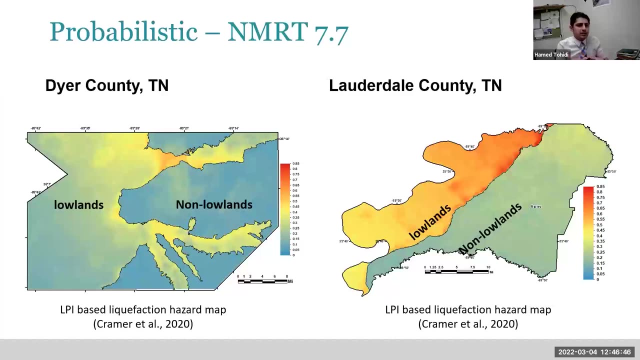 for lowland areas way higher than non-lowland And if we kind of take a look at numbers more closer we can see that for non-lowlands the probability of liquefaction surface manifestation is negligible. Also, these maps has been developed for different earthquake scenarios. 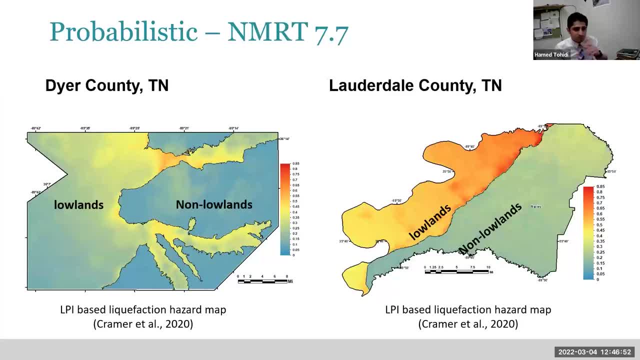 which we call it deterministic maps. Sorry for the title, it should be deterministic. These maps for Dyer and Lauderdale County, for new matrix, a real foot thrust magnitude of 7.7.. As you can see again, lowlands have higher. 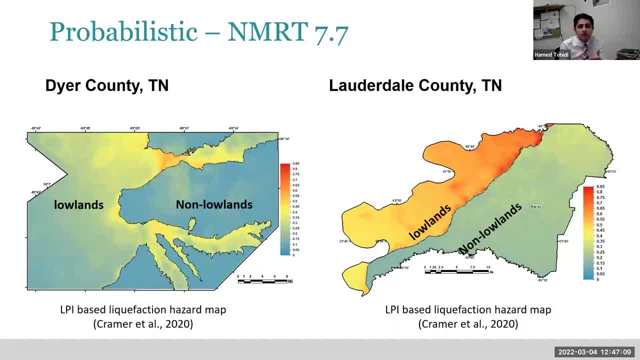 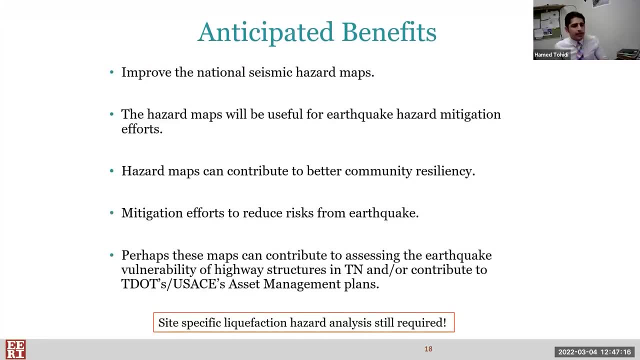 and significantly higher probability of liquefaction than non-lowland areas. So let's talk about the anticipated benefits of these maps. The new hazard maps will improve the National Seismic Hazard maps because the new maps incorporate the local standards, the local geology. The hazard maps will be useful for earthquake hazard mitigation efforts. 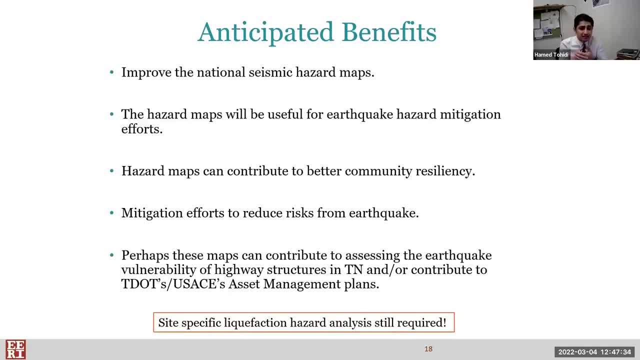 in the five western Tennessee counties. Also, these hazard maps can contribute to a better community resiliency through a better estimates of earthquake hazard needed for land use planning and mitigation efforts. So the mitigation efforts to reduce risk from earthquake. hazard maps protect and improve the public safety at all socioeconomic level. Also, perhaps these maps can contribute. 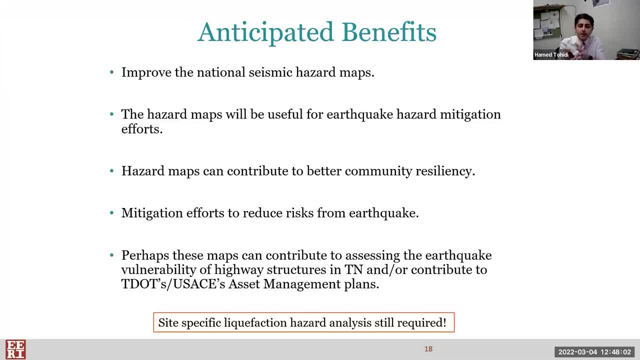 to assessing the earthquake vulnerability of highway structures in Tennessee or contribute to Tennessee Department of Transportation's and Army Corps of Engineers asset management plans. But again, keep in mind this project was done in the regional scale and only for delivery of liquid-faction surface manifestation, Still for site-specific liquid-faction hazard analysis. 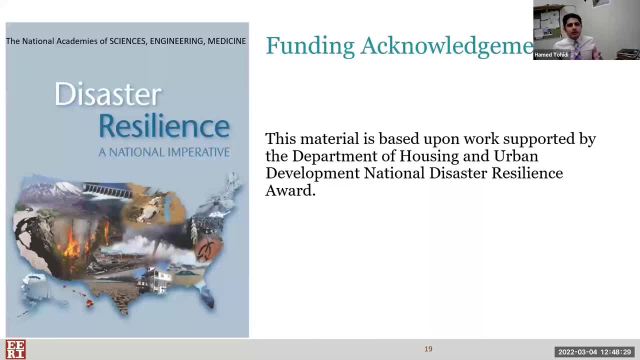 is required. Also, I have to thank the Department of Housing and Urban Development for funding this project. It was a great project. However, I learned a lot and also I had chance to present this project results in different webinars, conferences, And also I'm grateful to the 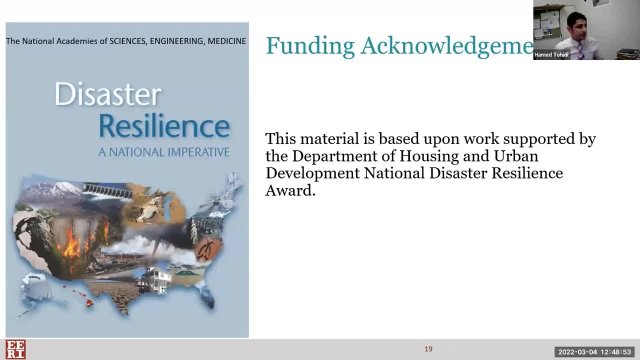 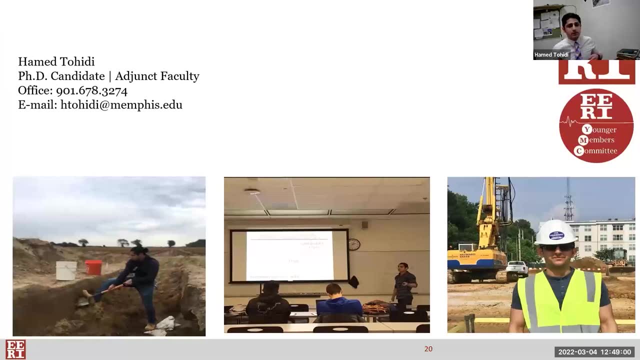 Department of Housing and Urban Development for funding this project, and I'm going to use some of the results for my PhD dissertation. By that, thank you so much for paying attention to my presentation. Again, my name is Hamed Touedi and you can see my email address on your screen in case you have any questions And also 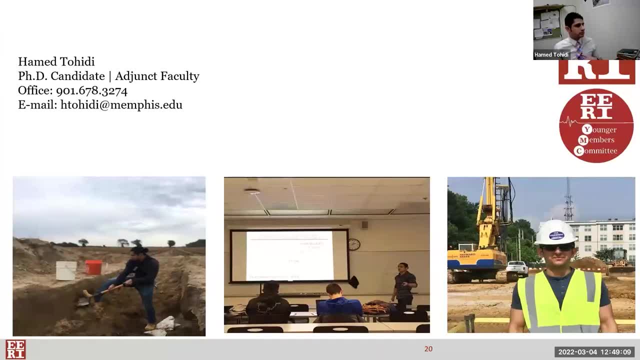 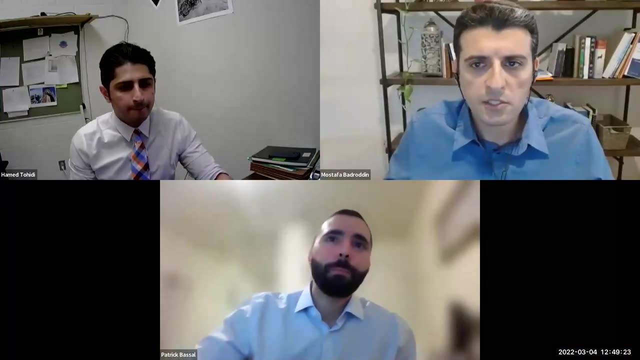 for each county. we have a report that you can reach out to me, and I will be more than happy to share the reports with you. Thank you so much. Thank you, Hamed, for a wonderful presentation. Thank you, So let's start the Q&A session. We received a few questions so far in the Q&A box, So please. 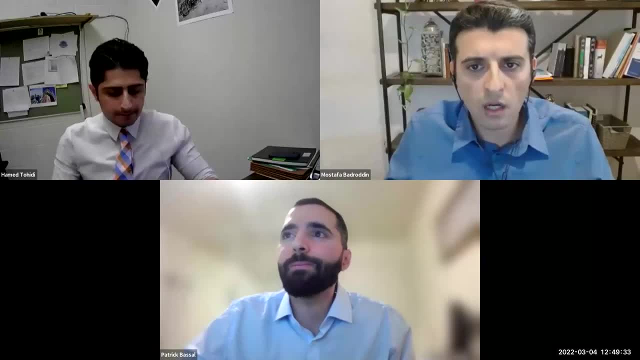 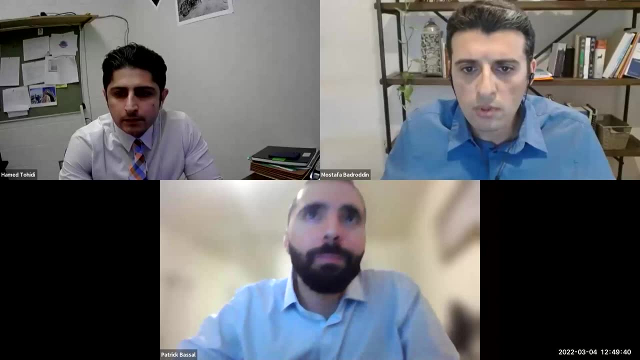 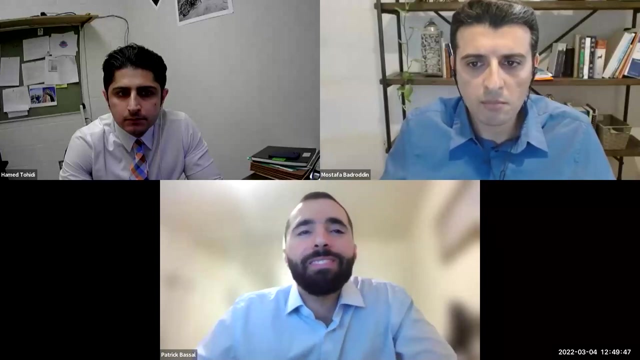 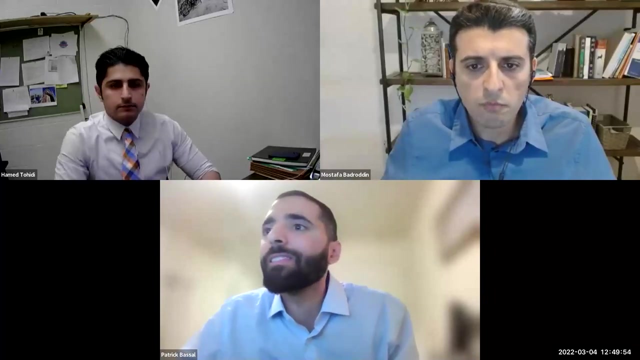 feel free to put your questions on the Q&A tool. We try to address questions as many as possible, So let's start by Patrick. So please excuse me if I don't pronounce your name correctly. We got a question from Wibi Jean for Patrick. Thanks for your excellent presentation. 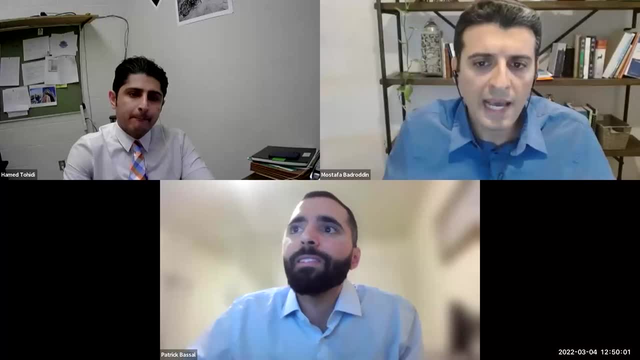 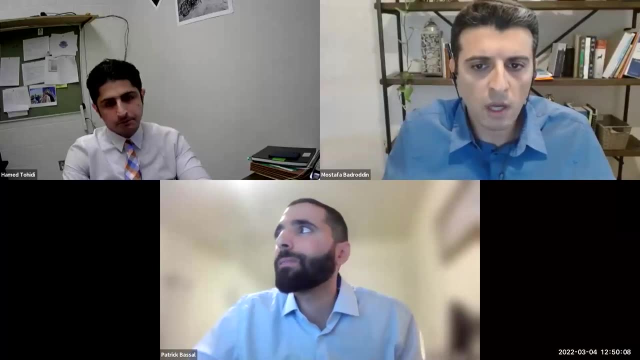 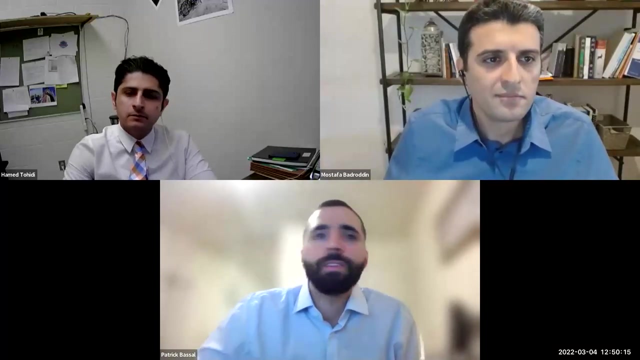 Do you have some suggestions on how to calibrate parameters for these complex constitutive soil models according to different type of information, for example SPT, CPT, element level lab data? Yeah, it's a good question And I didn't go into too much depth for my presentation on this. 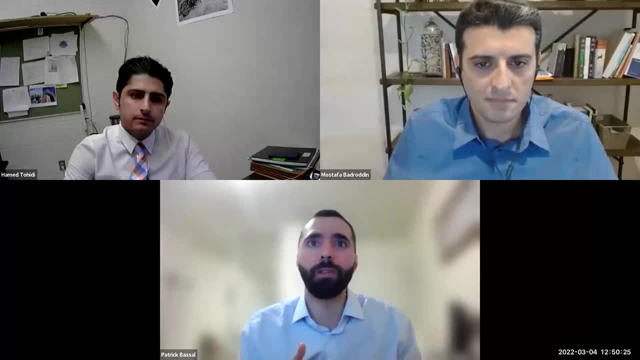 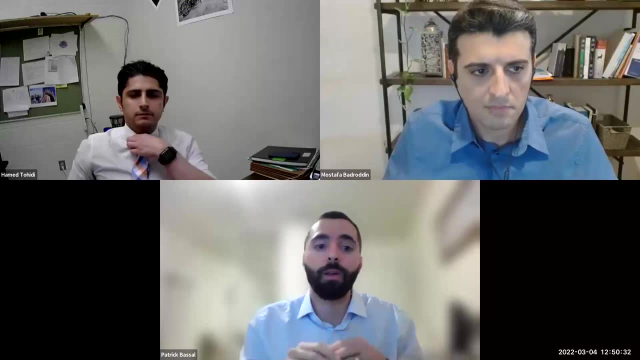 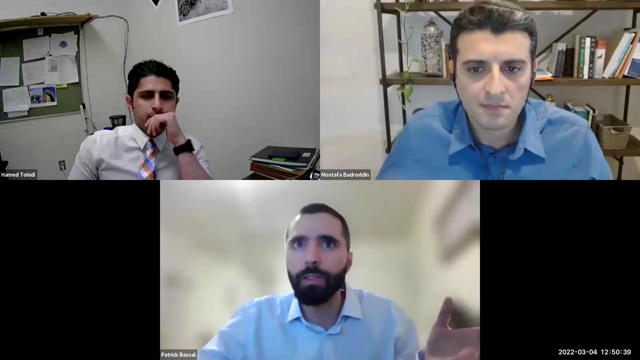 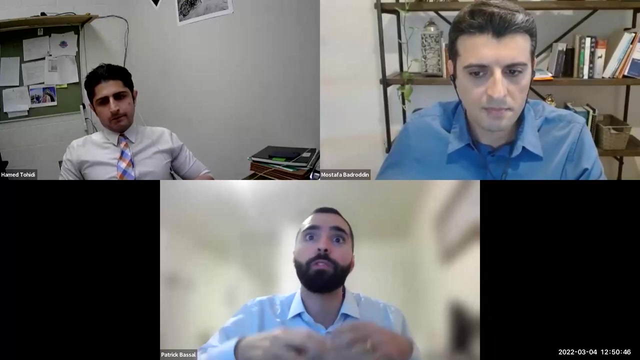 But I think it does really depend on what data you have available and also what mechanism you're looking at. And so if all you have available is SPT data from borings or CPTs, then typically the constituent models that I use, at least the PM4-SAN, PM4-SIL- they have these primary input parameters that you can use that typically work well for most situations. 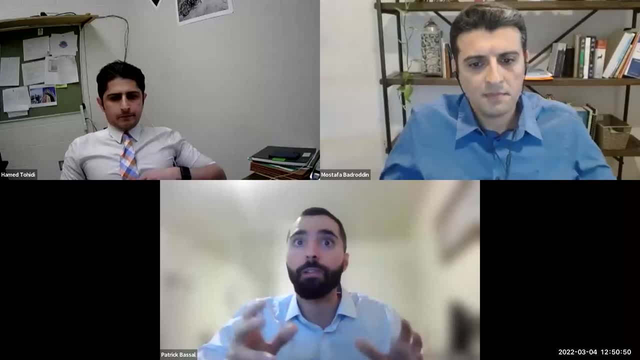 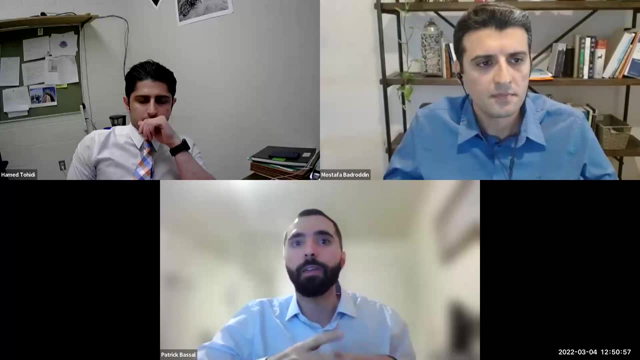 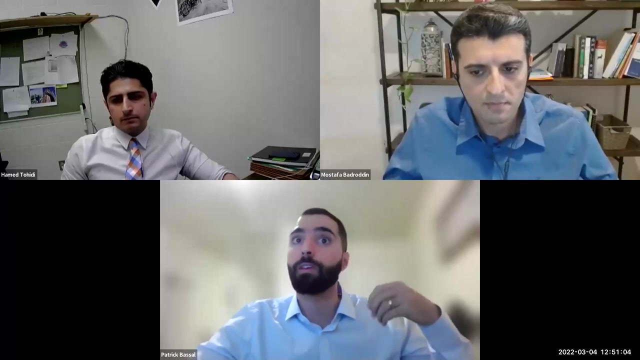 And so, again, every situation is different, But typically there are some primary input parameters. Relative density is one. There's a contraction rate parameter, which is based just on using a simplified analysis to get your cyclic resistance ratio. It's just such as I'm using the Anderson-Bohlen-Jay 2014 method, for example. 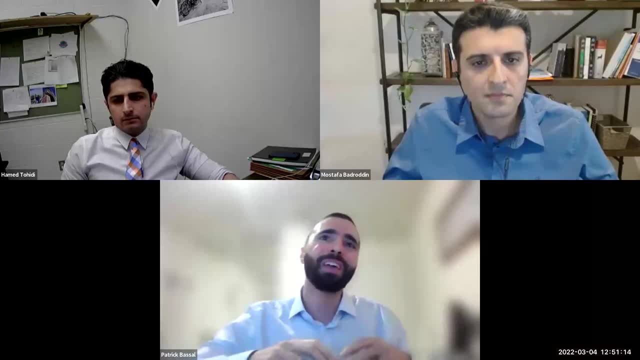 Or sorry, Bohlen-Jay Anderson-Bohlen-Jay 2014.. You can use that And you can ultimately calibrate your parameters. You know, using that that makes some understanding from simplified methods as well as the data you have. 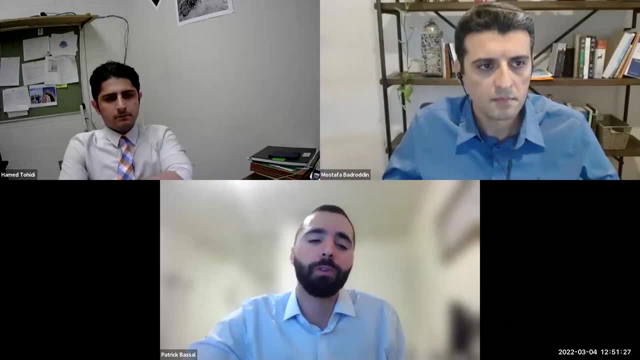 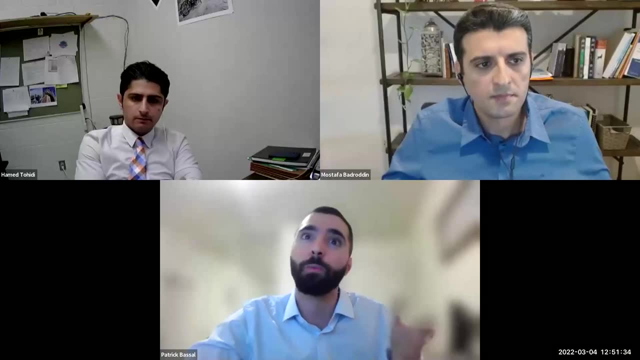 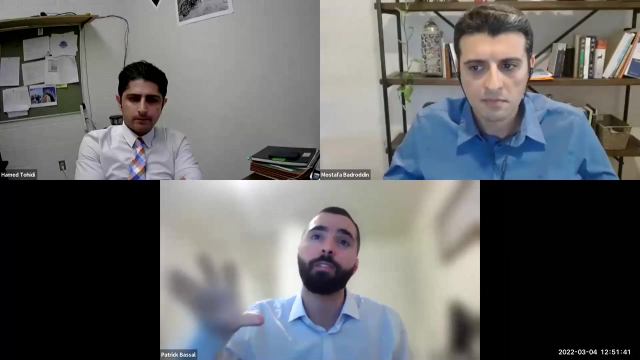 But there are. depending on what data you have, you could also account for other factors or other features. You can look at post-cycle fraction and shear strain accumulation. That's a big thing. a lot of research is now going into And I've actually written a paper on it for this case study site. 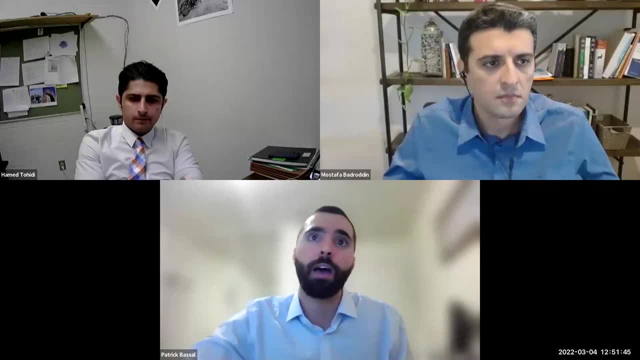 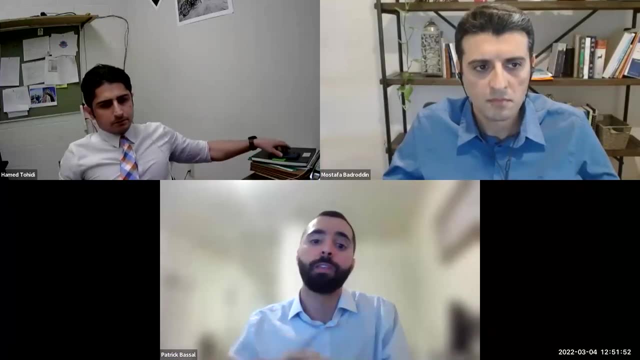 I did look at varying that And so, depending on what data you have, you could better calibrate For situations that might affect lateral spreading formations more strongly, And you can also look at that. you know, without having that data you can kind of see what effect having that data will have. 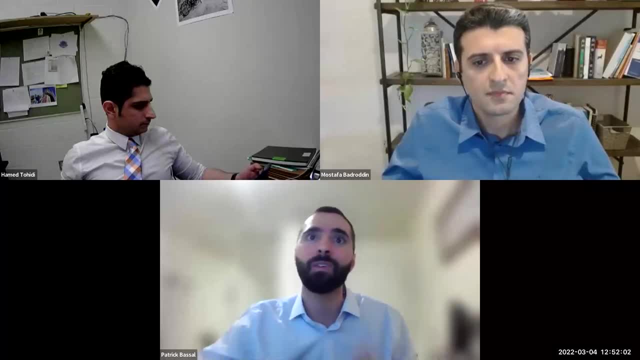 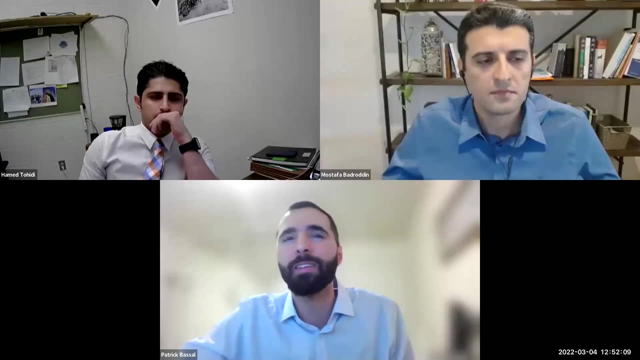 That can inform you whether you should do more advanced laboratory testing, Whether you should do, say, cyclic direct, simple shear testing, or not. So it really does depend on the data you have Also, of course, another important parameter for our dimension: 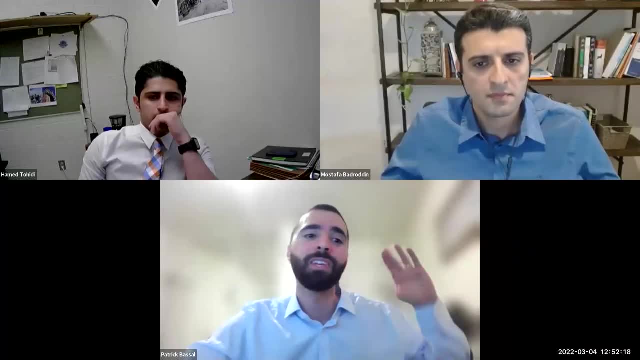 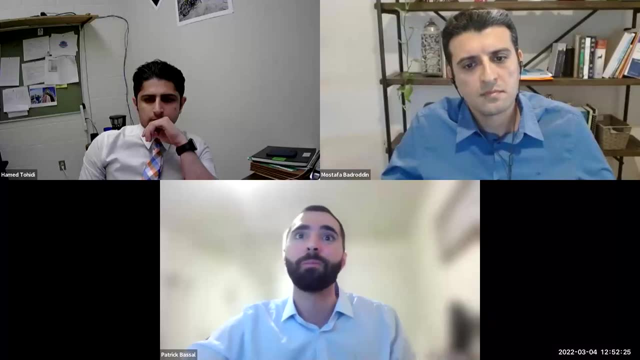 There's a shear modulus parameter that's used if you're for sand, if you're for sloth, And that can be brought about from measurements of your shear wave velocity, So from MASW testing, like what Hamid was talking about or other testing. 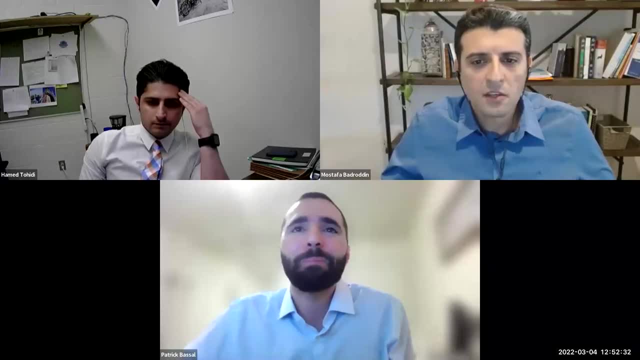 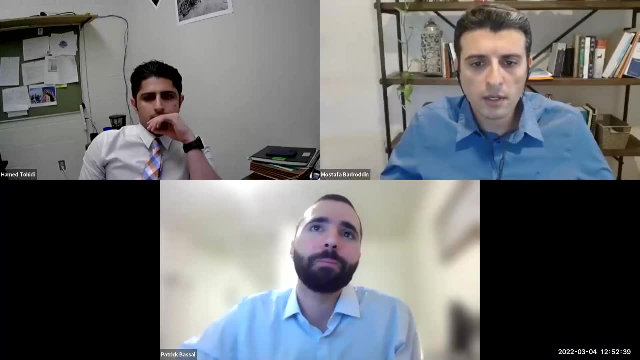 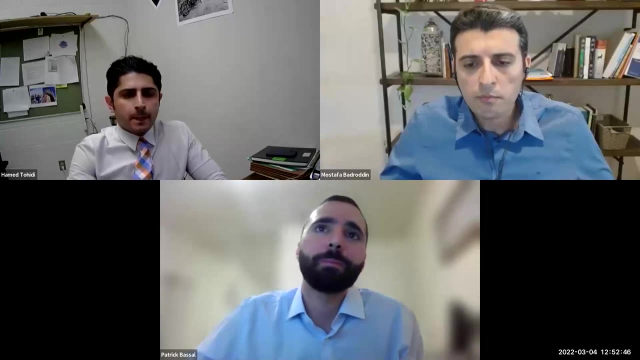 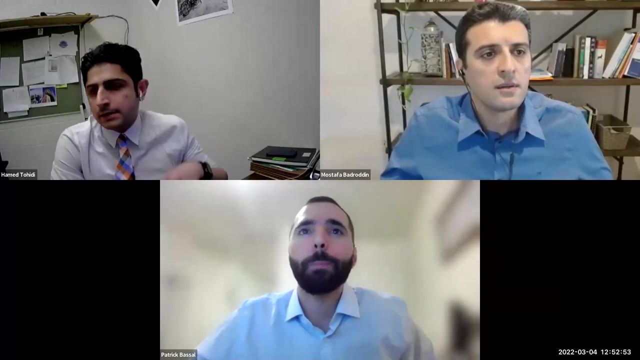 I hope that answers the question. Thank you, Patrick, for clarification. So the next question from John Louie for Hamed About the LPI lowland plot. Can you explain the differences between the severe and moderate to severe curves? Yes, 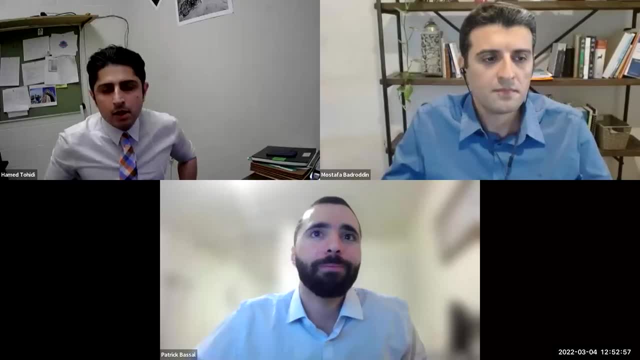 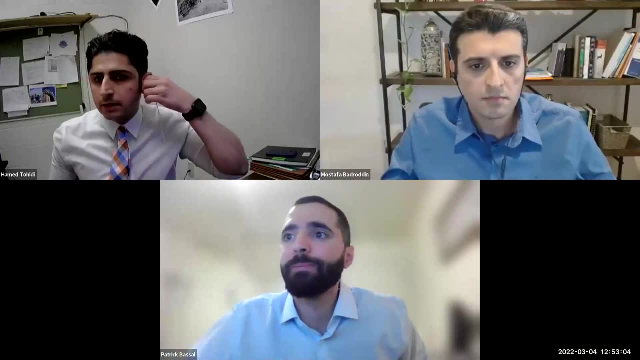 Actually, the method primarily used in this HOD project was the LPI that was developed by Iwasaki. However, it wasn't the only method we used. We're currently doing the numerical analysis, But due to the time limitation, I couldn't present everything. 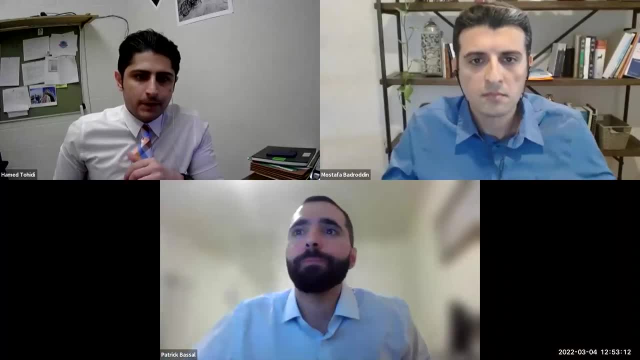 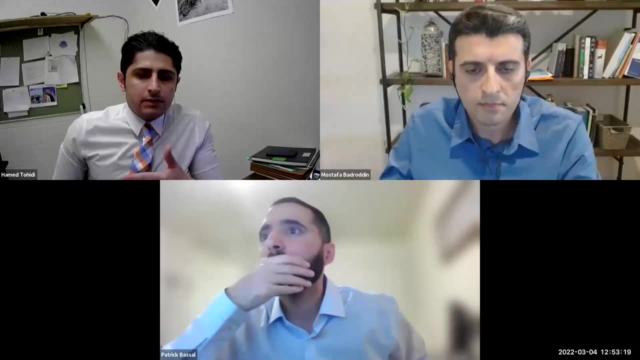 So that LPI had different thresholds. Okay, LPI 0,, 5,, 15.. The probability of liquefaction- moderate to severe- is counted when the LPI is more than 5.. Or in the other words, between 5 to 15.. 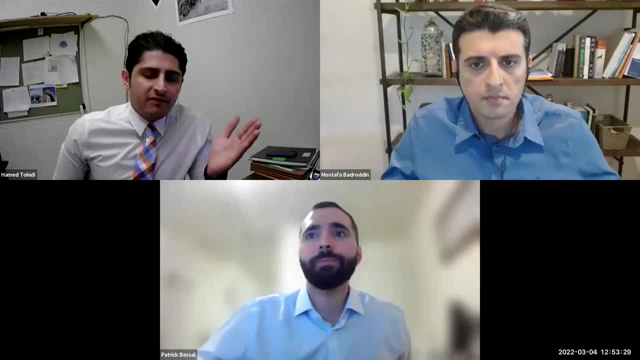 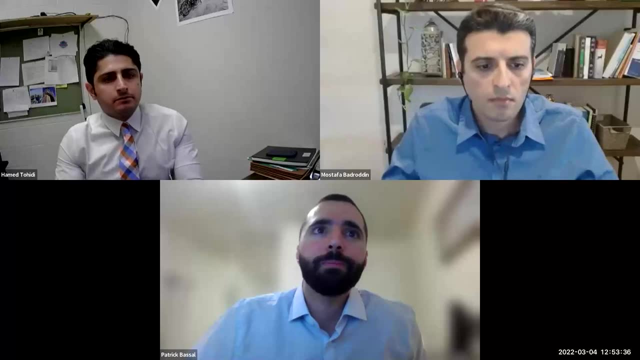 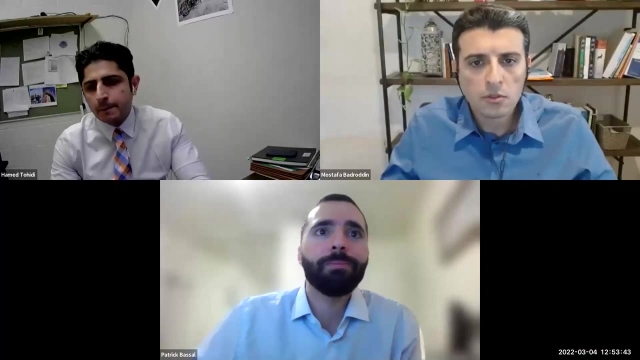 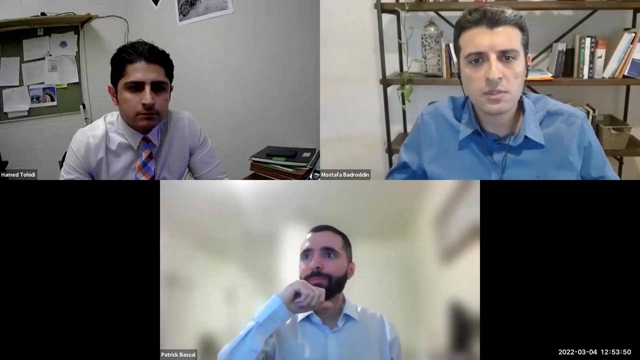 After 15,. if LPI goes above 15,, exceeds 15,, we call it the severe probability of liquefaction. Thank you, So next question for Patrick from Apol Atukorola. So how did you reconcile the lateral extent of a displacement predicted using the different realization with the measured values? 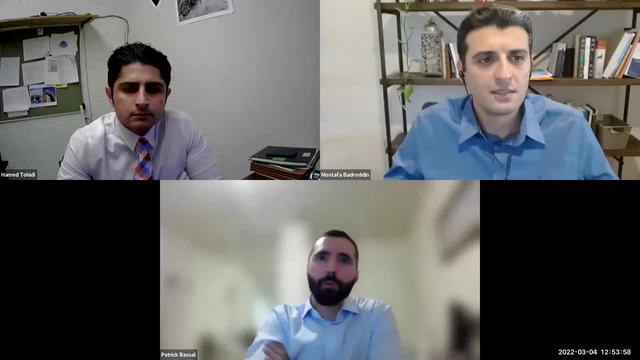 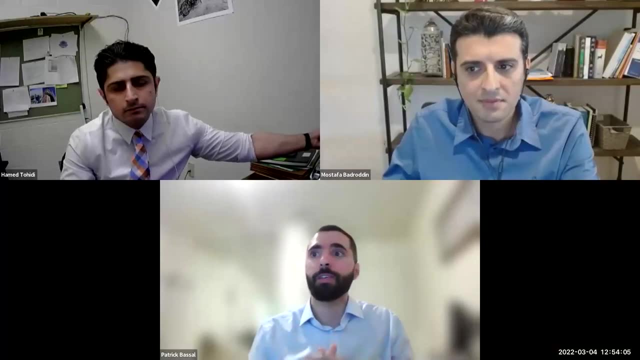 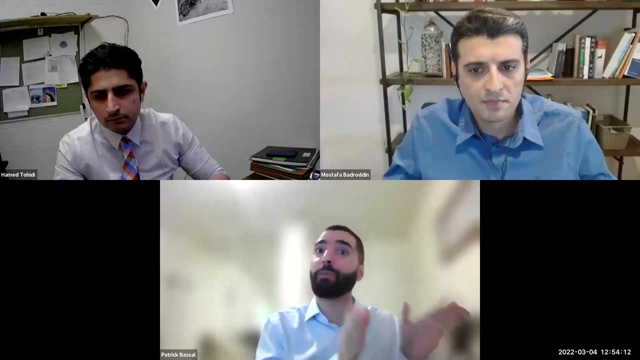 Yeah, it's a good question. So a big part of this work was to really expose what kind of variability you get based on these different realizations, And so we couldn't reconcile every aspect of the deformation. If you notice, we did have greater deformations. 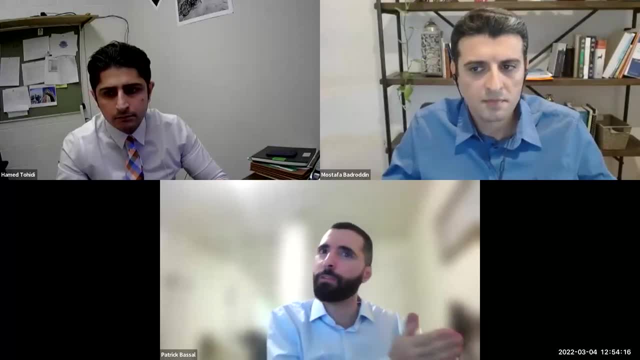 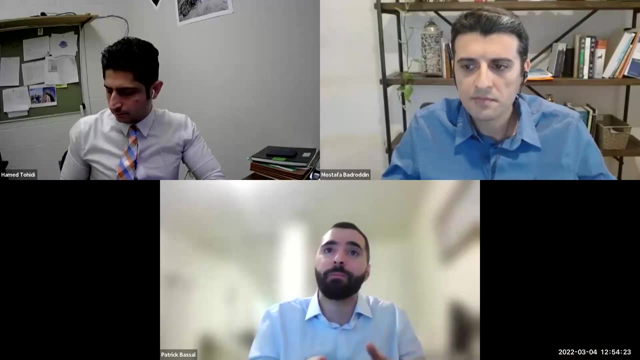 Further from the channel, When you're beyond like 20 meters from the channel, We did have greater displacements than what was measured, Because in the field we had a large crack. that was basically where the measurements ended, And so that could be due to a number of factors. 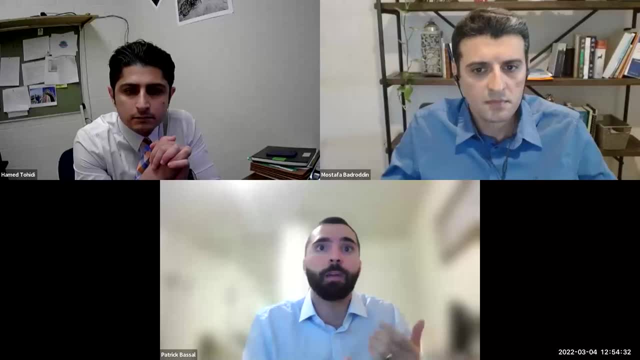 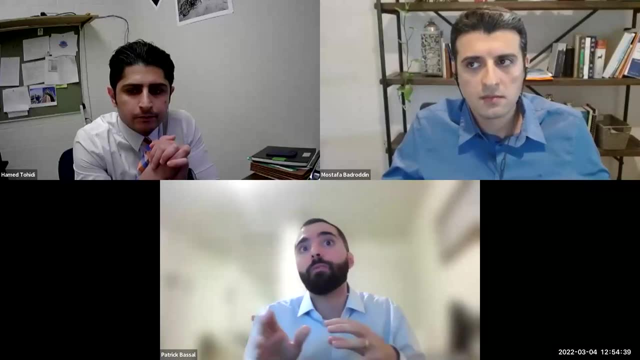 There are limitations in the modeling methods we're using, Because we can't model granular scale details, We can't model cracks directly And we can't- at least in our analysis, we didn't consider 3D effects. that can also play a role. 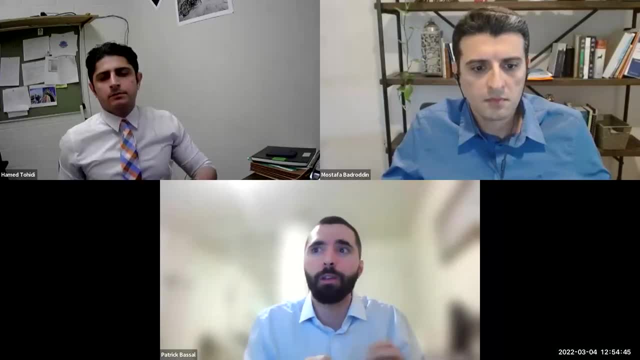 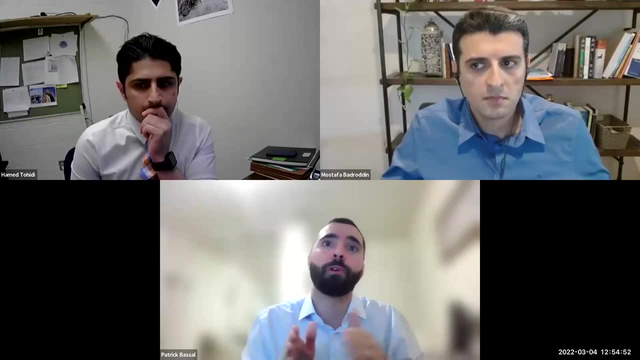 Nearby structures. So there are some details that could influence these results, And so a lot of my work was really kind of pointing to that. Also, the ground motions played a big role as far as how far the lateral spreading extended. So I'd say it was the ground motions and the stratigraphic variability that had a big effect in the end. 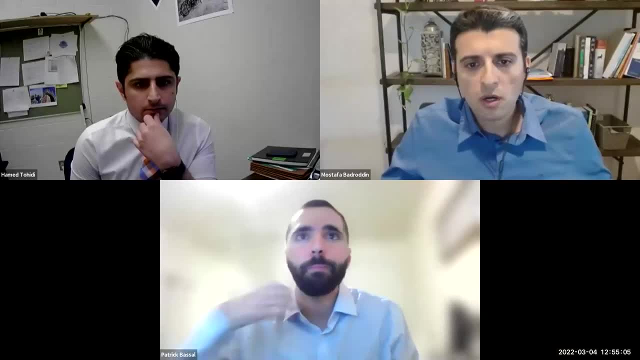 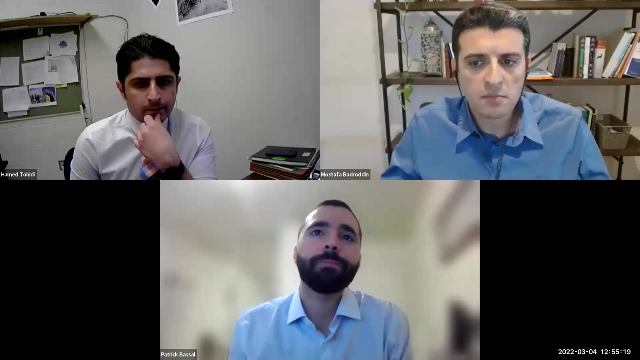 Thank you, Patrick. The next question for Hamed, Another question from John Louie. So any thoughts on what could have made the surface wave Work more efficient or more effective, Like better field equipment, or using passive seismic like refraction micrometer? 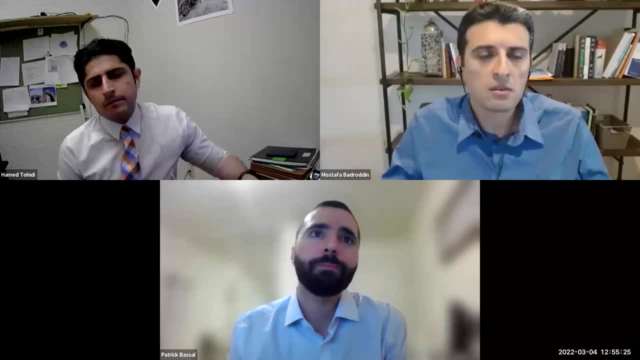 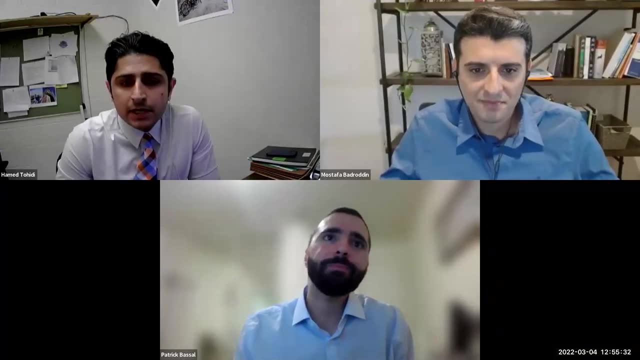 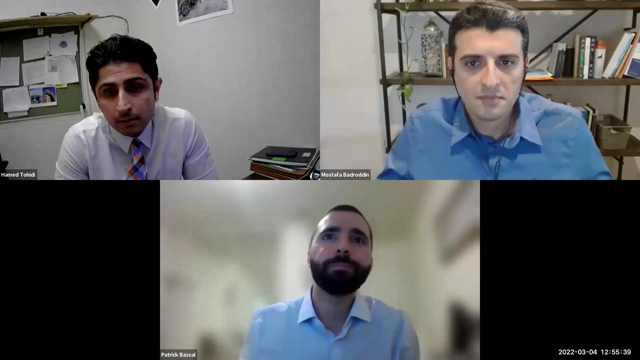 Easier data analysis and shear velocity modeling. Any thoughts on this? Hamed Sure. Actually, we have been using refraction micrometers, REMI and shear wave velocity. We use the shear wave velocity using MASW method. First of all, 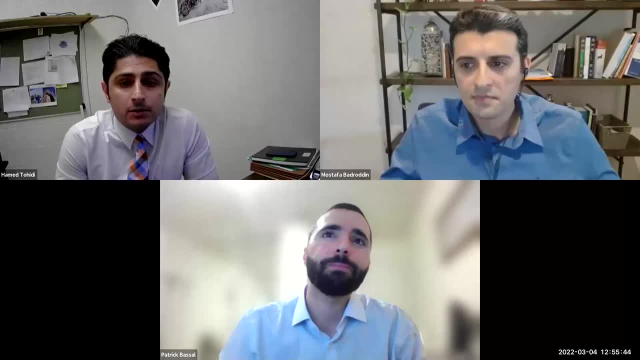 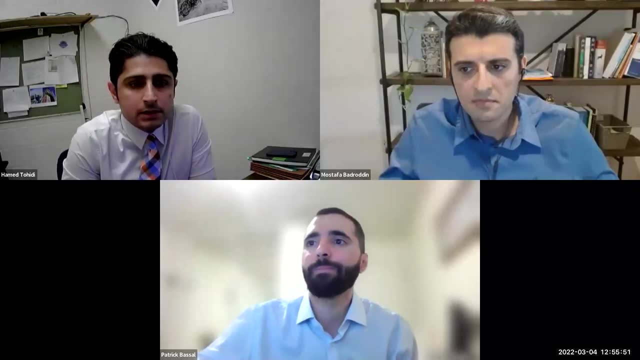 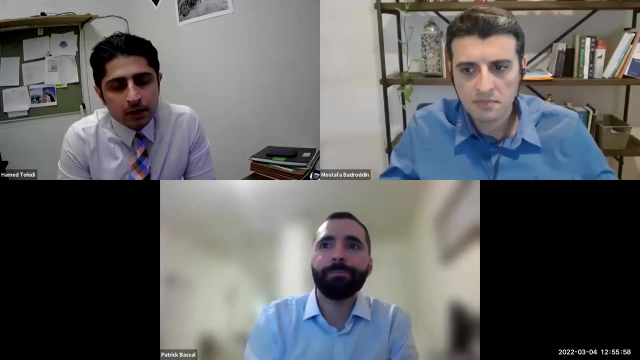 Because we had the equipment. Second of all, The MASW can go very deep. Also, we thought about using the GPR machine, But GPRs cannot go very deep. You know, GPR is good for shear wave velocity analysis of shallow. 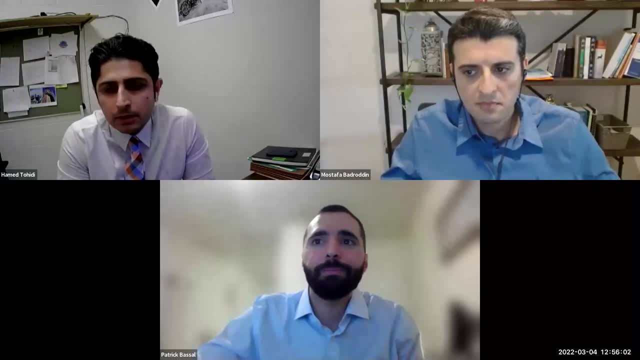 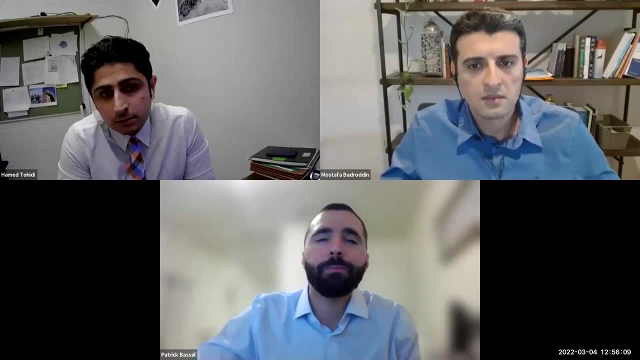 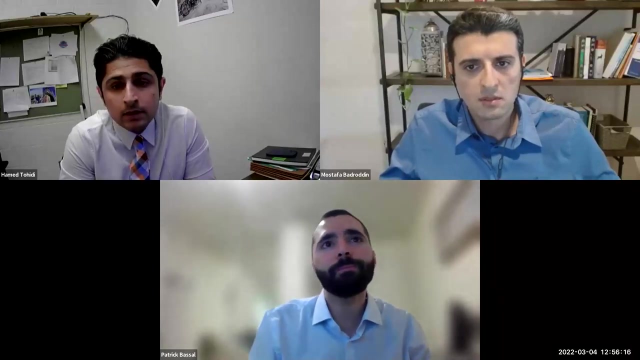 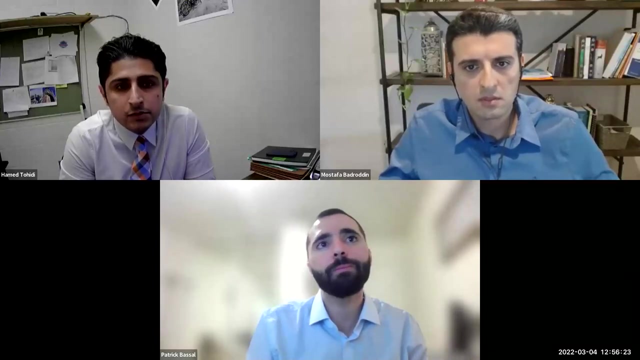 So according to our analysis based on MASW and REMI, so far I think for this project they were the most efficient. Of course We have the other equipment, other techniques to do the shear wave velocity analysis, But first of all to buy everything again from scratch and also to train students to use those new devices and new techniques. 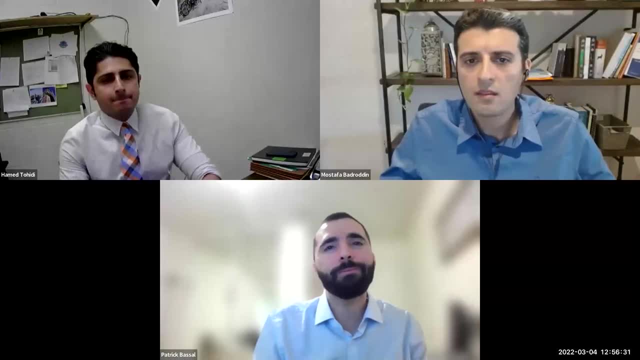 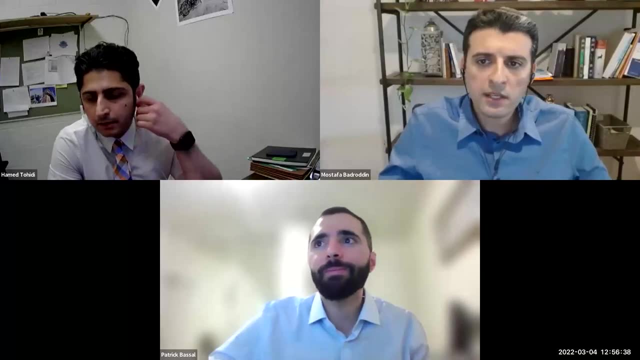 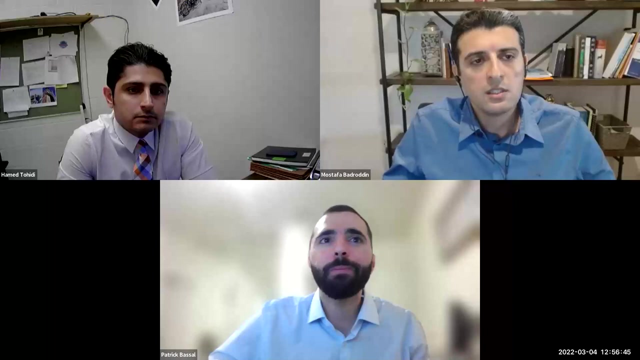 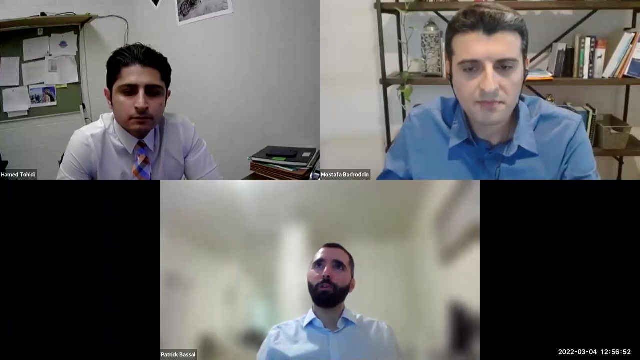 It's kind of costly and time consuming. Thanks, Hamed. So question from Muhammad for Patrick: Can you explain the effect of depth on the CPT, on the probabilistic permutation? Yeah, sure, And so depth is a factor that you might get a trend in your properties with depth as you go deeper, for example, 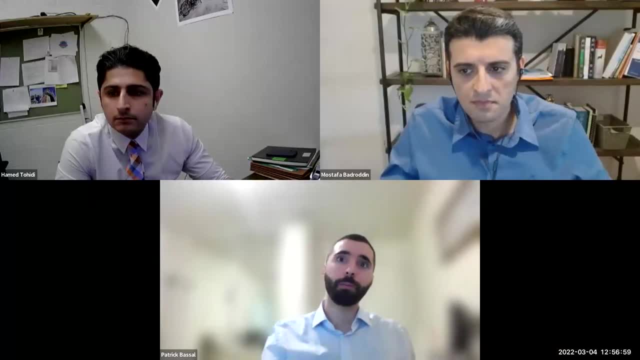 And so we didn't have too much of a trend when it came to our play data. We are using a normalized value. It's normalized by our effective stress, And so we really didn't see much of a trend at all going with depth. 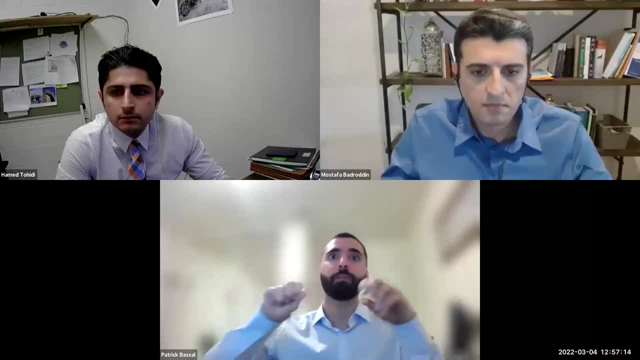 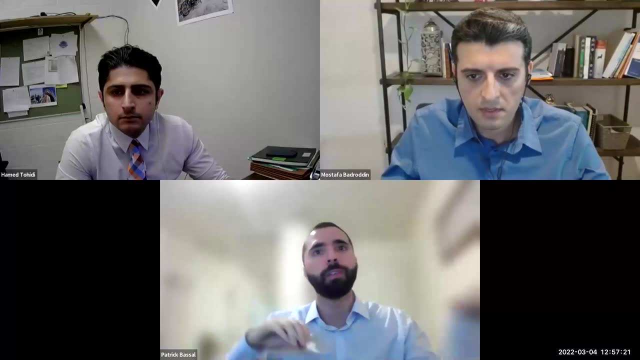 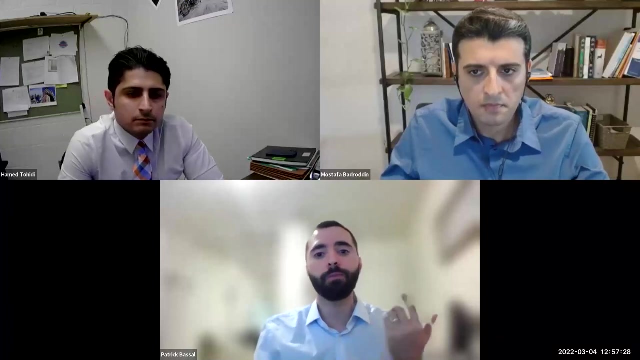 There were some trends more laterally. So we did account for different CPTs and how different layers that soft plane or the channel with different material further. So we did account for that by just modeling those units differently. So that was for the clay. 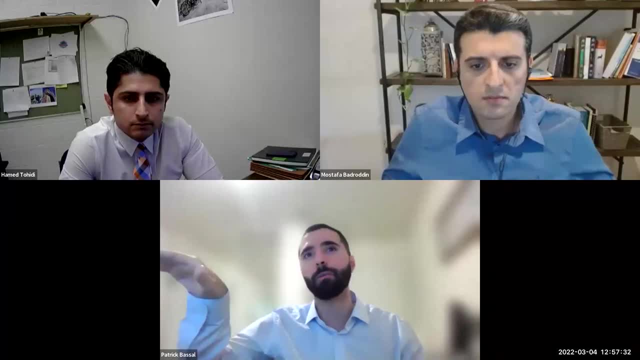 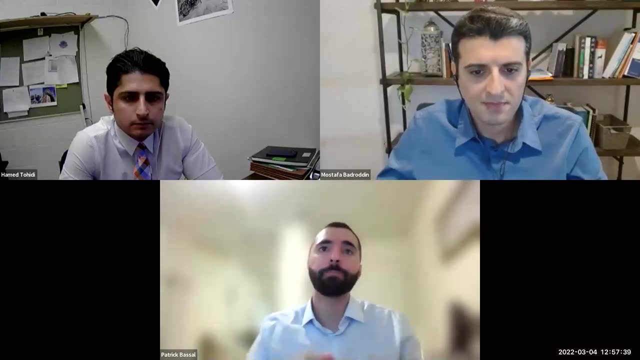 For the sand there was sort of like an intersection where we just kind of modeled two different units differently: above five meters We had lower strengths, And below five meters we had higher. So we did that pretty roughly for this model. Within geosynthetics there are ways to include a trend in your modeling. 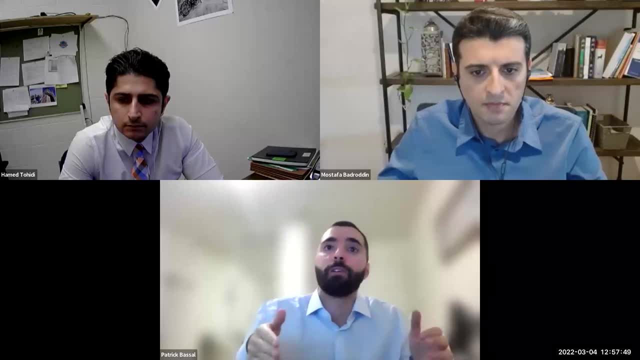 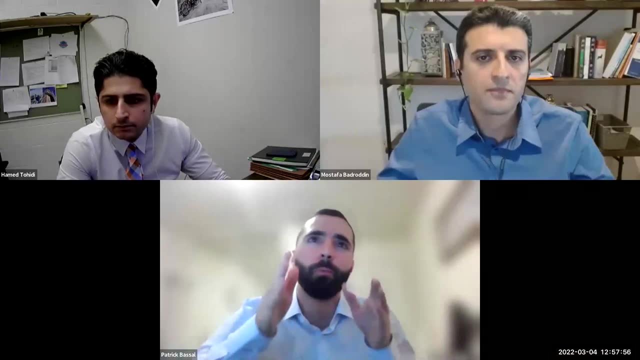 So you could, you know, if you don't have an overall trend in your analysis, you could use that average trend ultimately for your subsurface modeling. But in this case it was more rough based on, you know, based on the overall trends that we saw. 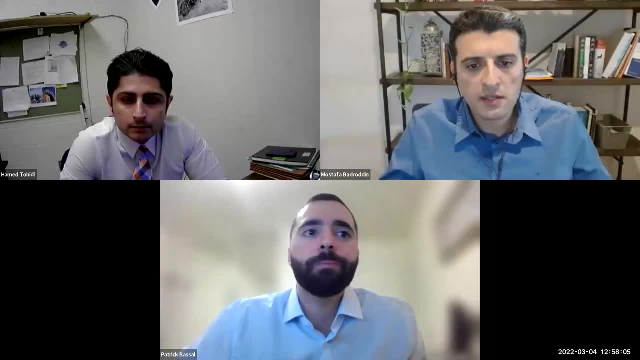 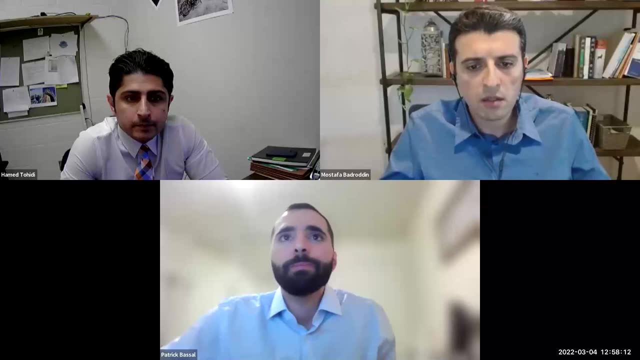 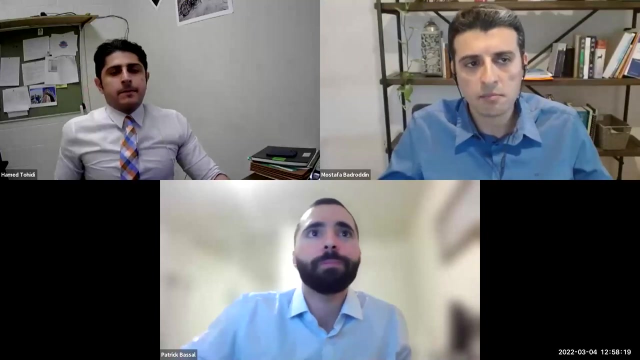 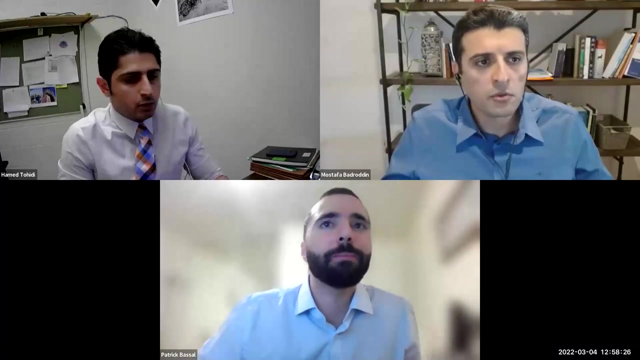 Thank you, Patrick. So next question from Jason Pinsa to Hamed: Have you accounted for seasonal variation of groundwater level throughout the hydrological year? If yes, how do you incorporate them in your liquefaction hazard maps? Hamed, would you please unmute yourself. 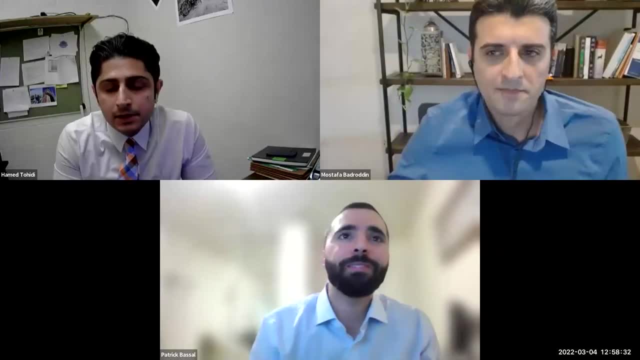 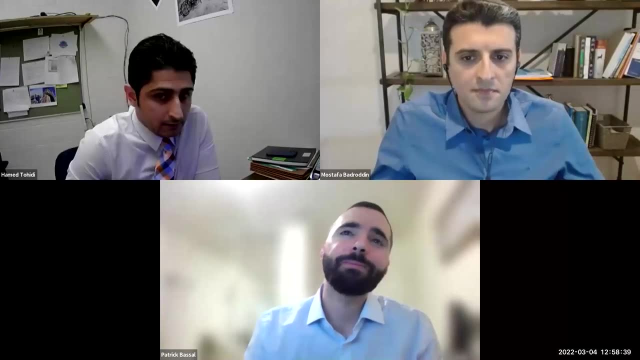 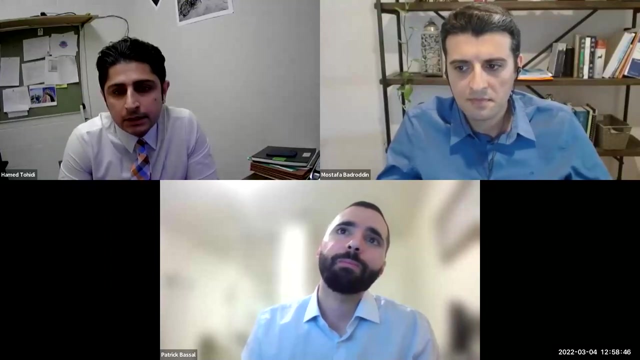 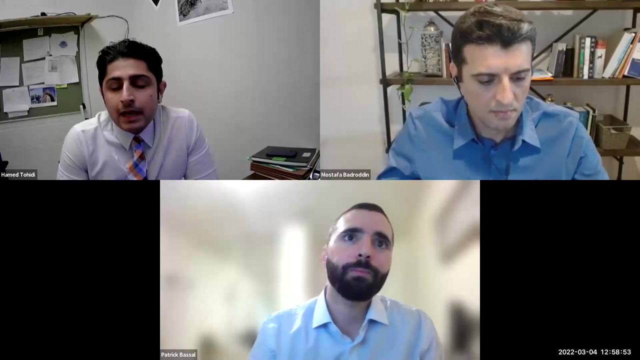 Sorry. Yes, we have considered the impact of. Yes, We have considered the impact of Variation, seasonal variation of groundwater level. That's how we did it. Okay, We obtained the groundwater level to record the data from different seasons. This is the most wet season and the most dry season. 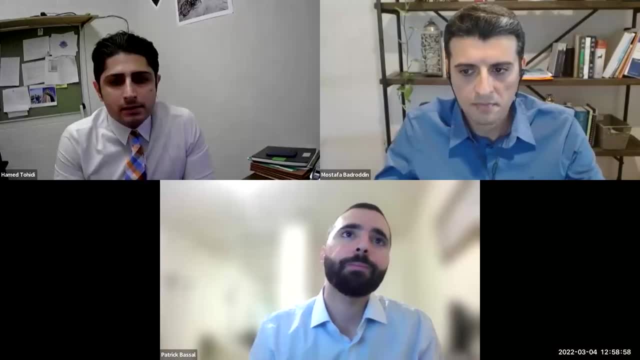 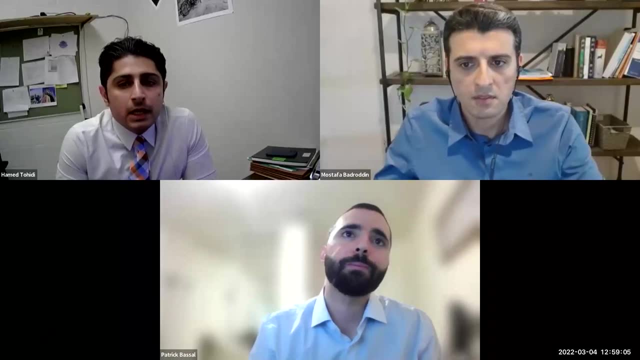 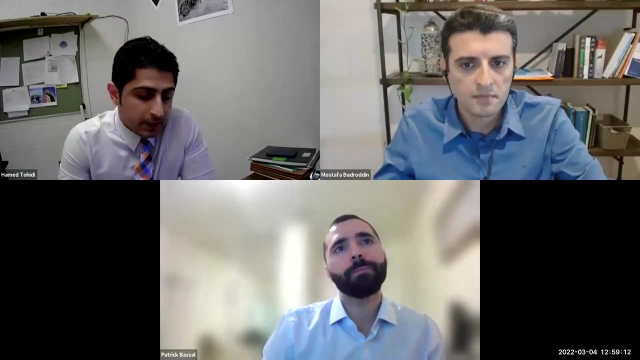 And different wells we have been. we have installed different wells okay to record the groundwater level in wet and dry season for each well and for each season. we have had too many recorded data for each wealth okay, and also sometimes due to the situation, for example, we couldn't have those wells. 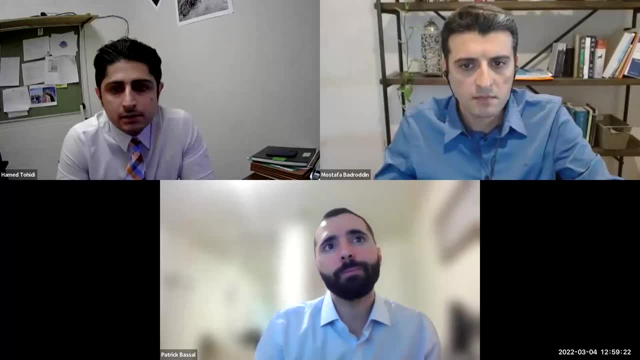 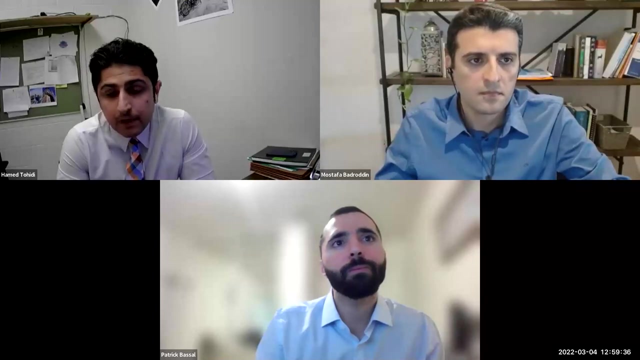 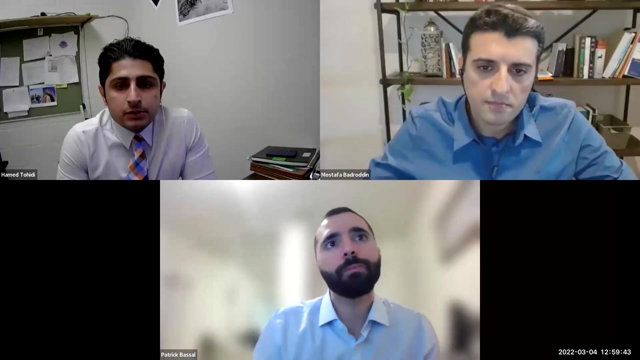 installed and also record the data. we asked the usgs and they were very collaborative to us. we got the average of groundwater level of the wet and dry season recorded data to do the liquefaction analysis. however, of course this is not you know the best way, but to kind of preventing the underestimation and 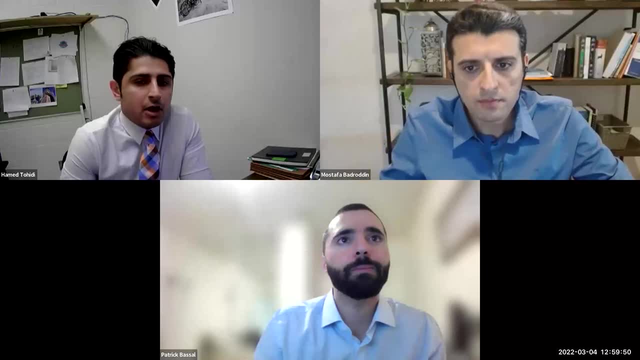 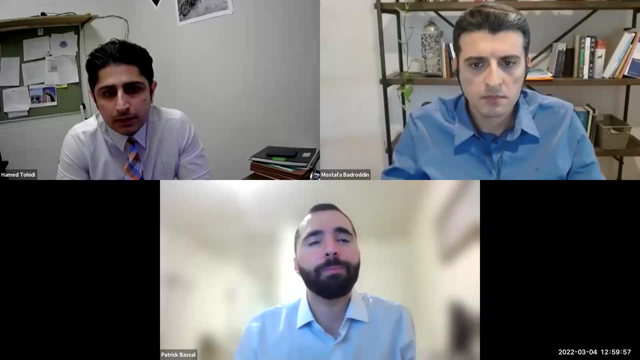 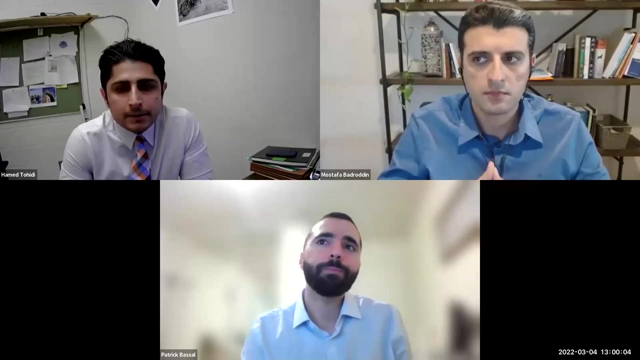 overestimation of liquefaction analysis. if we use the dry season groundwater level data, so of course the water was deep and the probability of liquefaction low. if we use the wet season, the water was shallow and, uh, probability of liquefaction was go high. so by 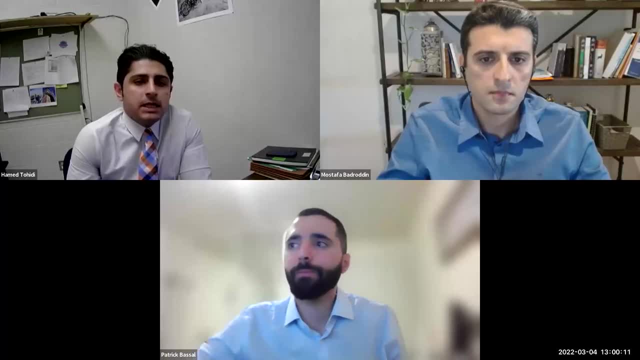 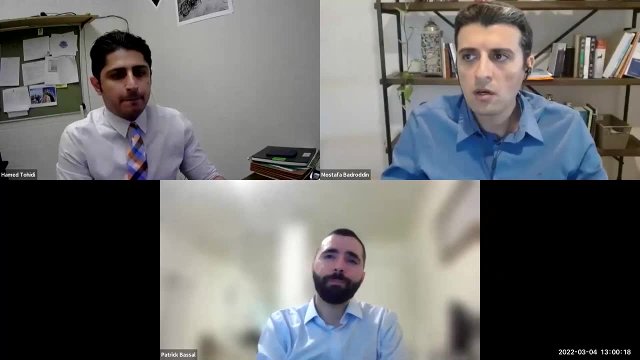 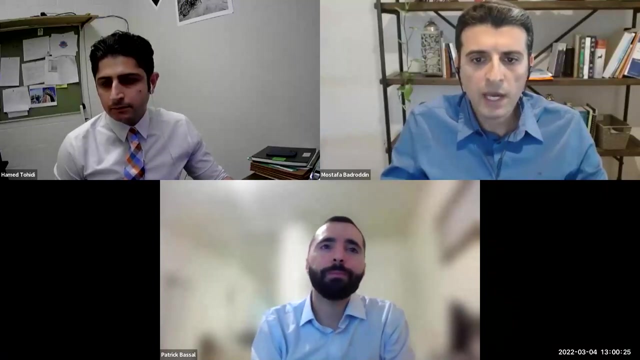 having the average, we tried to kind of minimize the amount of under and over estimation. thanks, hamid. so, uh, we know it's almost 1 pm, so this is this would be the last question. uh, we had a question from francisco franco. uh, to patrick, i found that. 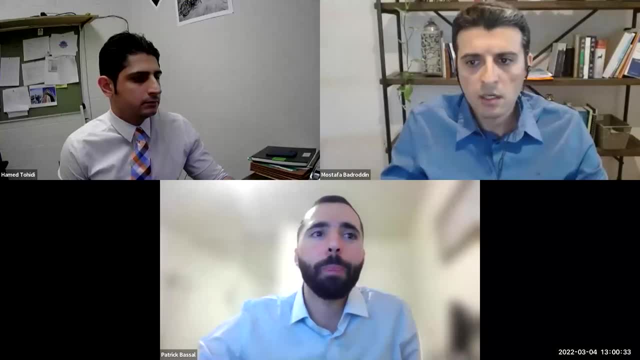 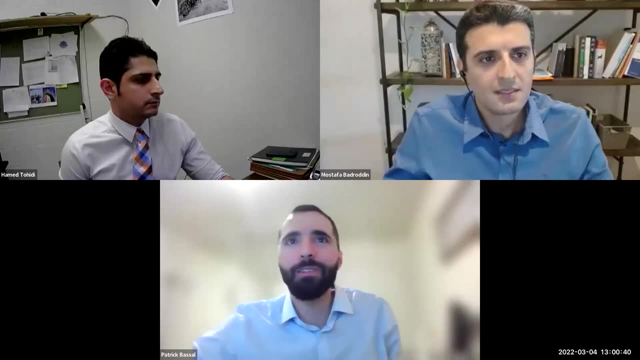 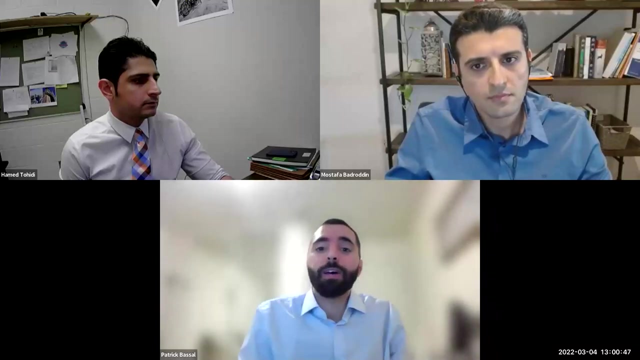 tprog you use very interesting. could you comment a little more about what it consists of, please? yeah, so tprogs, that's actually um. it's a geostatistical method. that's um. it was actually developed at uc davis, where i go to school, um, and and so it's really a program that. 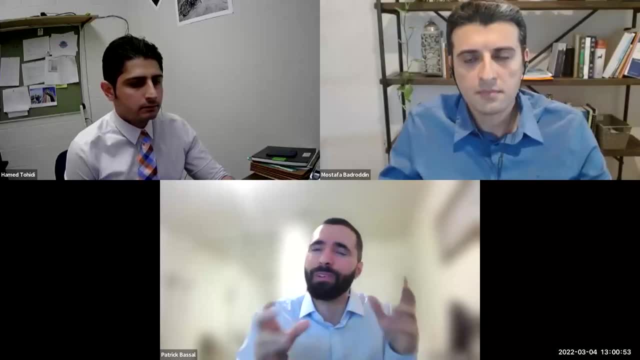 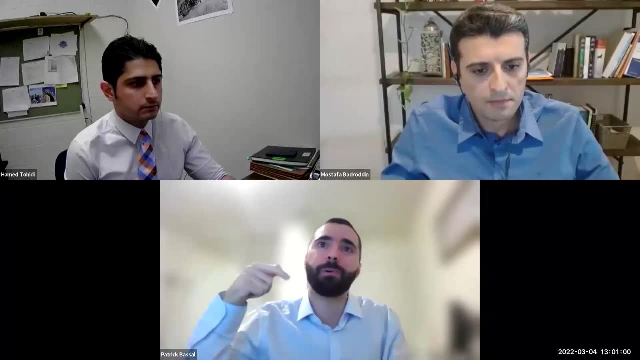 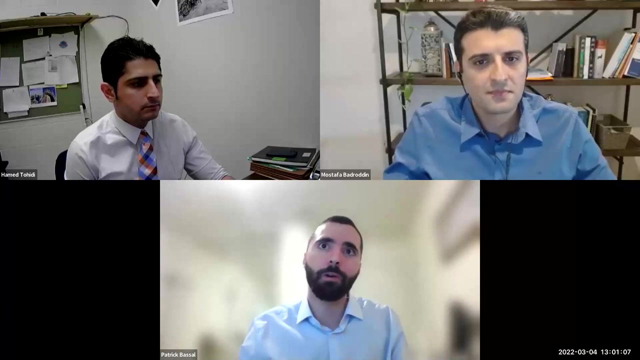 accounts for, um, basically your categorical variability. so you can, you can account for categories and create geostatistical models based on it, and so that transition probability example that i showed, um, that was just an example of, you know, the transition probability modeling scheme that tprogs uses, and so tprogs really, um, you know, based on the variability you have, um, or, sorry, the. 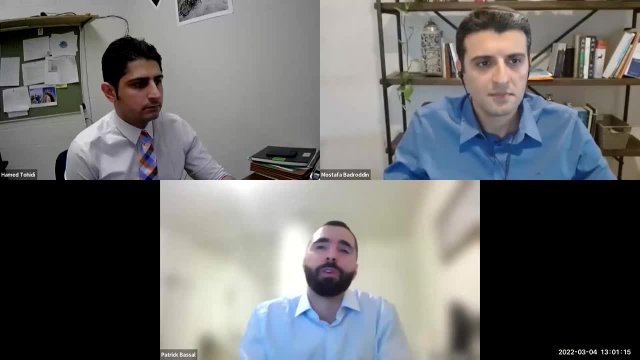 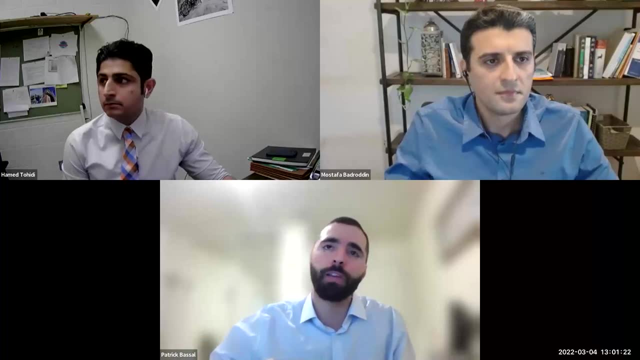 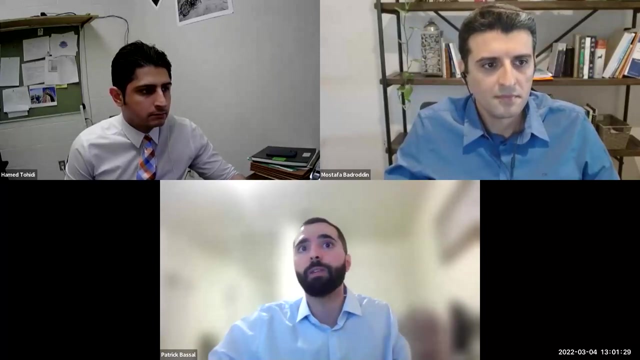 transition probabilities that you have from going from one unit to a different unit. you can build models for every possible combination. essentially, you build these markov chain models, you get that variation and then um, then it uses a, um like an indicator simulation approach to really um, really kind of get that um, the simulation in the end, you know, using that information you have.